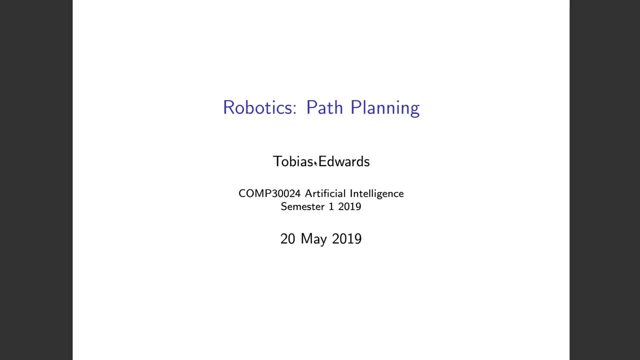 All right, Hi guys, For those of you who haven't met me, I'm Tobias. I'm one of the tutors for artificial intelligence this semester And I'm just going to be given a brief webinar mini lecture, kind of Python demo, just going over a cool algorithm that I've been looking into about path planning in robotics. 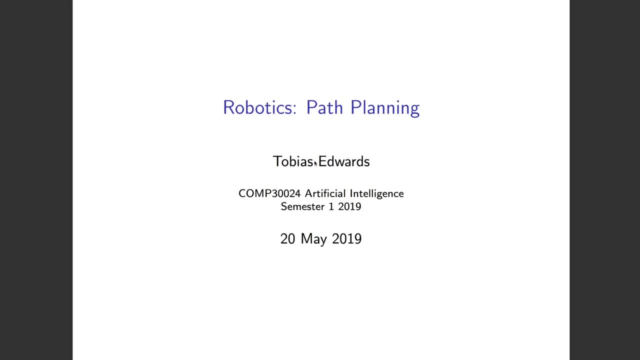 And this week we're going to be talking about robotics in class, talking about some of the issues there and how that relates to artificial intelligence, And we're going to hopefully be doing a little bit of a deep dive into just one particular aspect of that. 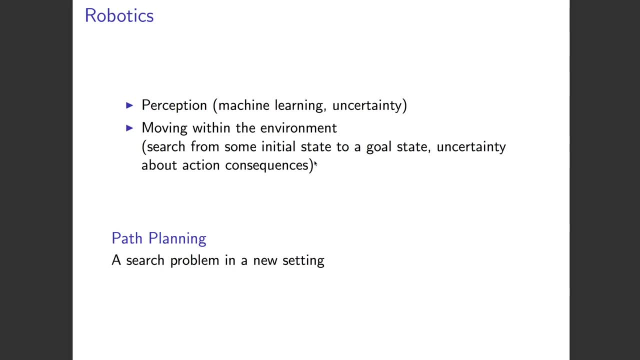 So what are some of the things in robotics that are related to the artificial intelligence course we're doing at the moment? Well, one big thing is perception, So it's all well and good. It's a robot that's able to act in an environment. 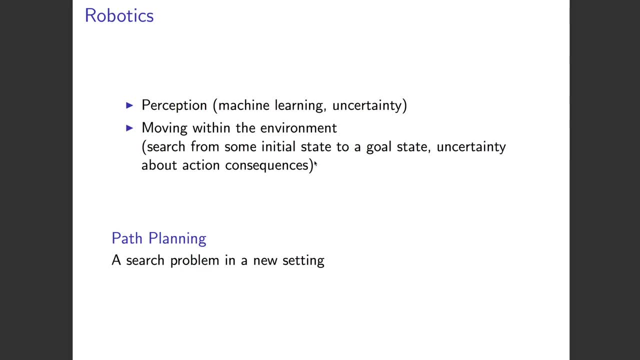 But if it's unable to understand its environment then it's not going to do a great job. So some of the things we've spoken about this semester that relates to that are machine learning, maybe some computer vision stuff. If you're able to capture an image of your environment, actually being able to understand that as a human would is quite a complex task. 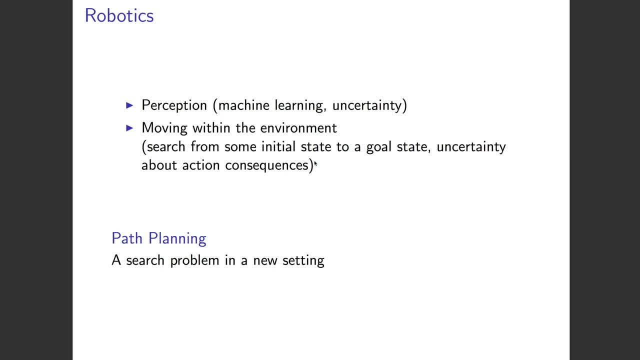 And the other thing is maybe what we perceive if our environment isn't fully observable, if it's only partially observable, then what we perceive might not be all of the relevant information to the state or all the relevant information for the environment around us. So there's going to be some uncertainty there. 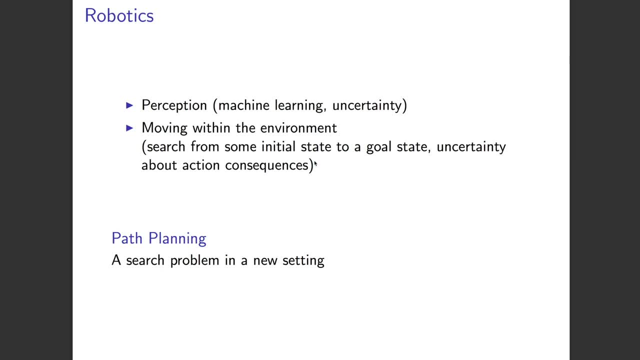 So some of the probability methods we've been talking about this semester would come into play there. Another thing is moving within an environment or just acting in general within the environment. We would usually model these robots as agents in the way we've been talking about in this semester. 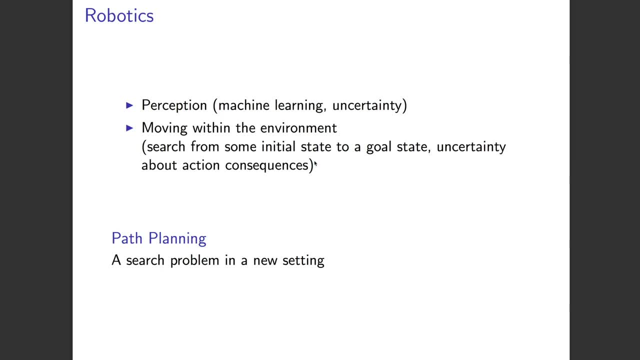 And then you get these search problems or planning problems like we were talking about. You've got some initial state of a robot and you want to get to some goal state- Some of the other things that might come into. that is maybe when you perform some action. 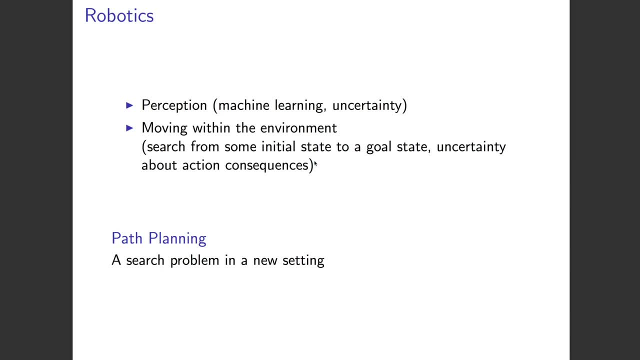 you're not 100% sure about what the result of the world or the robot state is going to be after that action. So maybe it's not a deterministic environment. Today we're going to be talking about path planning specifically, which is just a search problem, as we've been talking about in this semester. 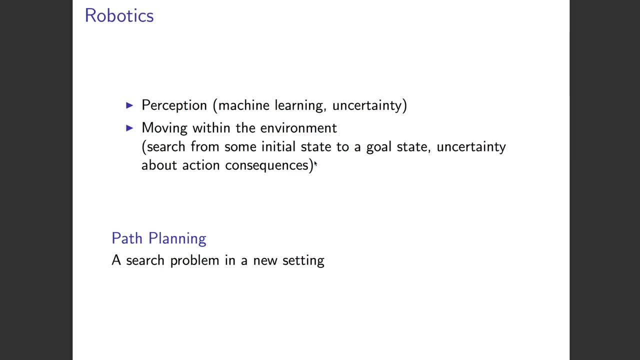 But it's a little bit of a new setting and some new challenges that come with that. But really we started in some initial state. We've got some finite or infinite set of actions that we could be taking at each step And we want to choose the sequence of actions that we can take to get from our initial state to a goal state. 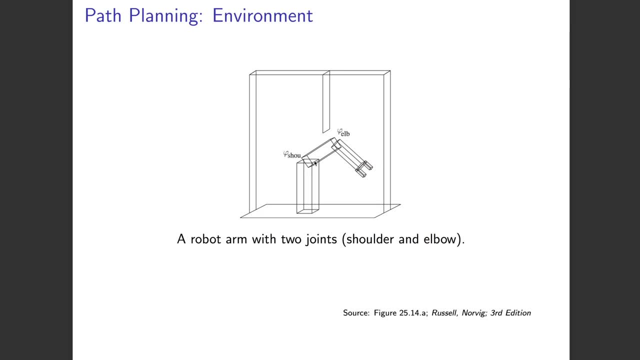 So just a bit of a toy example that we're going to be talking about here is this scenario where we've got some robotic arm and we've got some robotic hand And we're able to manipulate two joints within this robot: the shoulder and the elbow. 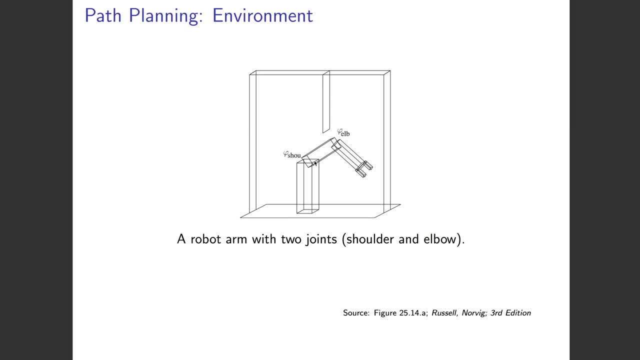 And using those two joints, we're going to be able to manipulate the position of the hand. So one example where this might come up is perhaps we're packing boxes in a warehouse and we're wanting to pick up one box and move it somewhere else. 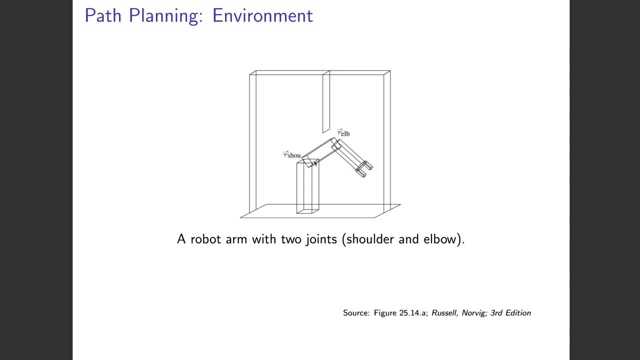 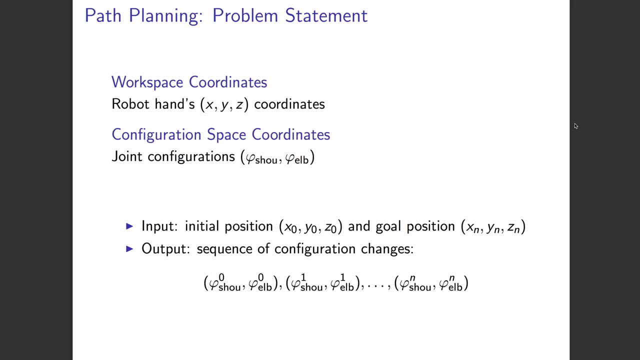 So it's important for us to be able to understand how to go through the sequence of actions with these two joints which we are able to control, to get from our initial state to some goal. So some of the issues that we have here are our understanding of the problem. 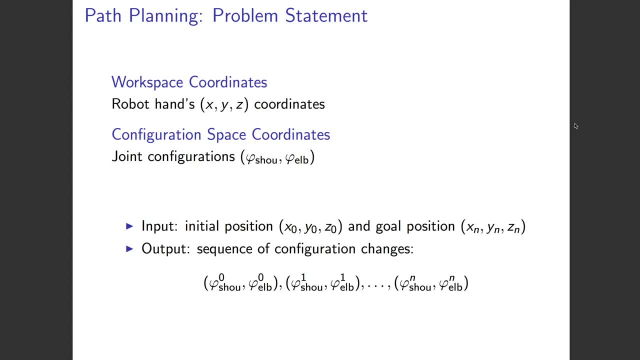 where the robot's hand is. So we have an XYZ coordinate, some position in space, right? So it starts off somewhere in space and we want to get to somewhere else in space. So perhaps the initial position is when we've picked up the box. 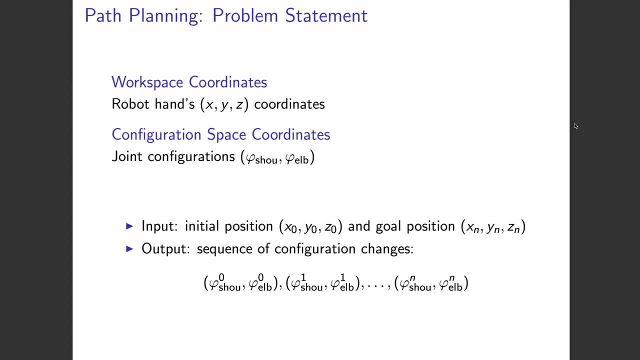 and the goal position is some conveyor belt that we want to place the box into or some pallet that's being packed. So we refer to this as the workspace coordinates in this setting, But the way we're actually going to be reasoning about the actions we carry out. 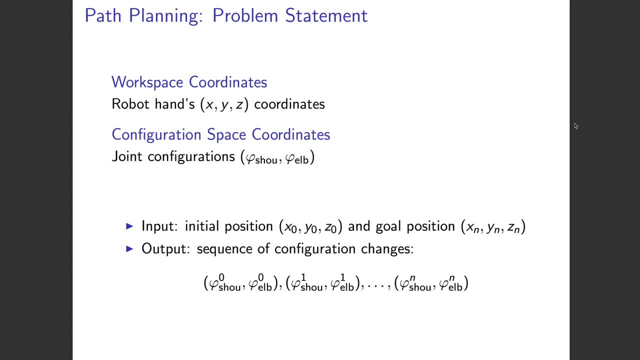 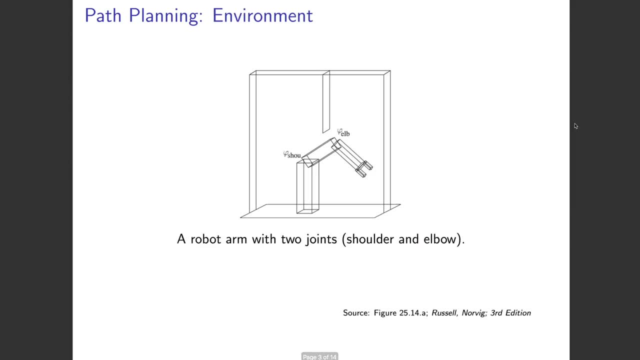 and the control we actually have over the robot is by converting these configuration space coordinates. We don't actually have direct control over the XYZ coordinates. We've only got direct control over those two joints we were talking about before, the shoulder and the elbow. 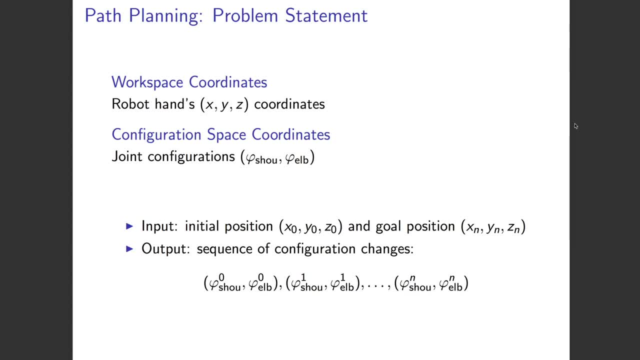 So one of the things we're going to have to answer is how do we convert between these coordinate systems? But in general, the problem statement is we're given some initial position in the real world and we're given some goal position in the real world workspace coordinate. 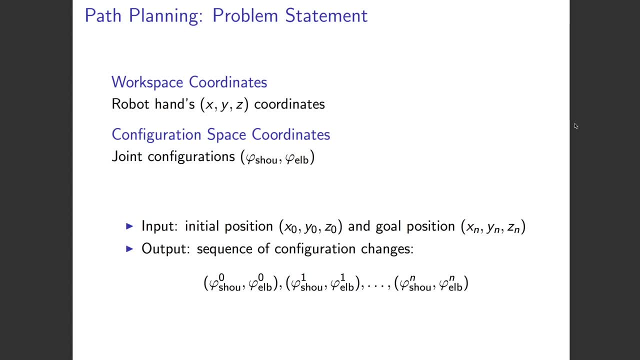 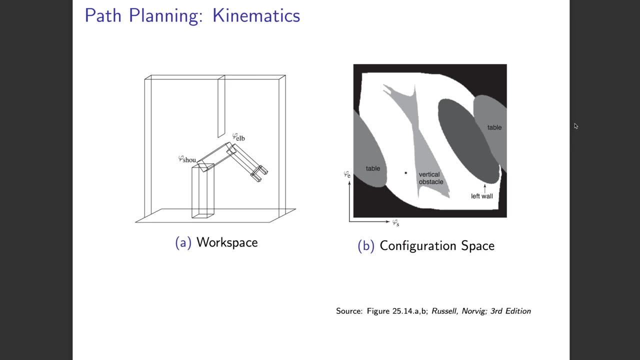 But what we actually want to find is a sequence of configuration changes or a sequence of actions we can take that moves the states of the joints that we can control from our initial state to some state which matches the goal position. So, on the left, here we've got the image I showed you before with the two joints. 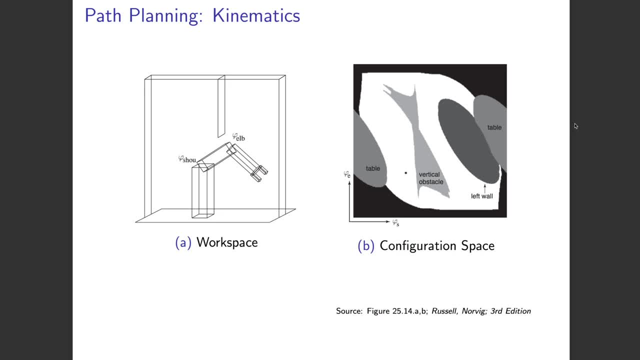 and where the hand is is its workspace coordinate. So the robot hand's position in space is that XYZ we were speaking about. But on the right we've mapped that three-dimensional space coordinate into this two-dimensional space, the configuration space. 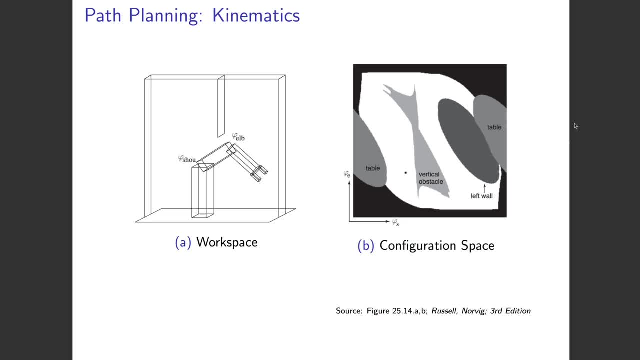 So the axes here are the angles of the shoulder and the elbow joints, And we've got white space for what we'll call free space, which is positions where the robot will configurations that this robot could take on. And then we've got these dark regions which correspond to obstacles. 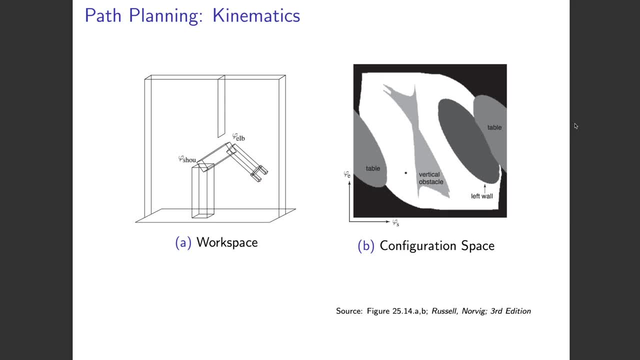 So obviously the arm can't fold in on itself. So that's the black region on the outside. It can't hit the table that it's on. So they're those two ovals labeled tables. And then there's also this vertical wall. 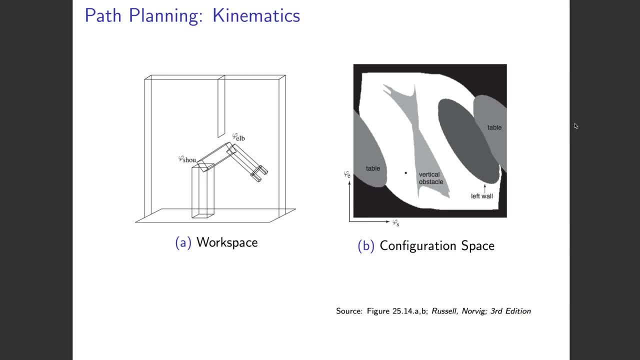 So there's a few constraints to how we can move and this configuration space diagram with the free space and the occupied space kind of encodes that. So the problem of transitioning from workspace to configuration space coordinates and vice versa is called kinematics and robotics. 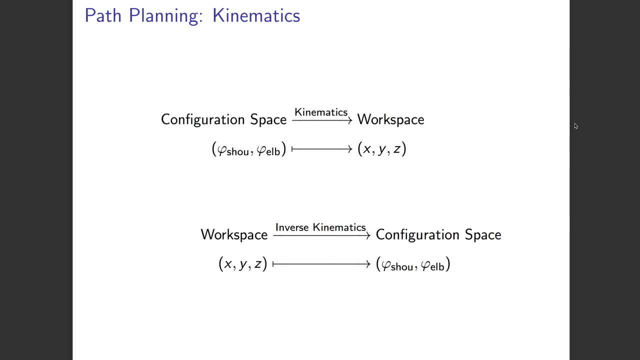 So we say that we're doing kinematics, if we're determining what the workspace coordinates are, given the configuration. And then what a more trickier problem is the inverse kinematics problem, which is taking a position in space and giving which configuration will actually give the hand, that position in space. 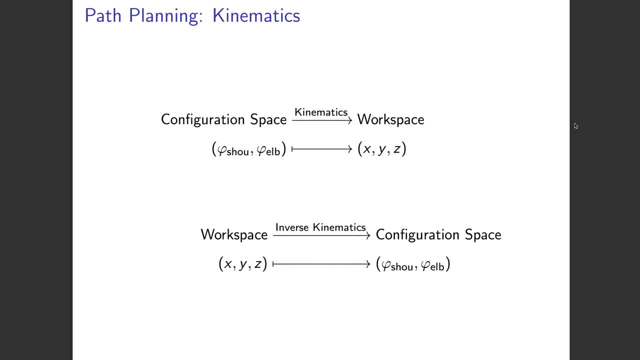 Depending on how many degrees of freedom our robot has. there can be no solutions, two solutions, infinitely many solutions to this problem. in which case it's a problem of not necessarily which configuration will get us this, but what's the best configuration to get this. 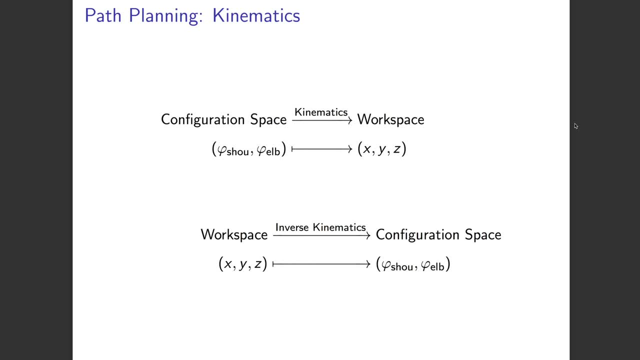 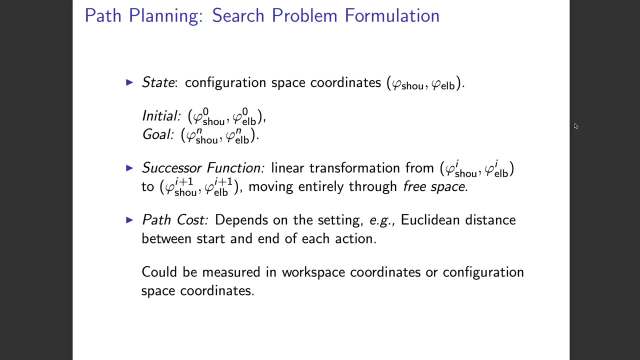 There's lots of different ways to get from an initial position to a goal state in this kind of real-world robotic setting, but some of them could be ridiculous, So we want the most sensible configuration to get to that goal. One of the things we've been doing this semester is formulating: 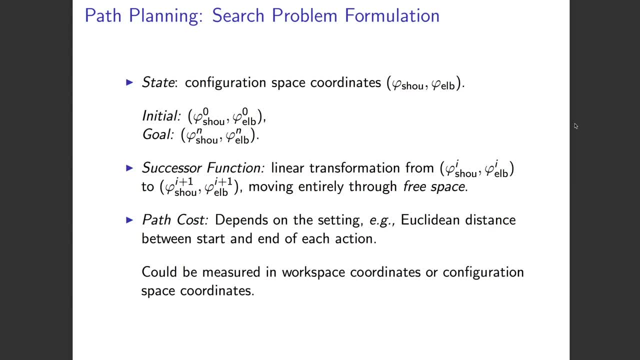 the problems we're given as a search problem And the questions we have to answer here are: what does the state encode? What information is relevant to the state of the problem, The successive function which gives us which actions we can take when we're in one state. what are the successive states that we can get to? 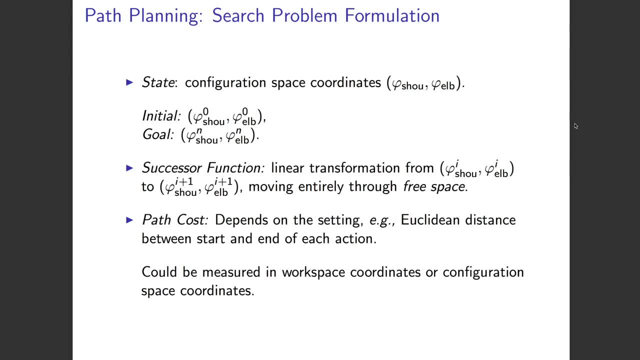 And then how expensive is each of these actions? What's the path cost here? And all of these things give rise to kind of a search tree, as we've seen before. So just going over these quickly, our state is just going to be the configuration space coordinates. 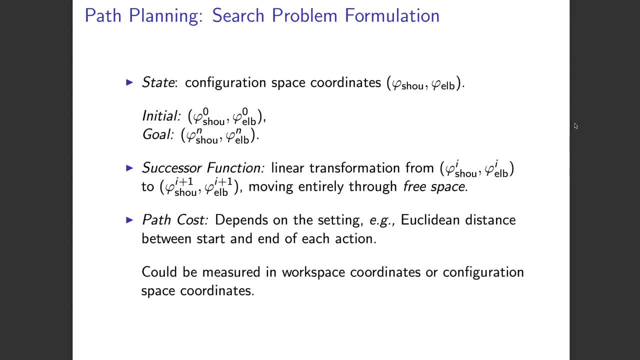 we've been talking about the angles of those joints. We've got some initial configuration and we've got some goal configuration. We're assuming here that we've already done the kinematics or the inverse kinematics, so we're just dealing with configuration. space coordinates. 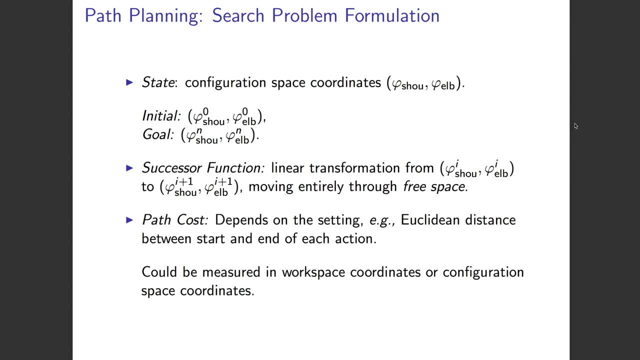 The successive function. well, this is how our robot can move, So we're going to assume that we're able to kind of change the angle of each of these joints at different constant speeds so that we're not hitting any obstacles. So it's a linear transformation from some configuration to another one. 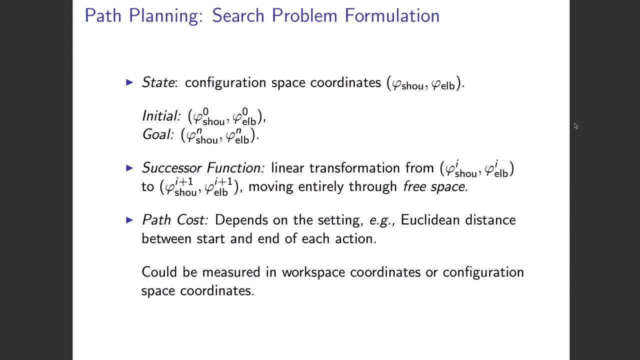 so that'll correspond to a straight line in our configuration space, as long as that straight line doesn't go through any obstacles. So we say it's moving entirely through the free space, And then the path cost. well, that really depends on the setting. 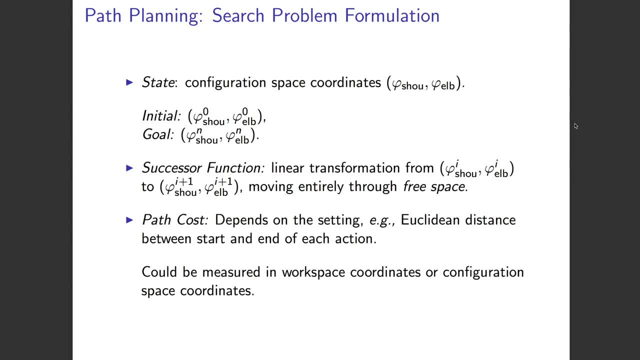 Perhaps it's Euclidean distance, Perhaps it's how long that line is, Perhaps it's how steep the line through configuration space is. It might be more expensive to move one joint in terms of electricity or power than another, And is our goal to do the least amount of work. 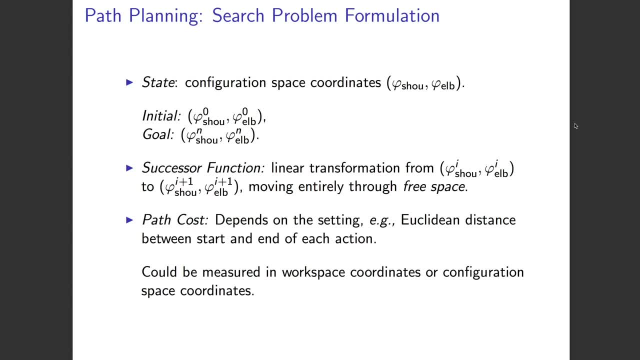 in terms of moving these angles, or is it to move the least amount of space in the workspace coordinates? So it really depends on the setting. I think here probably the most sensible thing is the Euclidean distance between the configuration states And I think, given our simple setting, 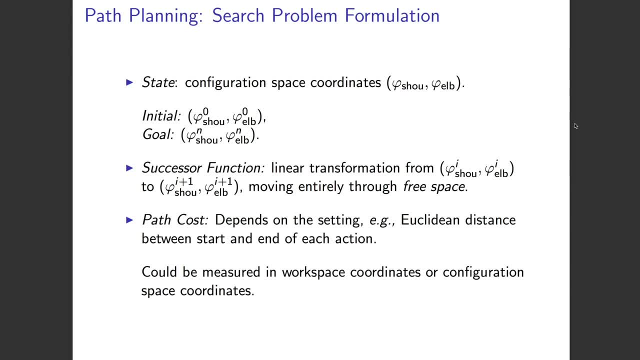 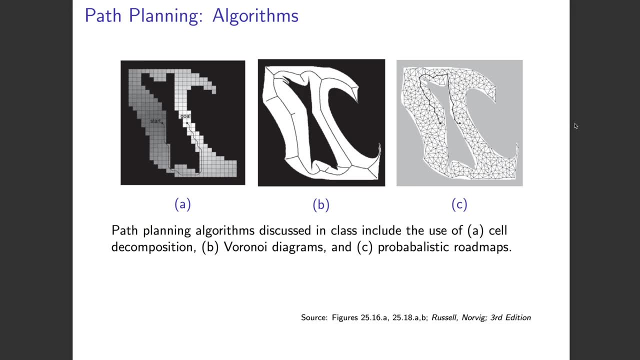 this will probably correspond quite well to a shortest path in the workspace coordinates. So there are a number of ways we discuss in this course to solve this problem. So these three diagrams kind of depict that configuration space, with the free space and the occupied space as before. 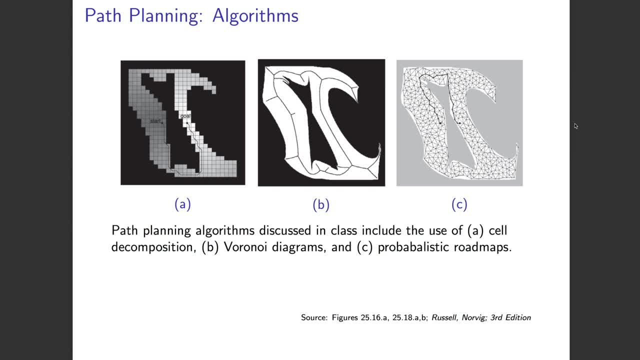 And we're kind of interpreting this in different ways. So the first way is we just split it up into kind of pixels. So the idea is that we're breaking it up into squares which are either entirely in free space or constrained in some way, like there's an obstacle there. 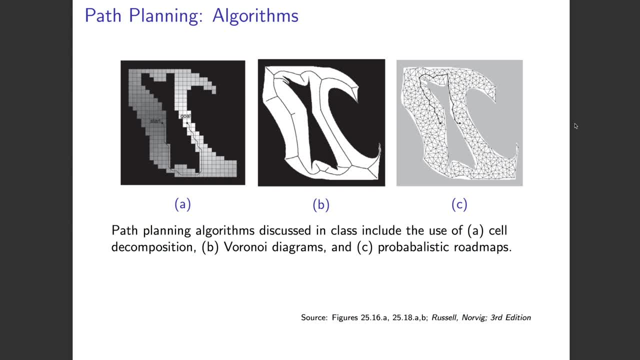 And then we can just treat it as a regular search problem. where we've got each square can get to all the names neighboring squares, And then we just run some maybe a star or breadth-first search algorithm to get from our start state to the goal state. 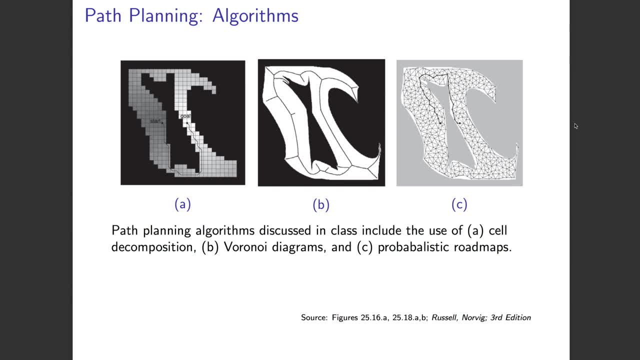 One of the issues we can see there is: it's quite hoppy like quite jumpy. You can see this spot between just leading up to the goal. You can see that you could just take some straight line, which would be a lot nicer. 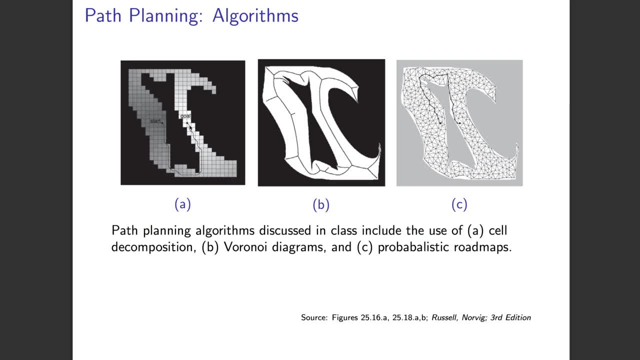 but instead it has to do this zigzag path, So maybe that's one of the issues with this method there. The second diagram is called a Voronoi diagram, And the idea here is that we've got some line and the points on that line are equidistant. 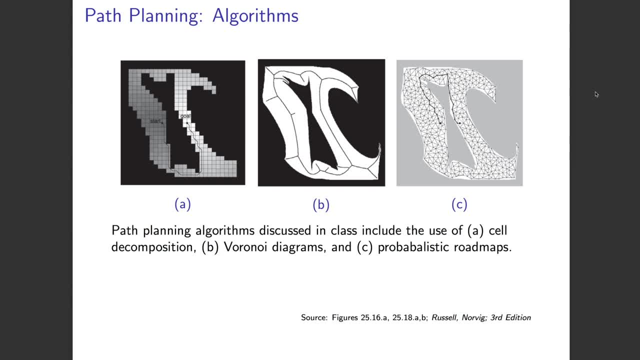 from two or more obstacles. So the idea is, this is kind of as far away from the obstacles as we can get. Maybe we place vertices on the corners of this line and that's how we can turn this into a search problem. One of the things here is obviously: 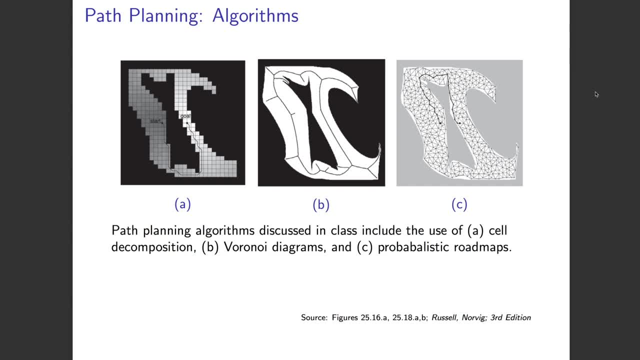 this doesn't necessarily fit with our linear transformations, as we were talking before. So maybe that's fine in this setting, or maybe we'll have to alter this algorithm to use only linear transformations. And this final one is a probabilistic roadmap which is getting a little bit closer to the algorithm. 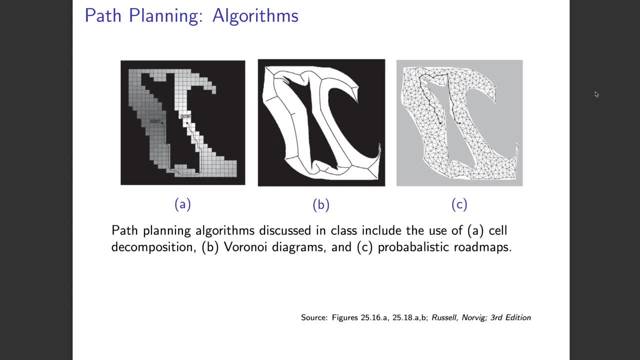 we're going to talk about today, And the idea is that we're just selecting random points in space which aren't in infeasible regions, They're not in space, They're in occupied space- And then we're just connecting them to the kind of neighboring states. 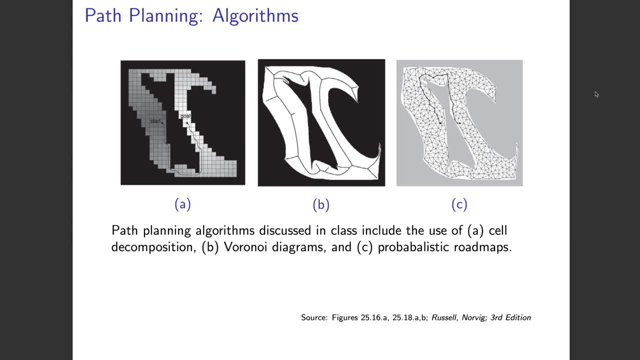 And then we're using that kind of roadmap that we've created and doing a search in there. So, similar to that first problem, the algorithm A, we're kind of turning this continuous space into a discrete search problem, What we'll be talking about today, however. 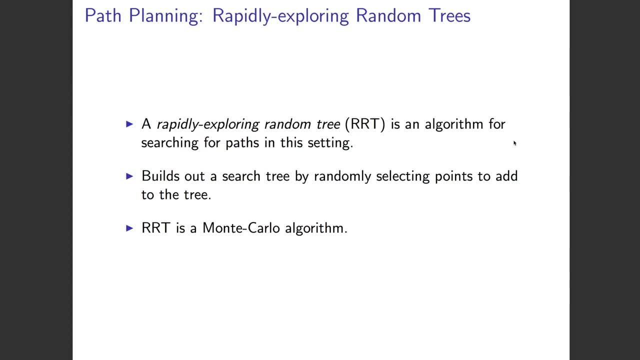 we won't be touching on the lectures- is called a rapidly exploring random tree. So this is an algorithm that we'll be discussing which solved just this problem. We've got some starting space, we've got some ending space, and we want to find a path between the start and the end. 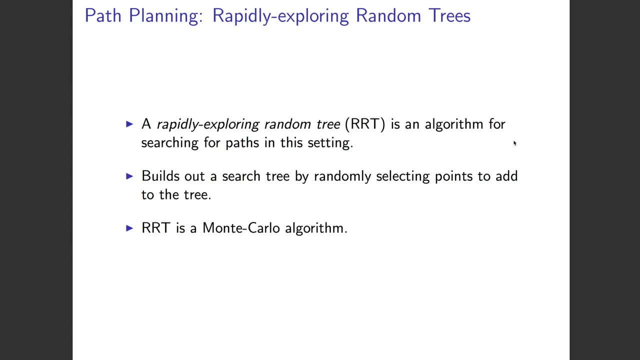 The way this works is: it starts out, it builds up a tree. it starts out, the tree starts at the root, and then it just randomly samples points and adds them to the tree. When we're doing this random sampling, this becomes a Monte Carlo algorithm. 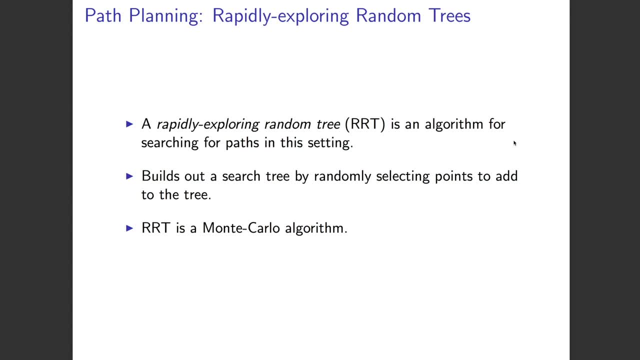 So Monte Carlo algorithms are a family of kind of algorithmic methods that uses random sampling to solve complex problems And we can see, or we will see, a few different ways that we can tune this algorithm to work well for this setting. Some of the reasons it does work well for this setting are: 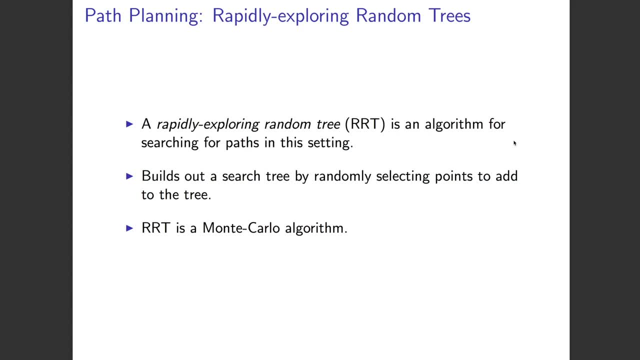 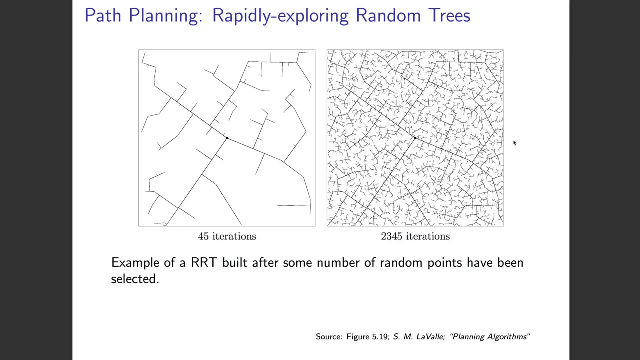 it can deal with non-convex spaces, it can deal with higher dimensions and it doesn't need any kind of. it doesn't need some discrete space. It can work in continuous space. So, really quickly, an example of how this might work. 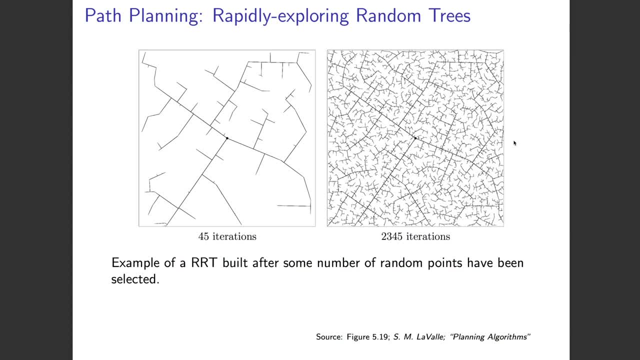 These depict some RRT that we've built. Each line is an edge between two points in our tree, I guess. visualized like this it just looks like a graph, but really that center node is the root and then everything coming off that is a tree. 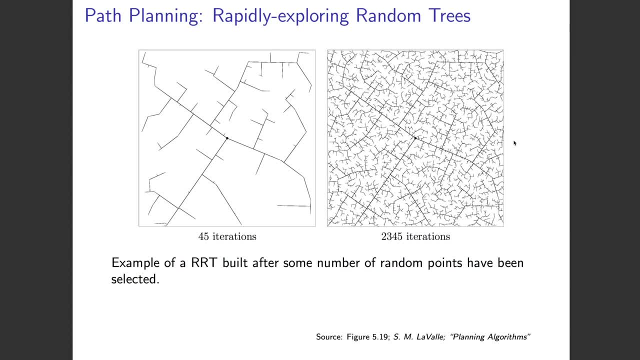 And it's what we call a space-filling tree. So, as you can see on the right, after more iterations we've filled a lot more of the free space with these points, and then that's the edges which are depicted here, And eventually, if you ran it for long enough, 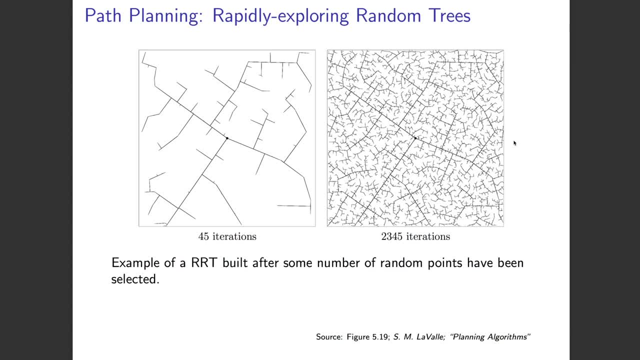 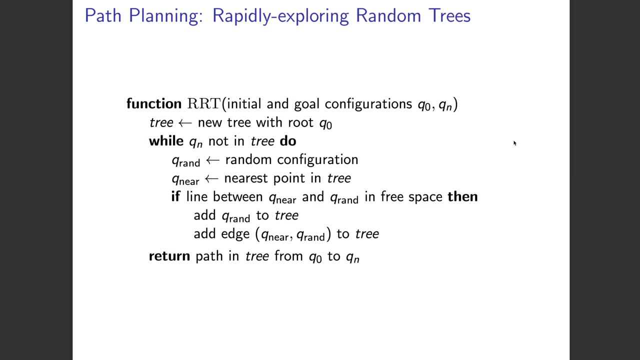 it would fill all of the space. So if you had one goal spot and you had an initial configuration, after enough iterations you will actually reach that goal, as long as it is reachable. All right, Let's go over a little bit of pseudocode for this algorithm. 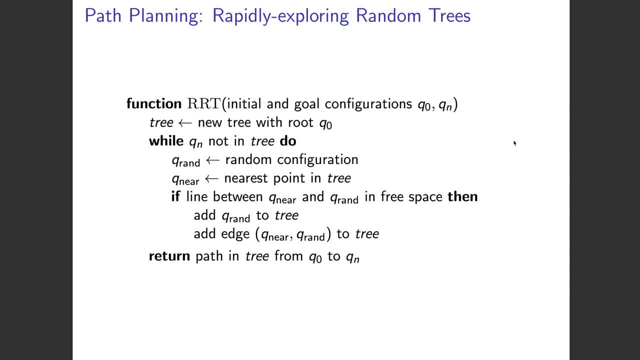 And then, after we've done that, we'll jump into a demo see if we can write some Python code to get something like this working for the problem I had, which is that two-jointed robot with a configuration space from before. So again, 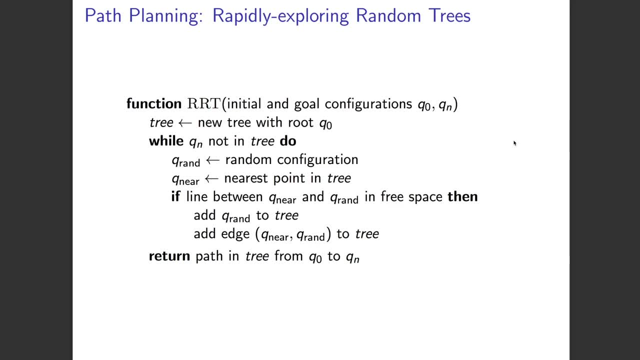 the rapidly exploring random trees algorithm takes in configuration space coordinates. So we're assuming that that transformation from the workspace to the configuration space and then back again we're assuming that that's already been dealt with in some other part of the program. So we're given the initial configuration. 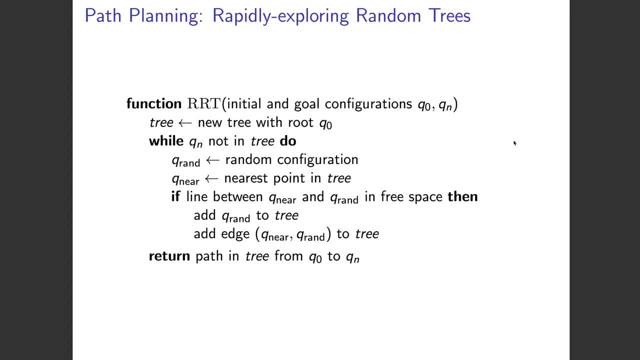 and the goal configuration and we want to start building out this tree. So we're going to initialize it as a new tree with the root as the initial configuration and then we're just going to keep building out the tree until we've found the goal state. 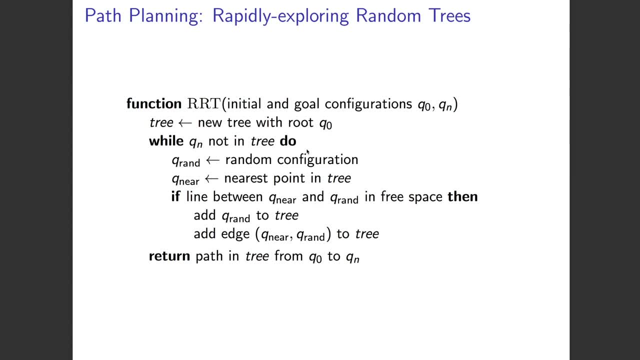 and that's a part of our tree. Once it's in the tree, we can just search for the path between the root and the goal. So what we do is we find some random configuration, and we'll talk a little bit more about how we do that efficiently. 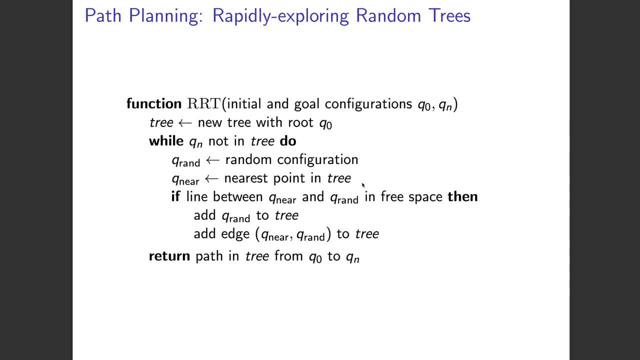 We find some random configuration and then we find the closest point in our tree to this new random configuration, which is not in the tree. By drawing a linear line between them we can see whether or not the transition between this nearest point and the new random point. 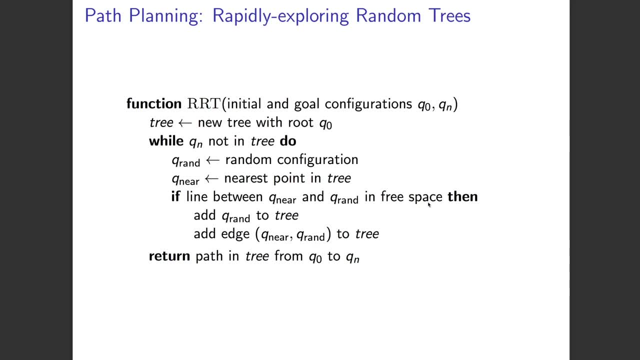 is feasible, ie it's contained entirely within the free space. and if it is, then this new random point can be a new vertex in our tree. So we'll add that point to the tree and add an edge from the nearest point. 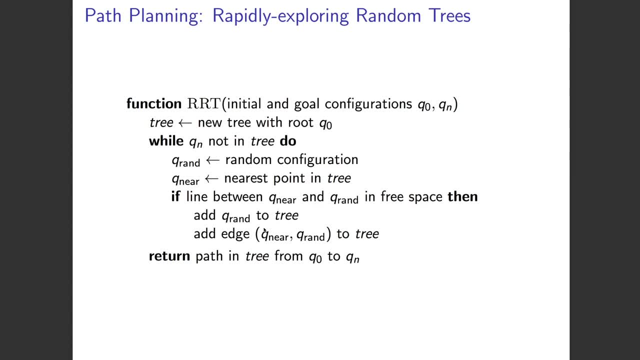 to that new vertex. Once this wild loop finishes, we'll have actually found the goal configuration, and then we can just return the path from the initial configuration to the goal configuration. One of the questions we'll have to answer is: do we need exactly the goal configuration? 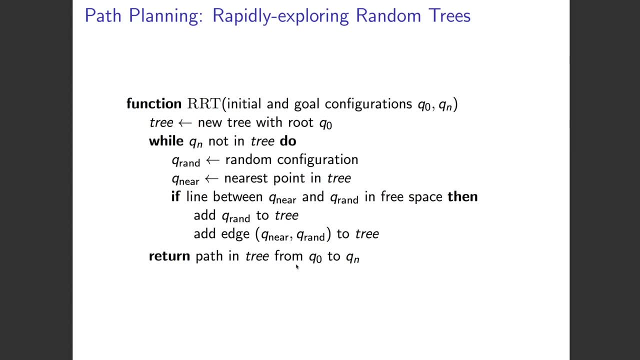 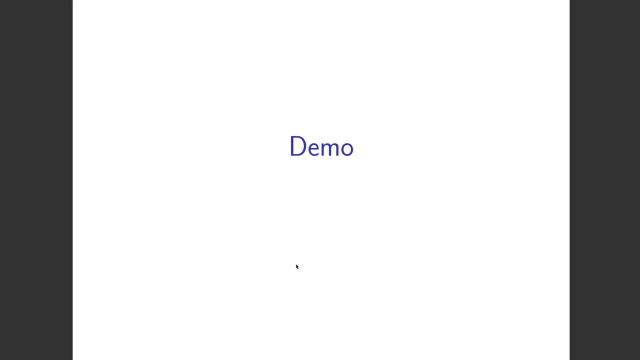 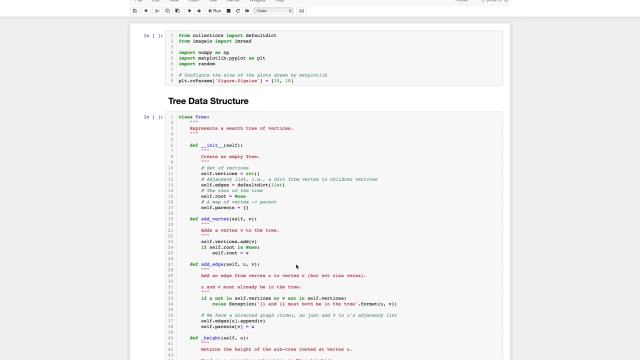 or maybe we can just get close enough. So we'll think about that in a minute. All right, I'm going to jump right into a demo and we'll see how we go. All right, so I've got this Jupyter iPython notebook up here. 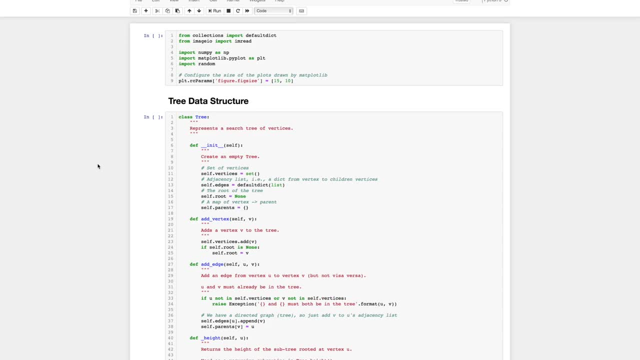 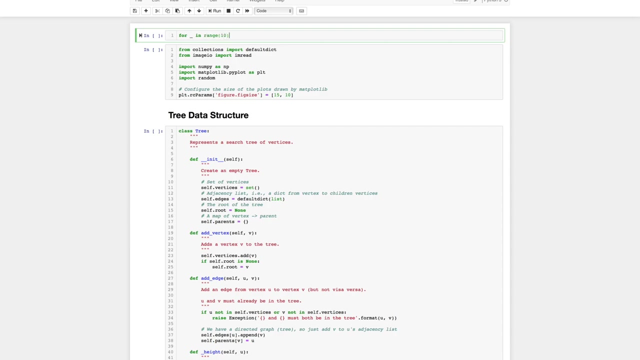 If you guys aren't familiar with that, we'll post some details about some pages you can go to to find out a little bit more about this. but essentially it's just an interactive Python shell, So as an example I can just write some Python code here. 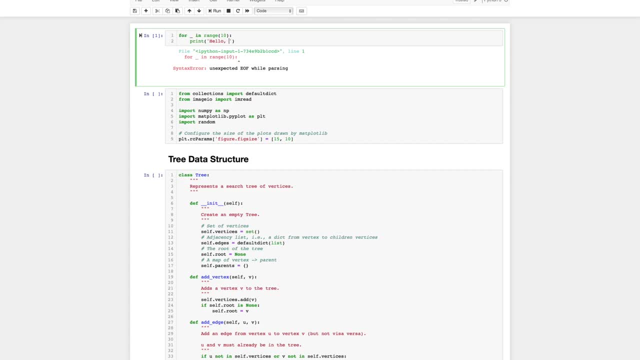 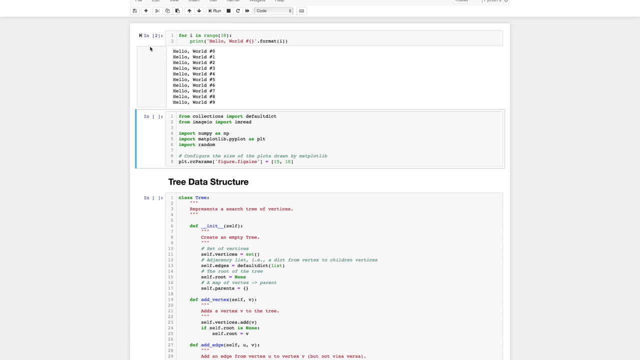 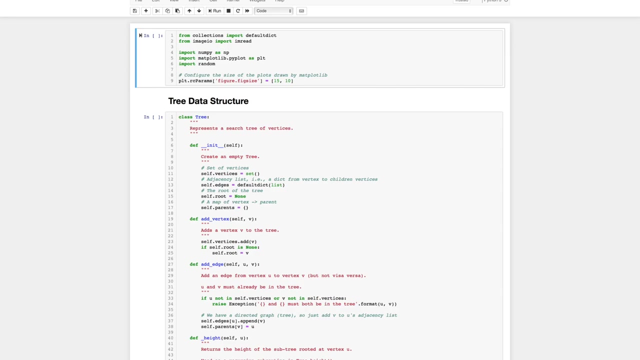 Oops, And I can execute that there. So I can execute things in line and the variables we create in cells will persist over these kind of Pythonic cells. So, to get started, we're just going to import a few of the libraries that we need. 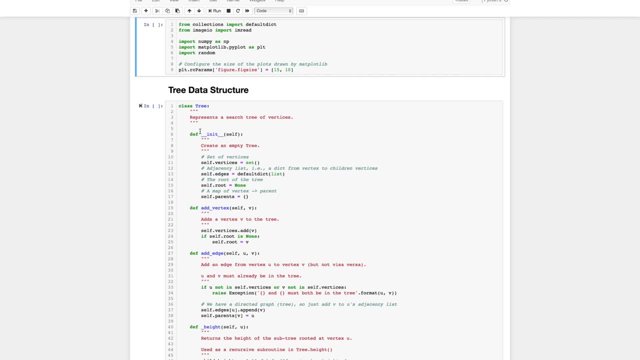 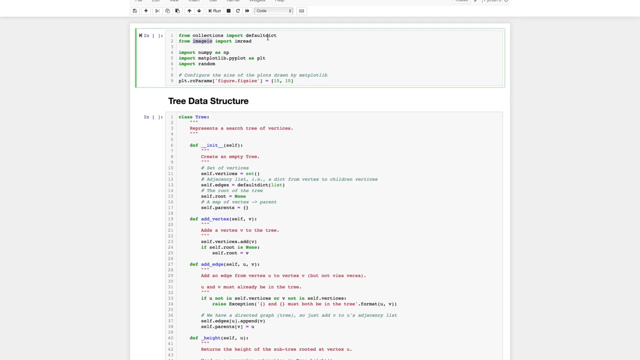 We're going to use matplotlib to visualize this algorithm. We're going to use NumPy to do some of the computations, And then we've got this imageio package which will help us read the configuration. We're storing our configuration spaces as images. 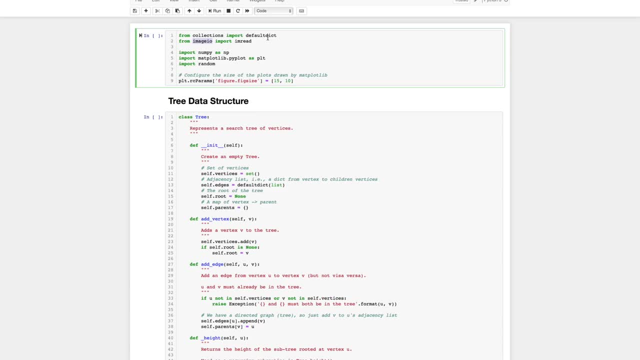 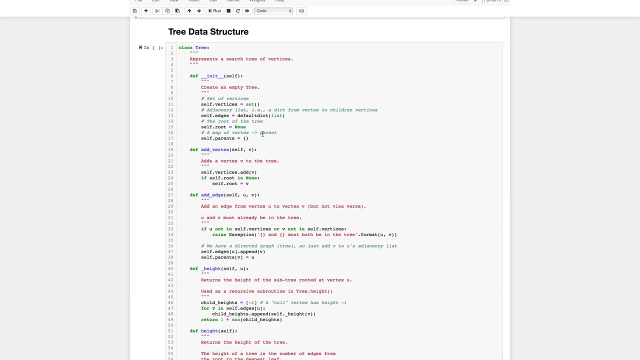 and we're just going to treat black pixels as occupied space and white pixels as free space. So the first thing we're going to need to do is create some tree data structure. One of the things we're doing in the algorithm from before is querying this tree and adding and building up this tree. 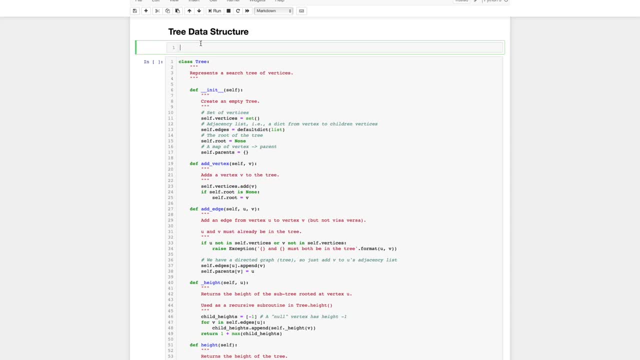 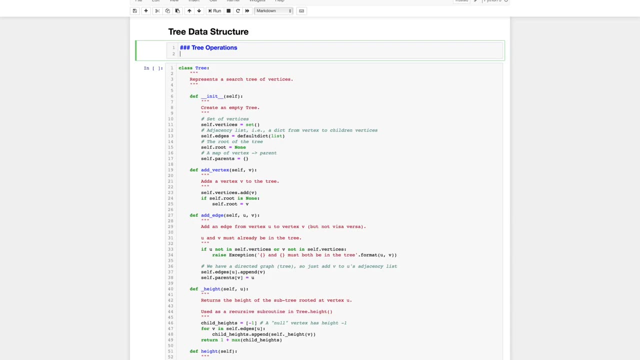 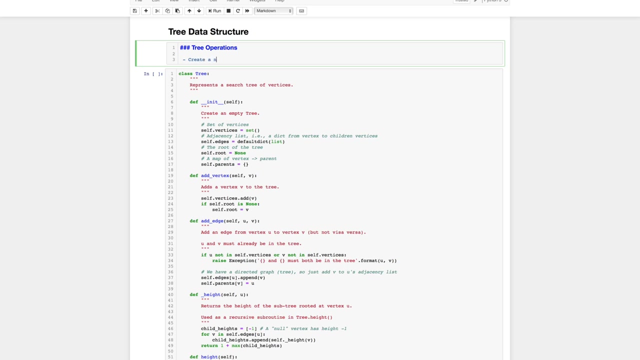 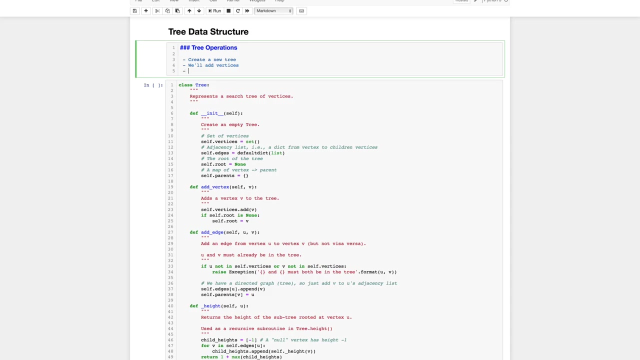 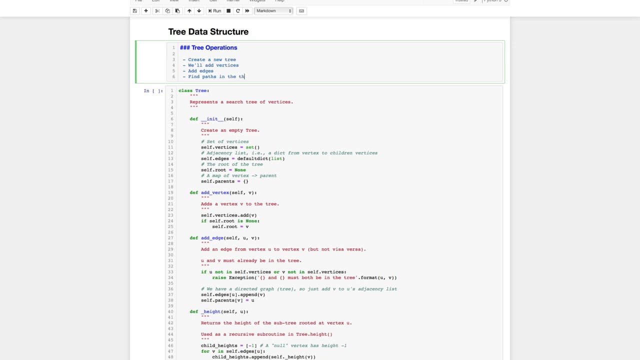 So what are the things we're going to need from this? Well, we're going to need to be able to create a new tree. We'll want to be able to add vertices, add edges, find paths, find paths in the tree. 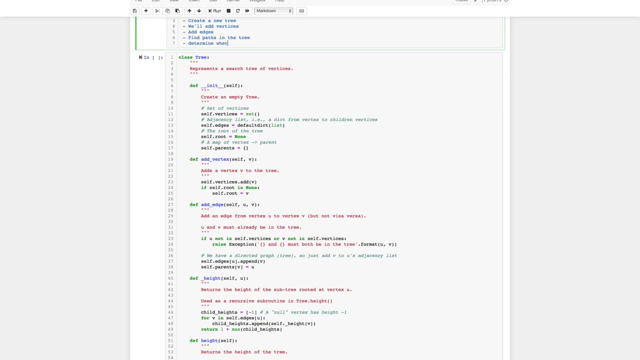 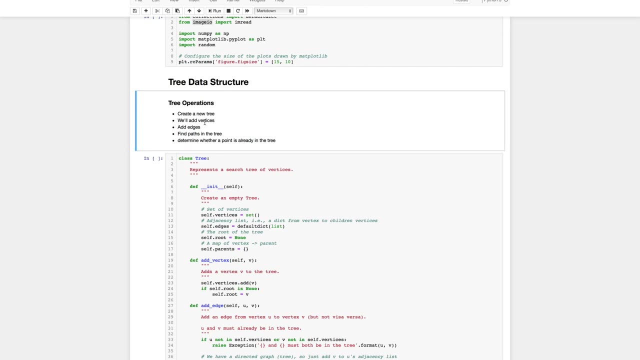 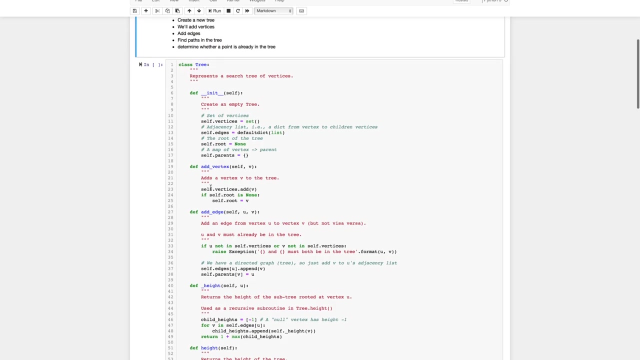 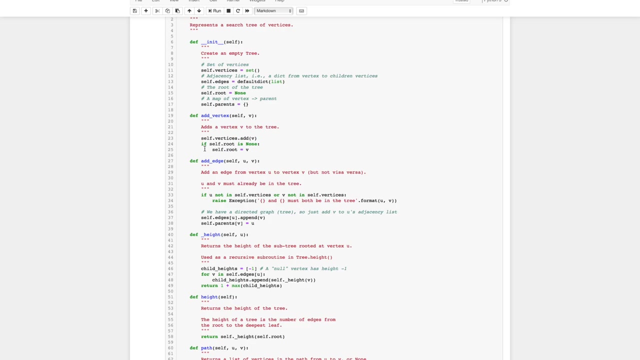 and determine whether a point is already in the tree. So these are the goals that we want our tree to be able to satisfy. The way we're going to store this is with a set of vertices, A set of edges- Well, actually an adjacency list of edges. 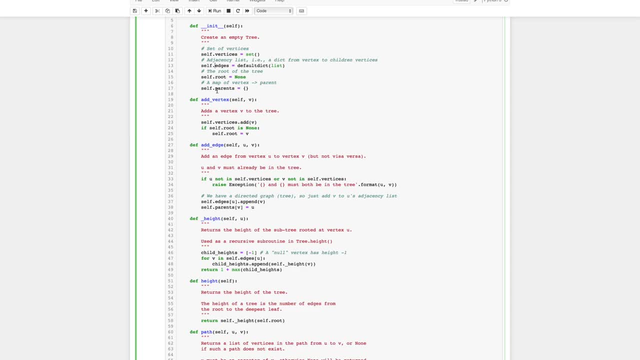 We'll store what the root is and we'll also keep track of the parents of each vertex. That way, if we're searching for a path between two points in the tree, we'll just go to the lower-down point and we'll just search up the tree until we find the original point. 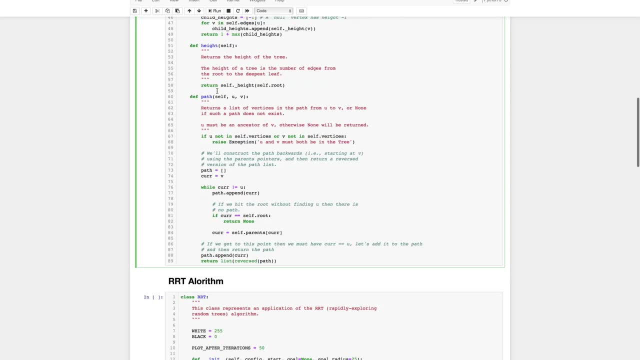 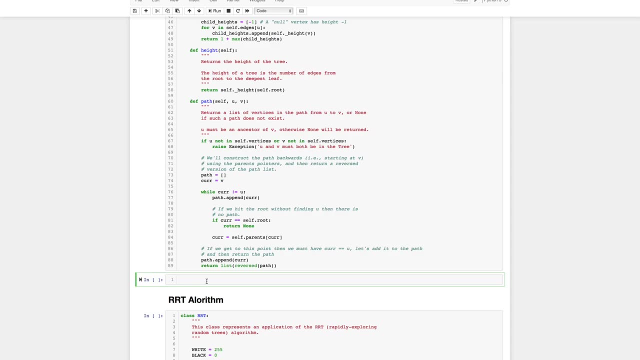 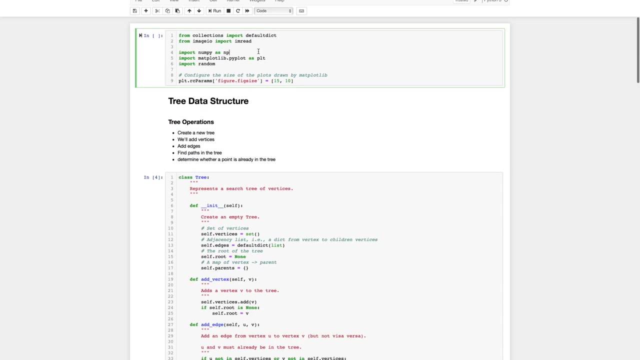 So I'll post this code on the LMS so you guys are able to have a read of it. If you're interested in how the implementation works, which is just a quick demo, let's say we've got some new tree here. Bear with me to import all of this. 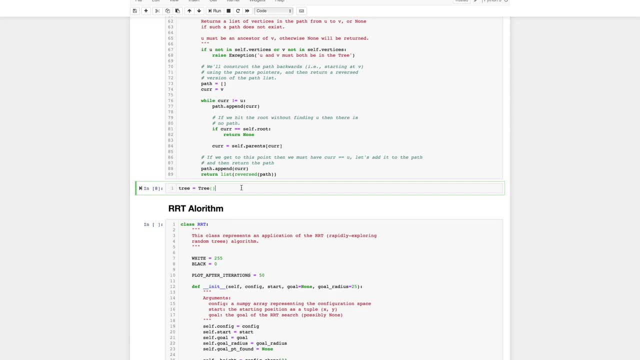 Alright. what's going on There? we go Alright, so we've got some tree. If we print out the state, well, we've got the vertices as just an empty set And the edges will be an empty default dictionary If we were to add vertices. 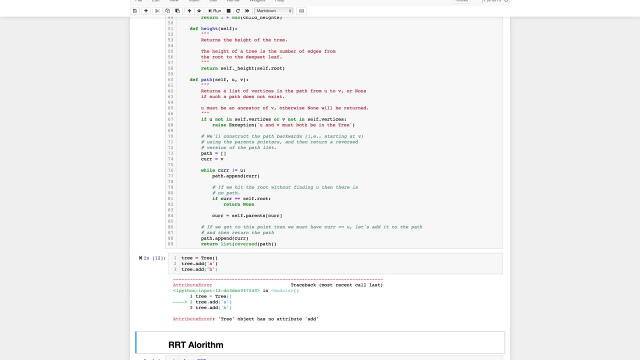 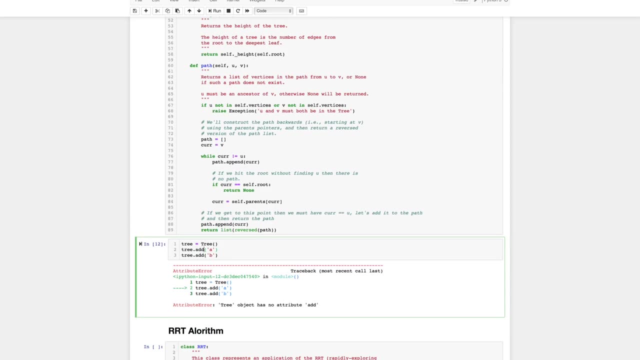 maybe we add A and B. Whoops, What is it? Add vertex And we'll add an edge between A and B. Let's now inspect this. So the vertices should be A and B, which it is, And the edges will say: 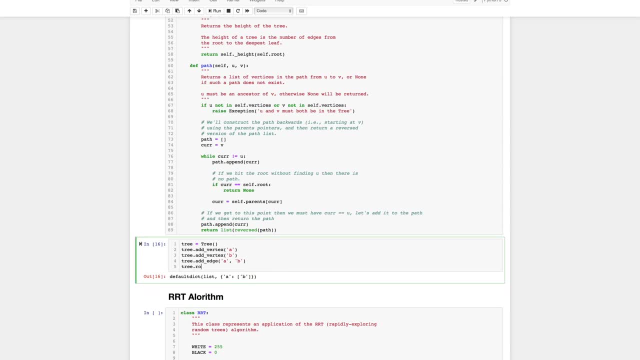 well, from A we can get to B, So that's an adjacency list. The root should be A, because that's the first vertex we added, And if we want a path from A to B, well, that's just one edge we need to follow. 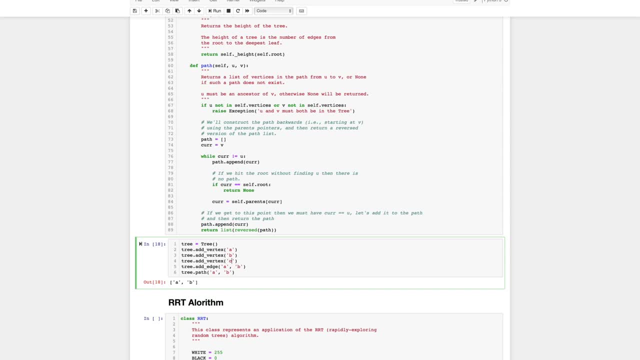 If we were to add another vertex. so this is going to be a stick that looks like A at the top, B as its child and then C as B's child, And then we want a path from A to C. It'll tell us that we need to go from A to B to C. 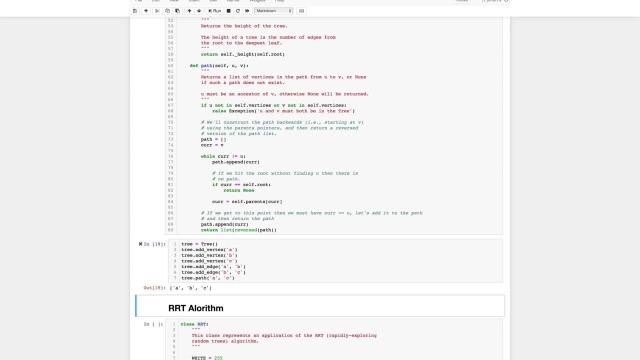 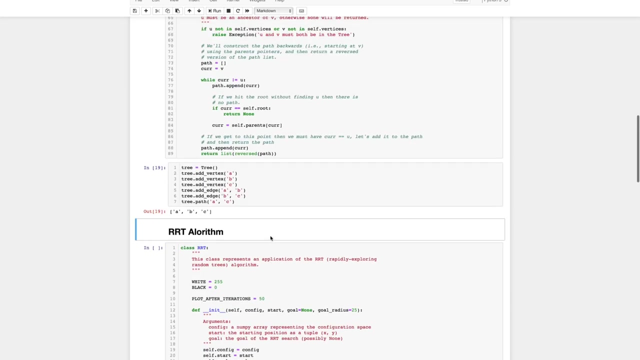 So this will be useful when we're backtracking in our algorithm, when we've found a path from our initial configuration to the goal configuration. Excuse me, All right, So that's this tree data structure that we're going to need to use. 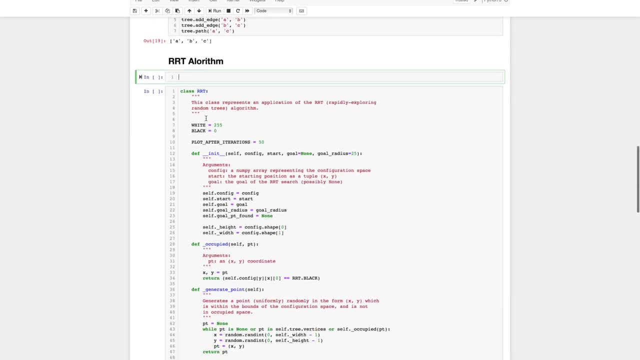 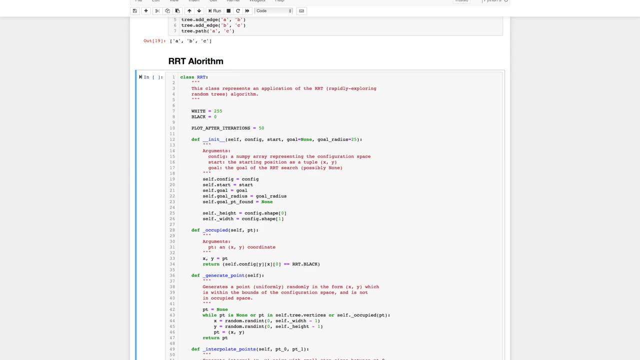 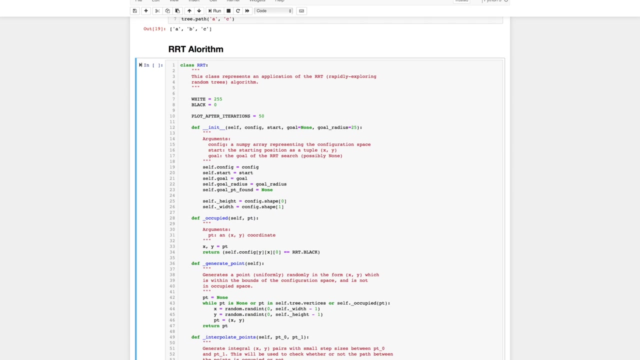 The next thing is we're going to implement the rapidly exploring random trees algorithm. So one of the choices I've made here is that I'm going to implement this algorithm as a class, So, rather than a function, which is normally how we'd implement an algorithm. 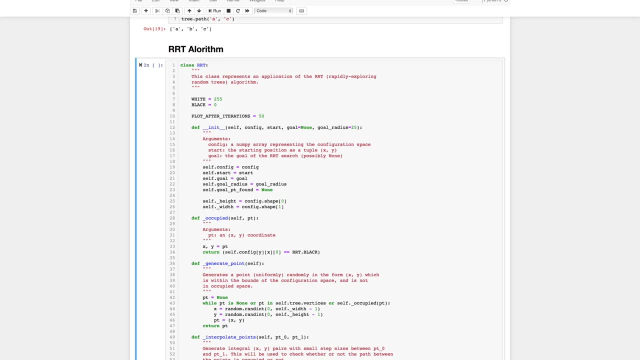 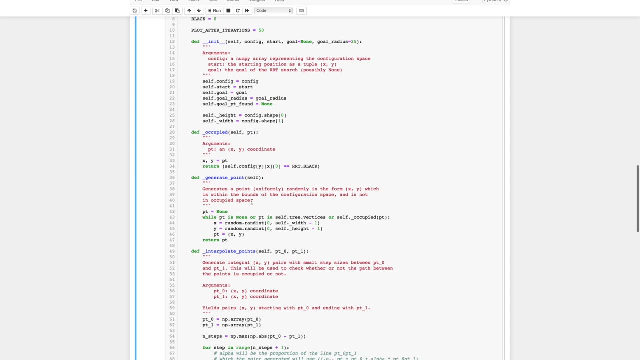 I'm going to use a class, an object, just so that we can source some state, and that's going to make our lives a little bit easier. It also means that we can kind of group all of the intermediate functions that we'll be using. 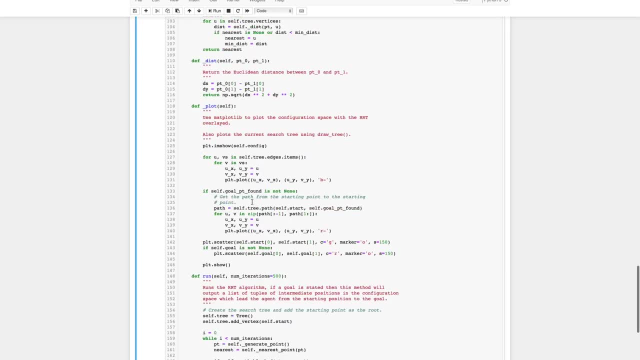 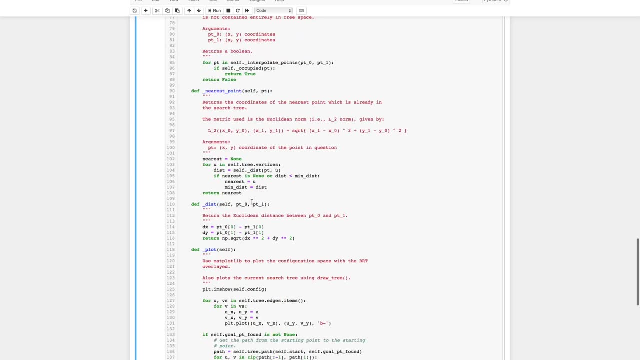 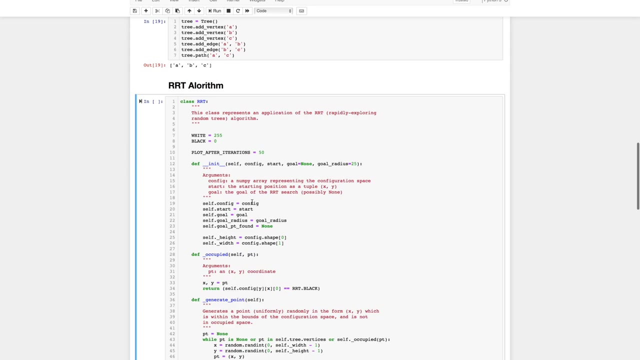 to make this a nice, easily readable piece of Python code. You'll notice that I'm using docstrings and kind of keeping my functions nice and short. So how are we going to go about this? Well, let's have a look. Well, all right. 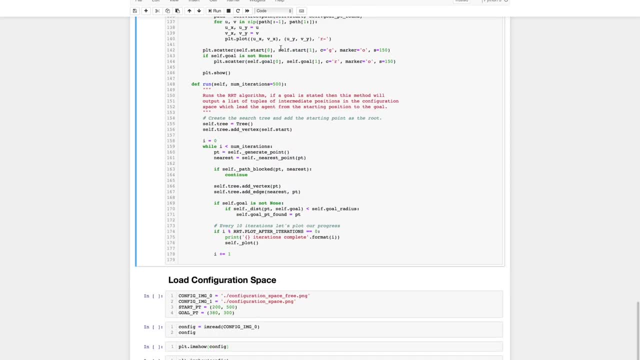 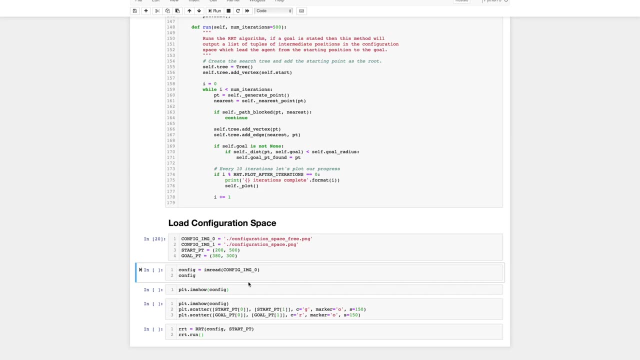 You know what I'll introduce: a little bit about the setting that we're going to be working in, and then we can go and actually implement the algorithm ourselves. So down here I'm loading the images. So you can see when I load this image. 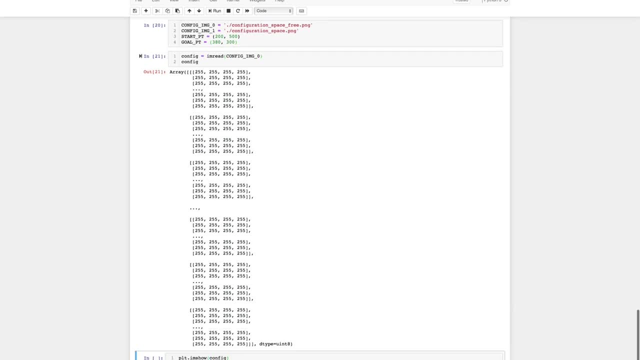 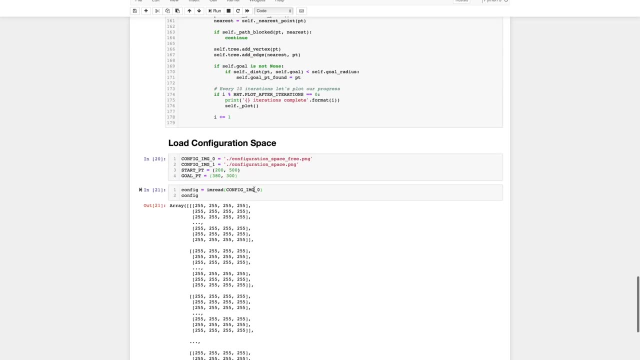 I actually just get an array of pixels, It's just a numpy array, And then we're able to use matplotlib to plot that. So this is just free space. It's just going to be a white image, But if we load the configuration from the book, 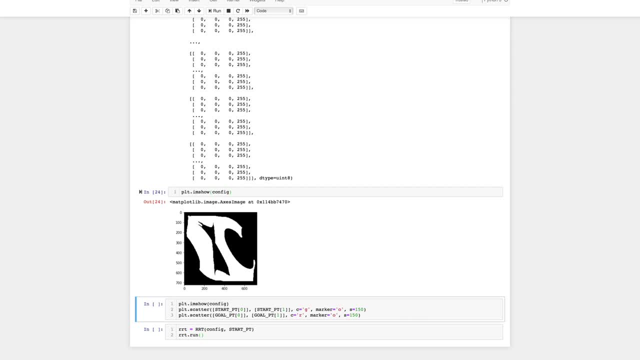 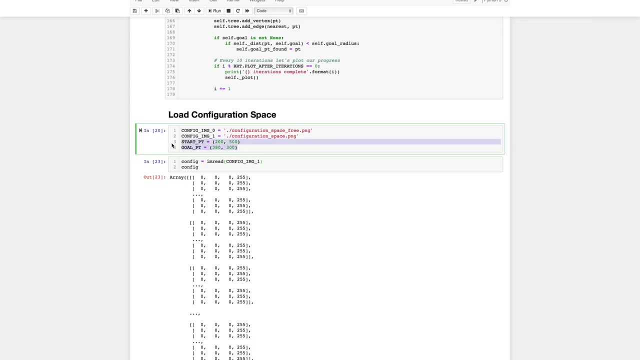 we get this, which is just what we saw on the slides. One of the things we might want to do here is we can add a starting point and a goal point, which I've defined just here, And to plot that we can just use this pyplot command. 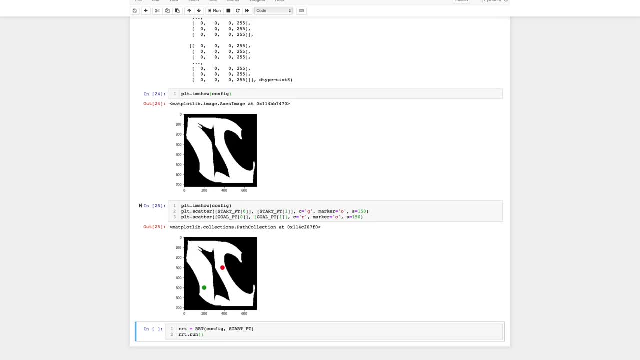 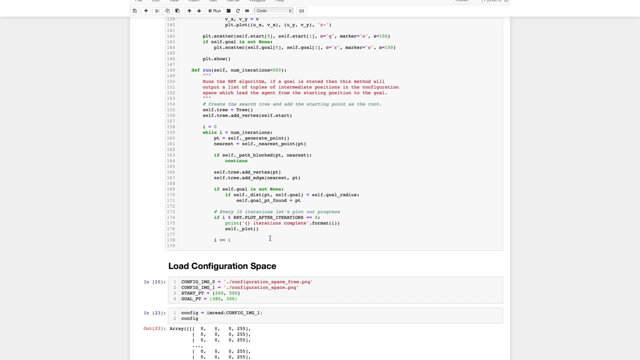 So there we go, We've got. the green is our initial configuration and the red is our goal state. All right, So let's have a think about how we can implement this algorithm. So I've done it beforehand, So I'm just going to get rid of this. 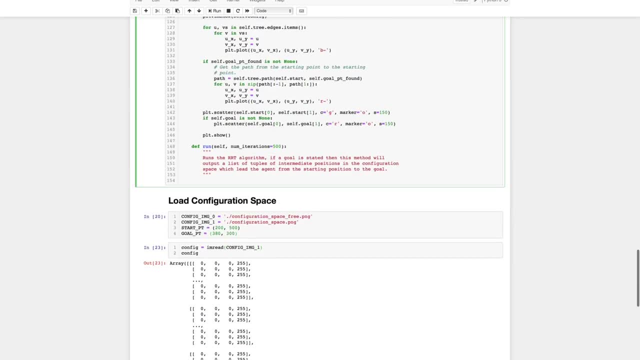 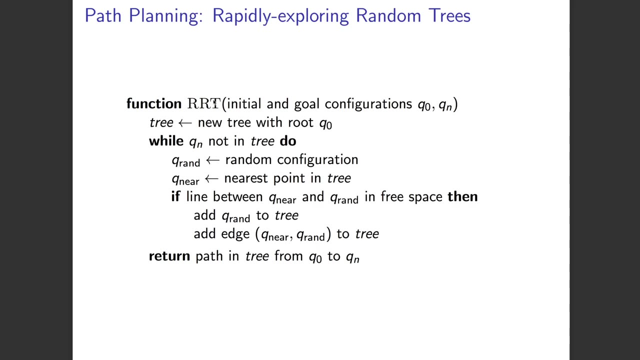 And let's start from scratch. So what's the first thing we're going to have to do? Well, if we go back to our slides, the first step in the pseudocode is to create a new tree. So let's do that. 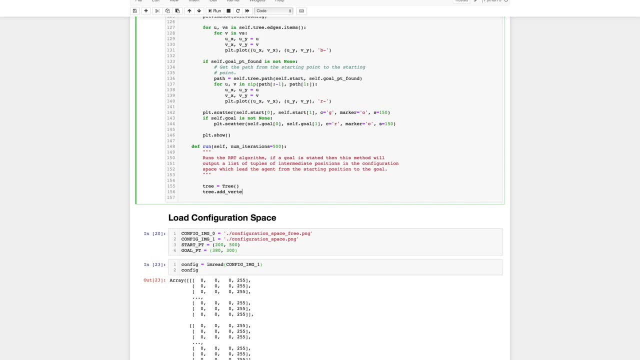 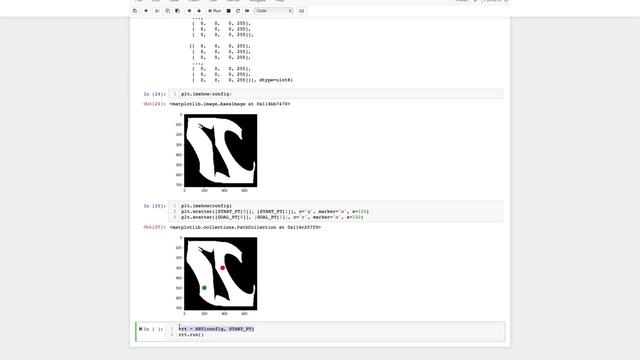 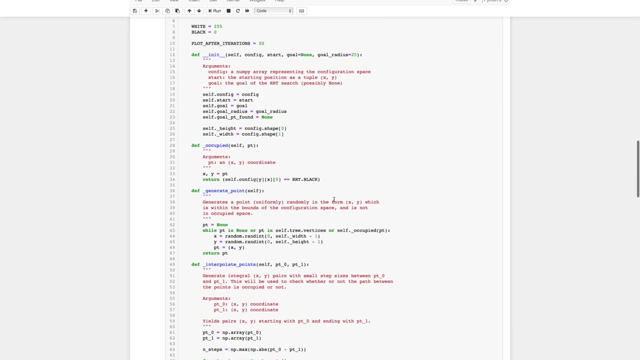 Let's just create a new tree And we'll say: we'll add a vertex. And what's that vertex? Well, down here we have initialized this algorithm class with a starting point, And we can see here that we saved this starting point as selfstart. 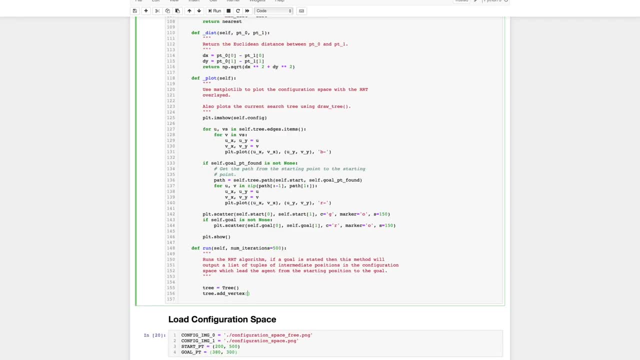 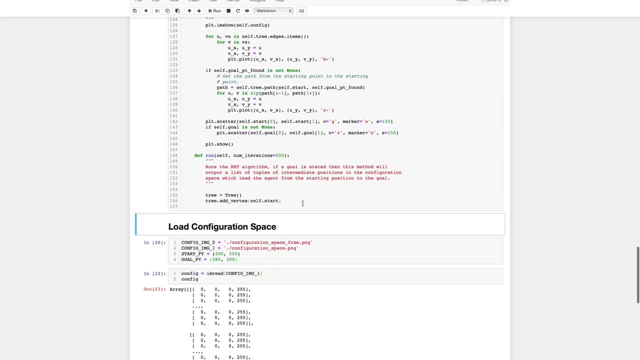 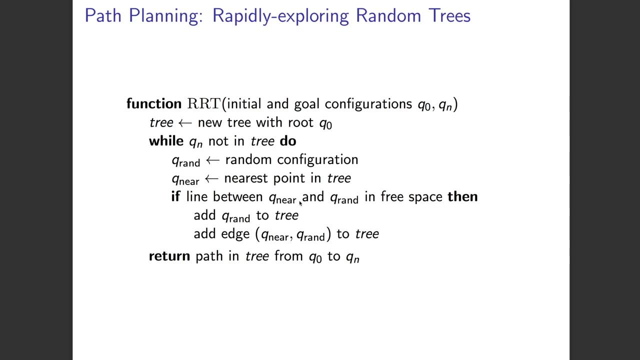 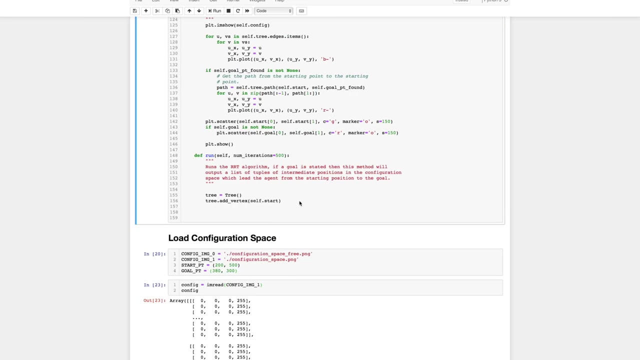 So let's say that the first vertex in our tree is going to be selfstart. Okay, What's the next thing I want to do? Well, the algorithm from the slides says that we should iterate through until our goal is found. At the moment, 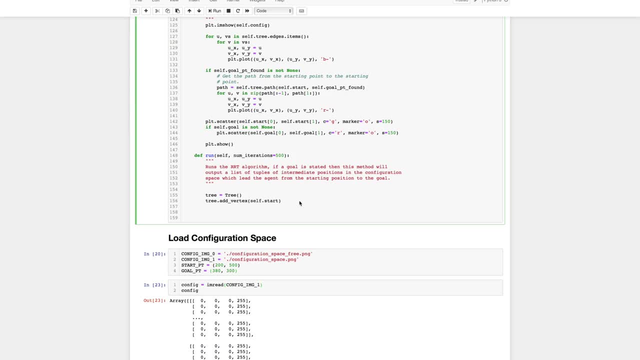 just so that we're programming this algorithm incrementally. let's not worry about a goal, Let's just worry about building out this rapidly exploring random tree, And then we can have a think about how we check for whether or not we've seen a goal. 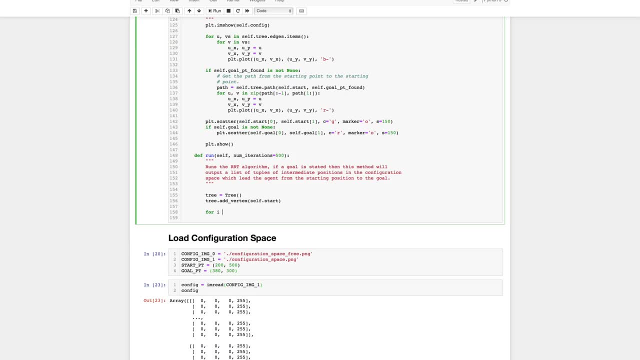 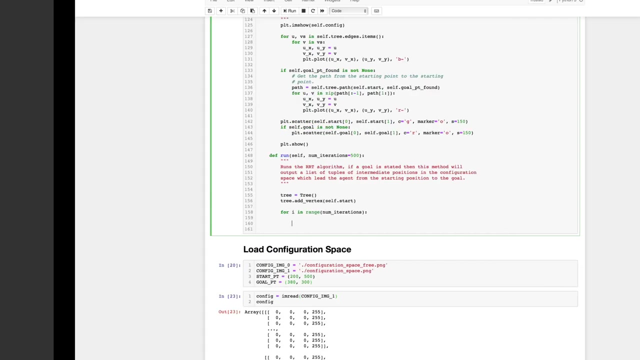 So what I'm going to do is I'm just going to do some number of iterations. By default, it is 500, as you can see just here. And then what are we going to do? each iteration? Well, the algorithm says that we should choose some random configuration. 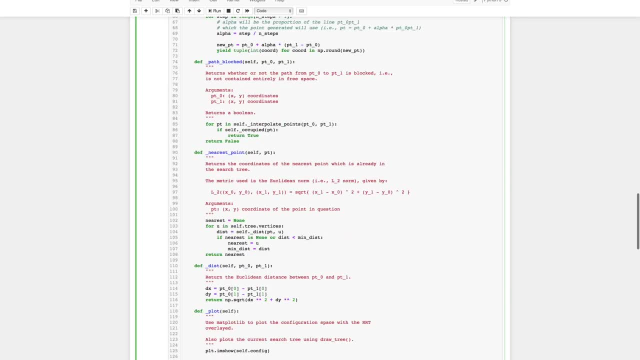 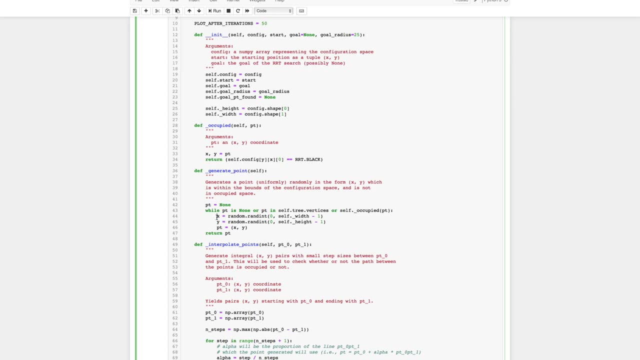 So let's do that. I've written this function generatePoint, which should generate a random point. So what we're doing is we're generating a random XY coordinate that fits within the bounds, But we're not returning it until we find one that is not already in the tree. 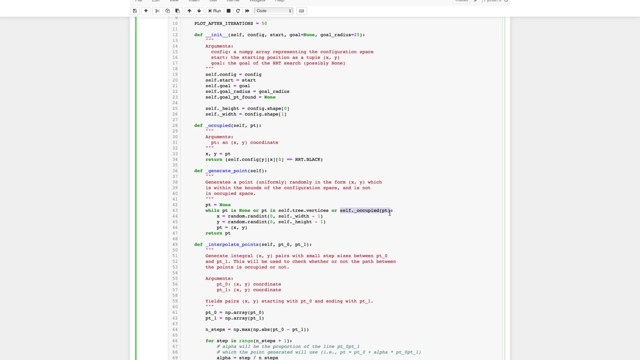 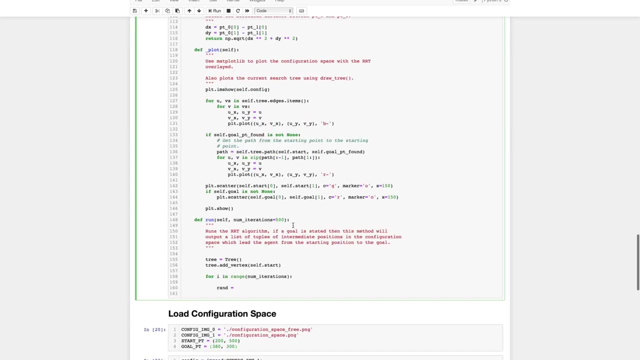 and which is not lying in occupied space. So the way we check if something is occupied, we're just checking whether or not the image has a black or a white pixel at that point. So what we could do is we could just say self generatePoint. 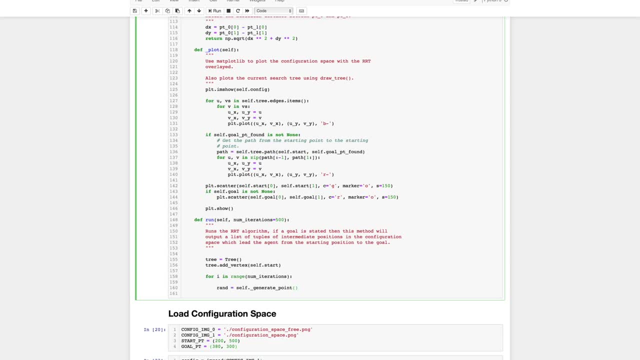 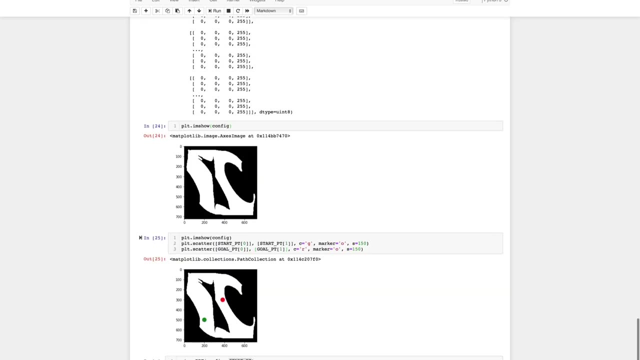 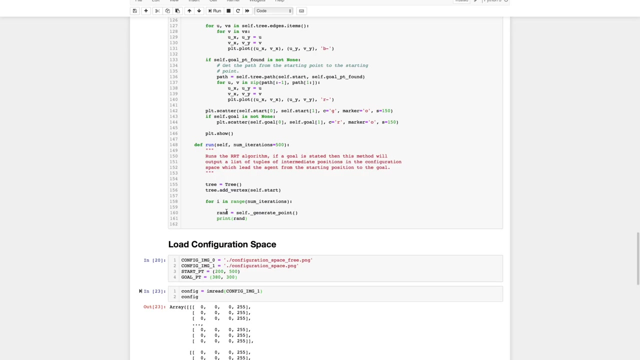 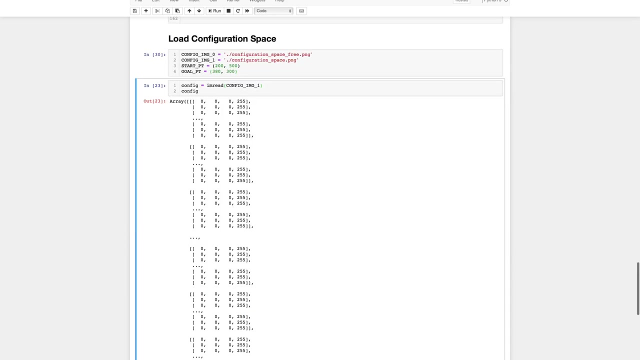 And I might just print some of these out just to make sure that it's working properly. So let's do that, And we go down here and let's run this code. So here we've got tree. We just want this to be a field of our class. 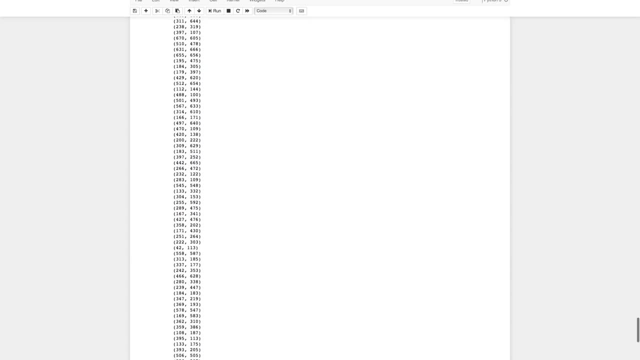 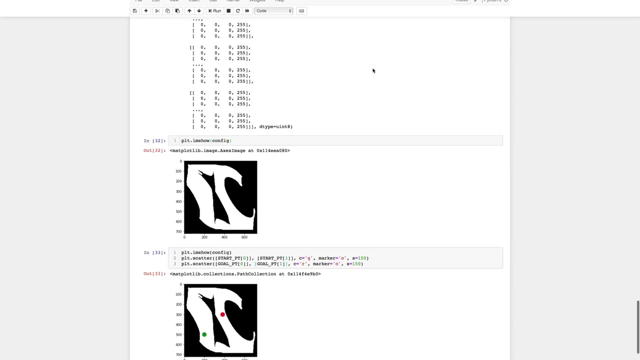 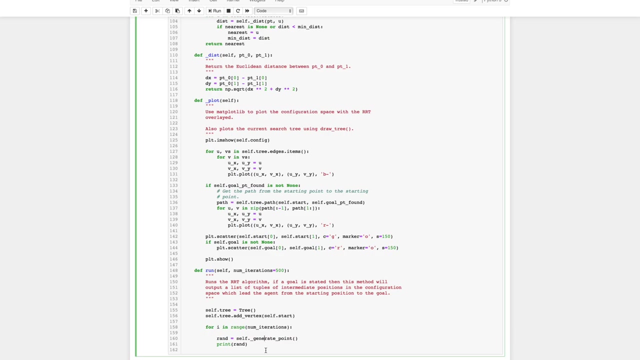 Cool. So we're generating a bunch of random points. There should be 500 of them. How are we going to confirm that these are actually, in fact, not in occupied space? Well, let's have a think. Perhaps we can return these and then plot them. 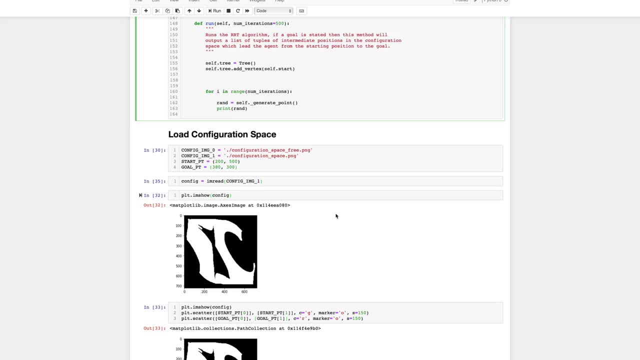 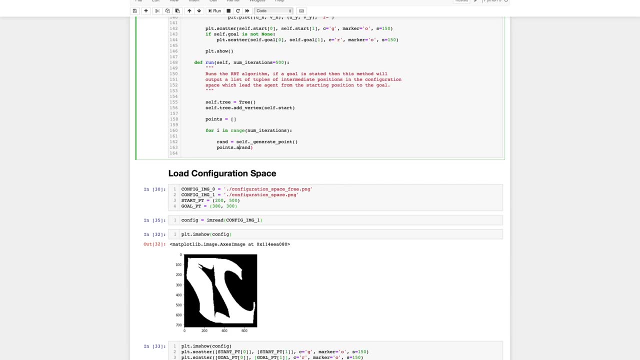 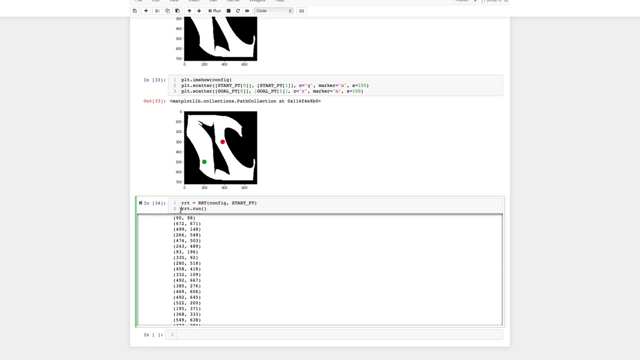 That should be an easy enough way to tell. So let's just keep a list of the points And we'll just add these points and return them once we're done. So now this should return some points array. Let's check, Looks good. 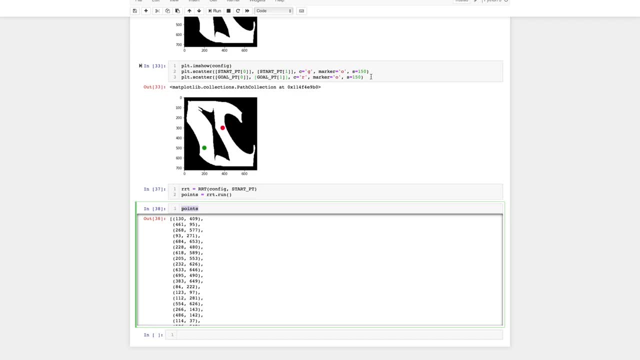 Okay. So how are we going to plot these? Well, above here, we've got this scatter function using PyPlot, which is to create a scatter plot, but it also is going to allow us to just plot a collection of points on our image. 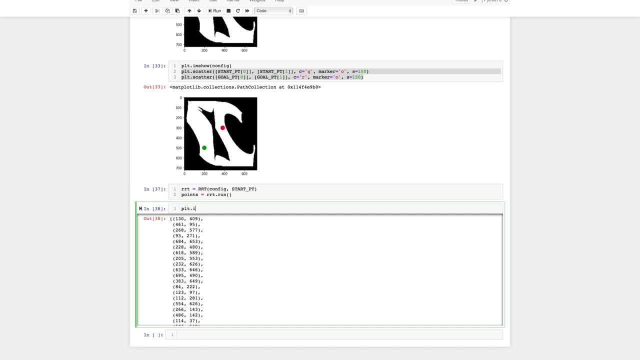 So what are we going to do? Well, show the image, which is the configuration, And then we're going to have all the x coordinates and all the y coordinates. So to create them, we'll just say, well, it's all the points. 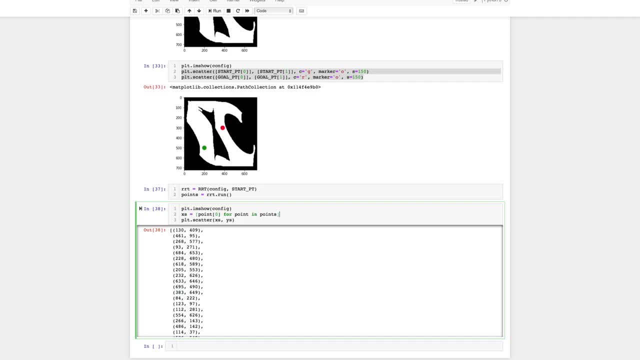 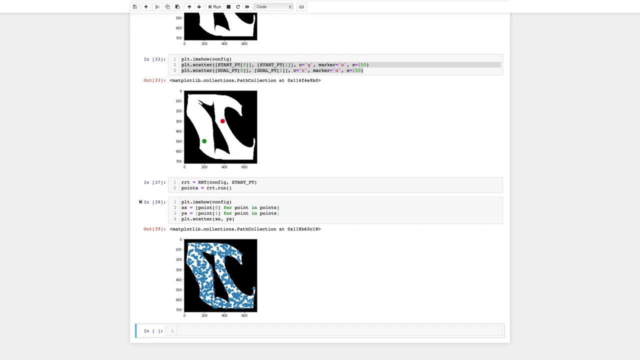 in the points array. However, we just want the first coordinate And we're going to have the second coordinate, Same for the y's. That's just going to be the second element in each tuple. Looks pretty good. All of our points do indeed lie in the free space. 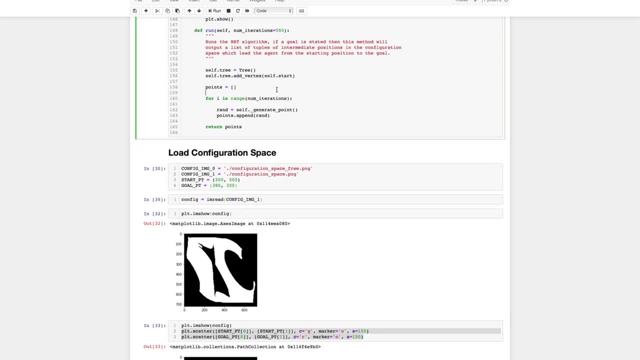 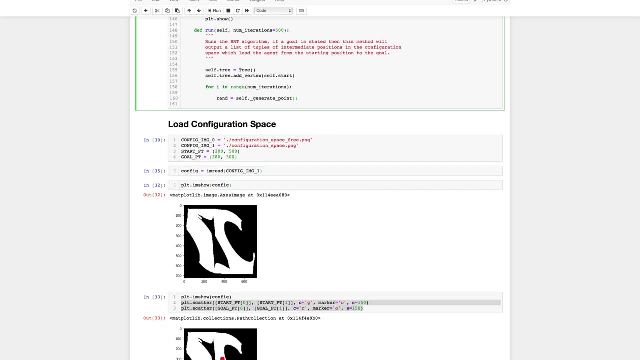 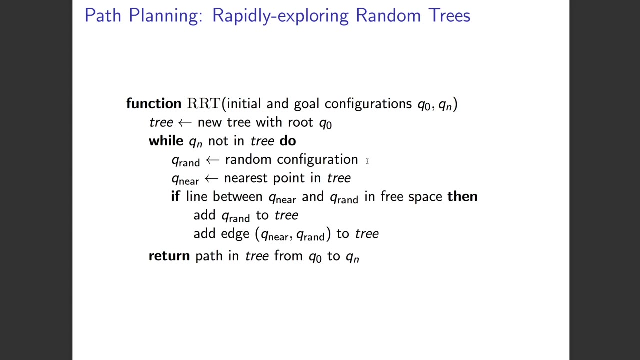 So I think we can move on. So let's get rid of this auxiliary code that we've written. Okay, So what is the algorithm going to do next? Well, once it's found a valid random configuration, we need to figure out what the nearest point. 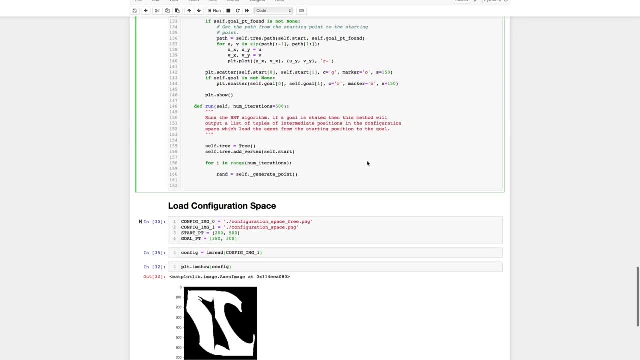 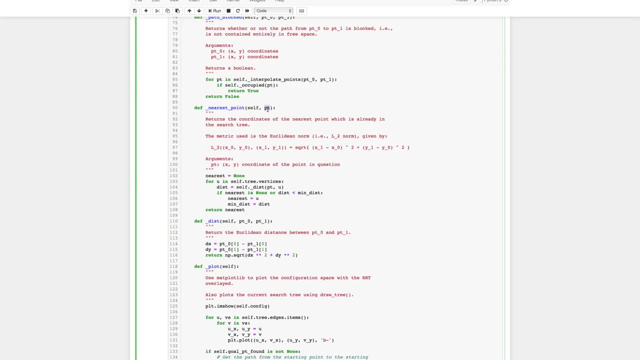 that we've already added to our tree is. So I've already written a function that does this, called nearest point. So the idea here is: we're given, we give it the random point that we've just created and it's going to find us the vertex in the tree. 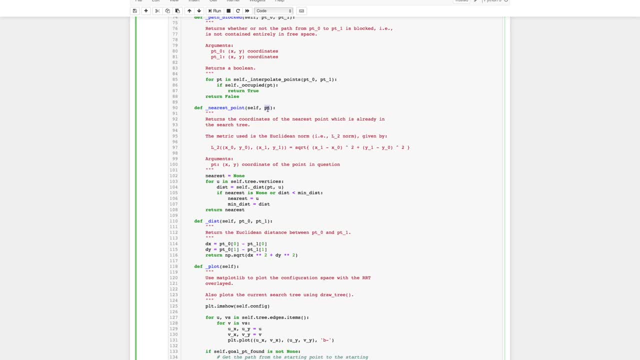 which has the smallest Euclidean distance in configuration space coordinates to that point. This is going to be a linear time algorithm which, looking over all of the the vertices in the tree, we're keeping track of the smallest distance. This distance function just calculates the Euclidean norm. 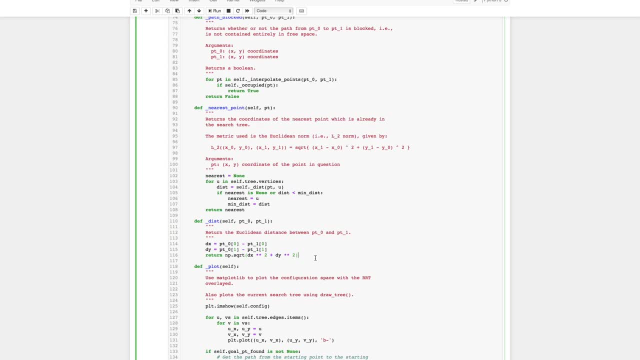 as you would expect, which is just the difference between the x coordinates and difference between y coordinates, both squared and then taking the square root of the sum of those. So we'll find the minimum distance point and then we're going to return that point. 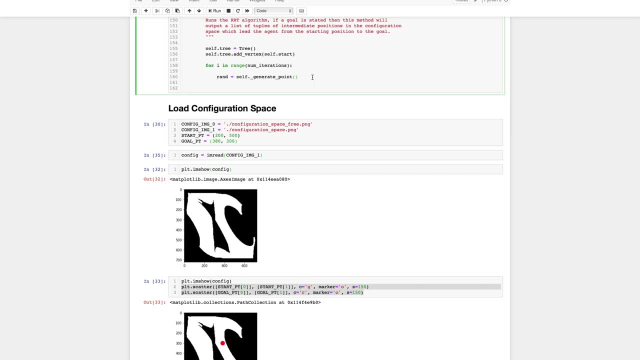 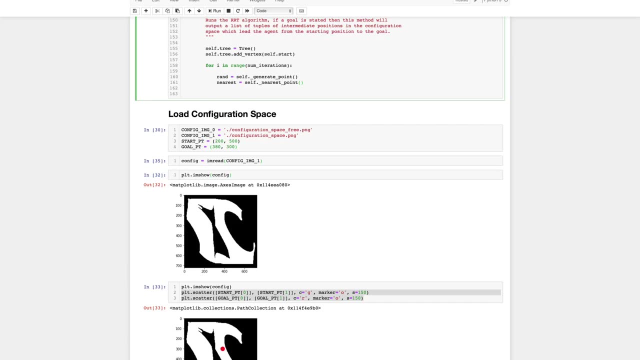 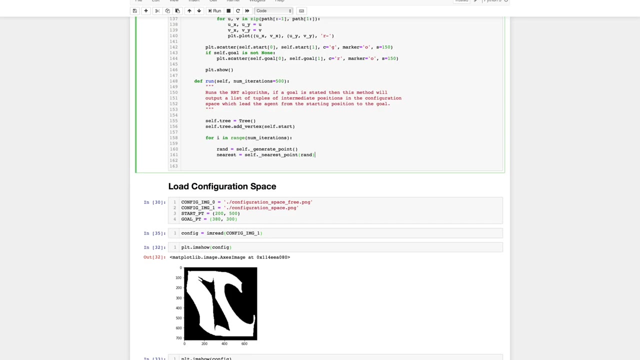 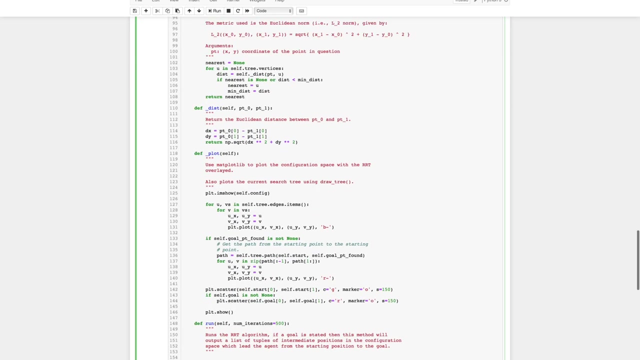 So how might we be able to visualize this? Well, first of all, we'll actually find that nearest point and we'll give it the random point, And then I would like to plot the edges between these nearest points. So if I have a look at the function I wrote before, 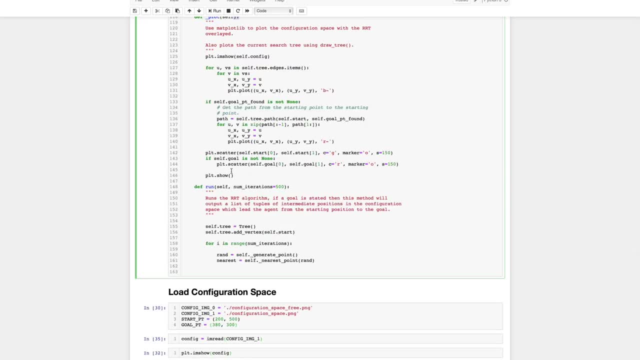 this plot function. I should be able to use this plot function. So what we're going to do is we're just going to say plot image, show the configuration, and then we'll plot well, the first coordinate of the random point and the first coordinate of the nearest point. 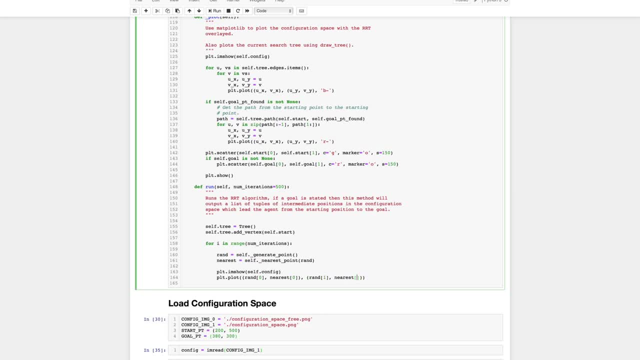 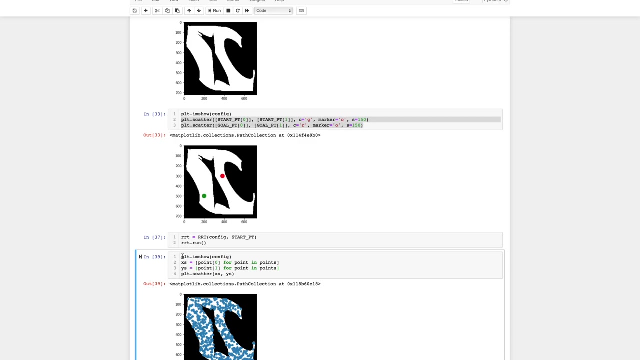 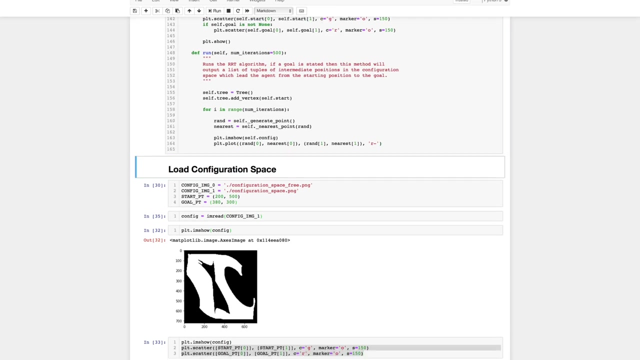 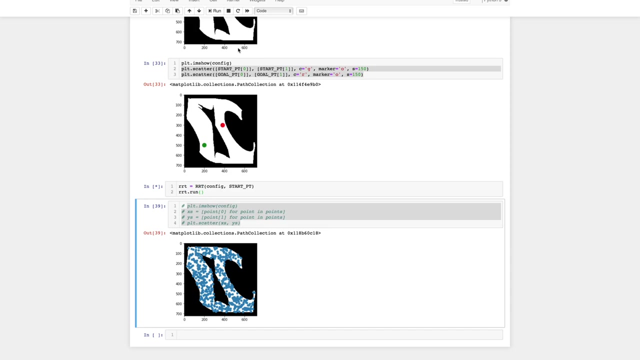 and then the second coordinate. So these are the x and y coordinates respectively, And let's go red. Let's try this. We're not returning the points anymore. We'll comment this part out. How are we going? I wonder what's going on. 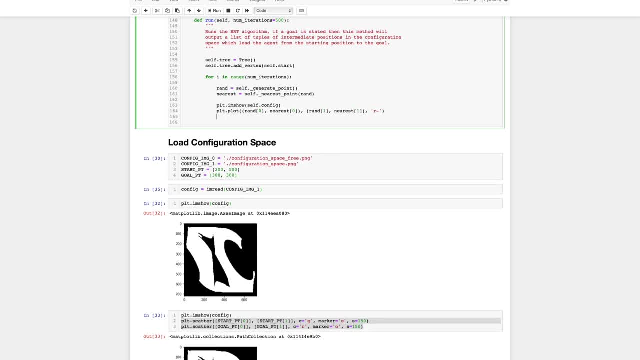 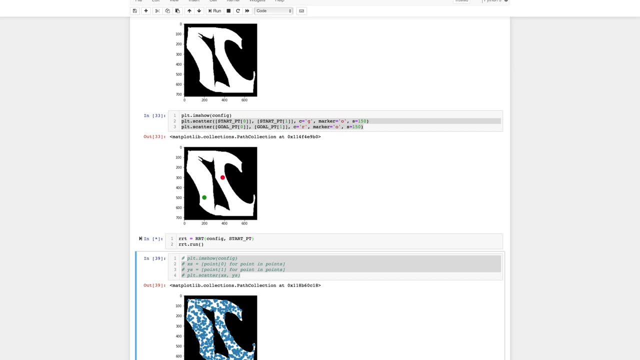 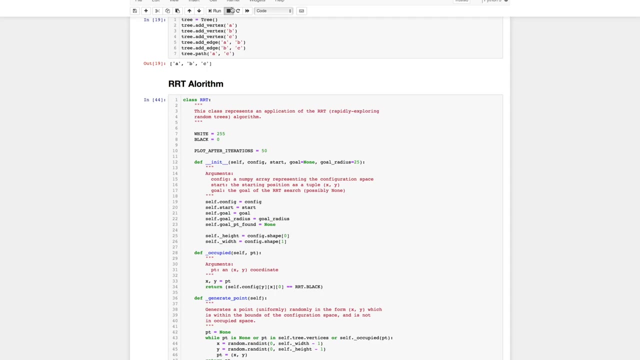 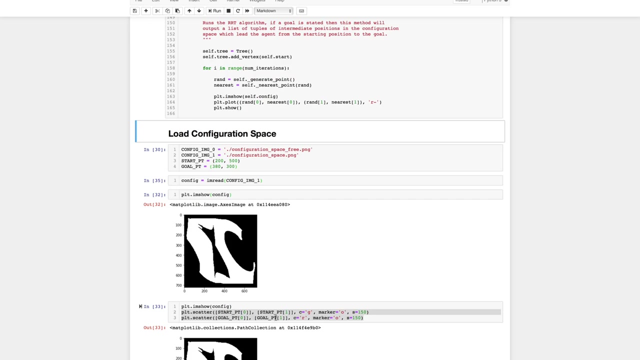 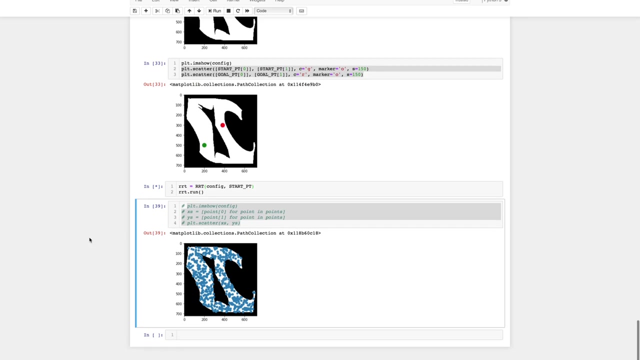 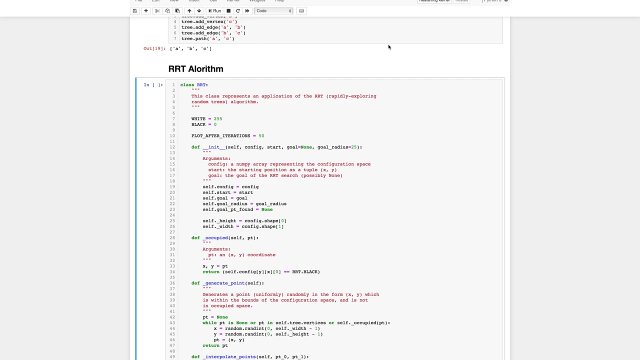 OK, Ah, They want to show the plot. Maybe that's our issue, No dice, Oh yeah, Just as I gave up. All right, Let's go again. Anything happening, This shouldn't take a while to execute. Let's just restart and run everything again. 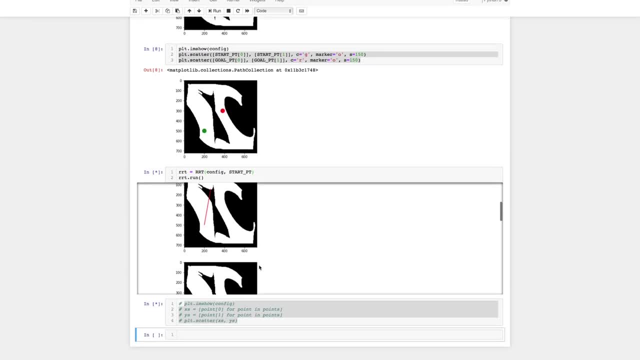 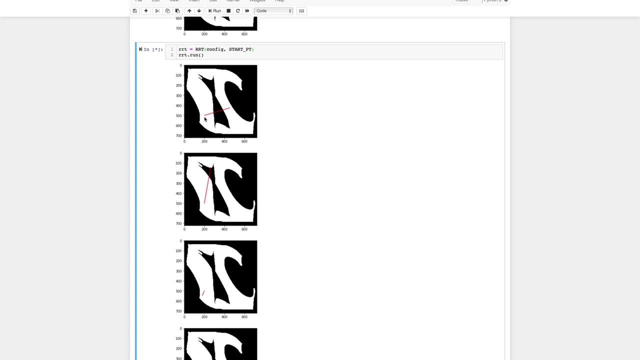 There we go. All right, Great, So we're getting these points and a line between the random point and the nearest point. At the moment, we haven't added any new points to the tree except for the root, So its nearest point is always going to be. 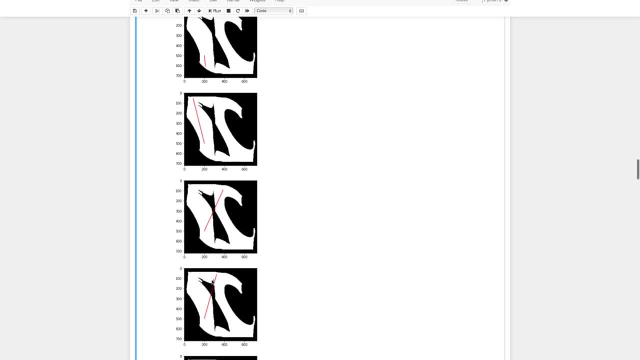 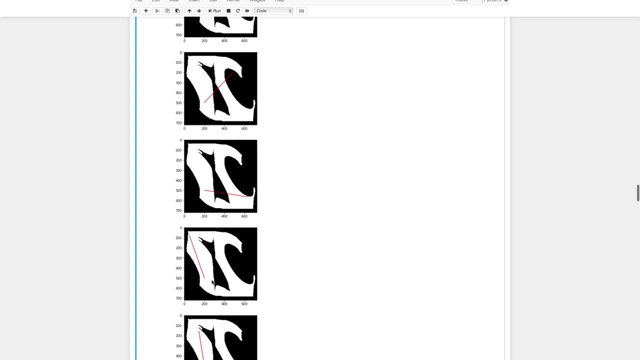 this starting position that we've specified, But it looks pretty good. We're finding points in random space and we're drawing a line between them. However, what's the issue here? Well, we can see that the majority of these lines- this one, for instance- 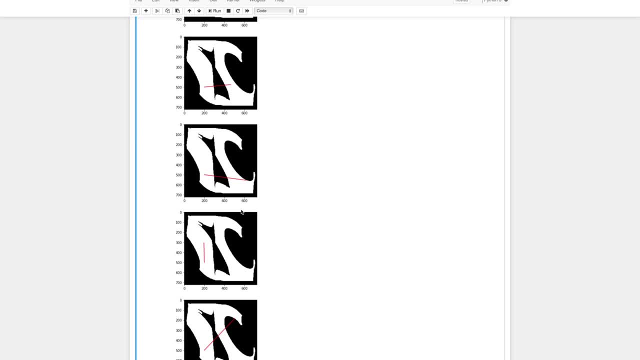 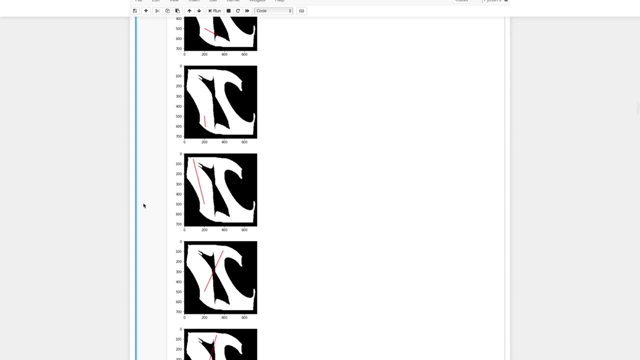 doesn't actually go entirely within free space. It's crossing these obstacles and it wouldn't actually be a valid path for our robot to take. So what can we do about that? Well, there's a few ways that we could deal with this. 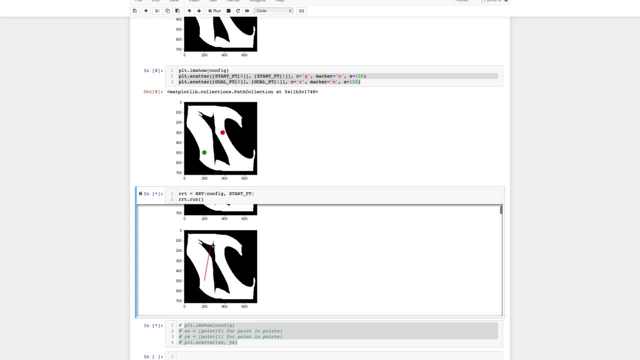 One is we could just cut short. So if this is our edge, then maybe we could choose this point on this side of the obstacle. How would it make our life easier? Well, let's just discard that random point if it is the case that its nearest point is an obstacle away. 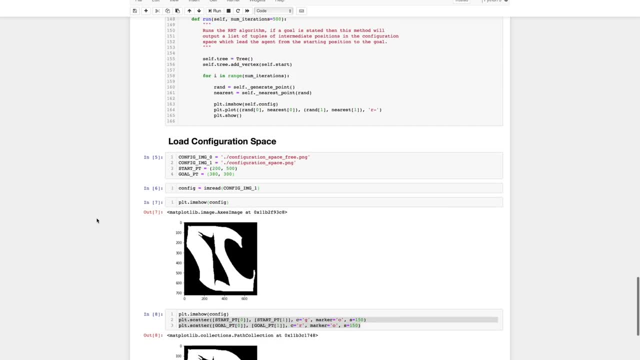 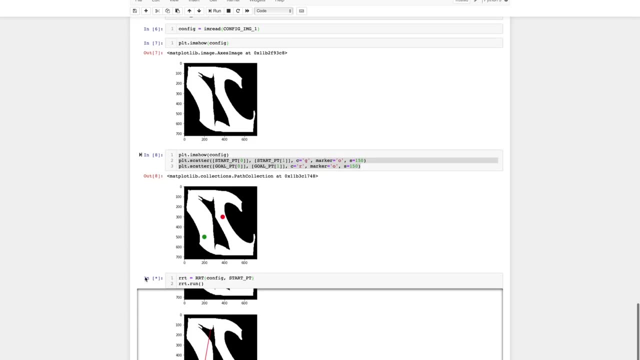 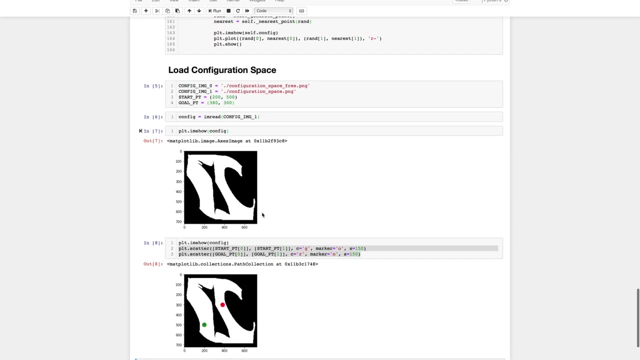 If there's an obstacle between the nearest point and it. So let's just only choose random points such that the line between them is entirely in free space. So, excuse me, I'll stop that function, All right, So what are we going to do? 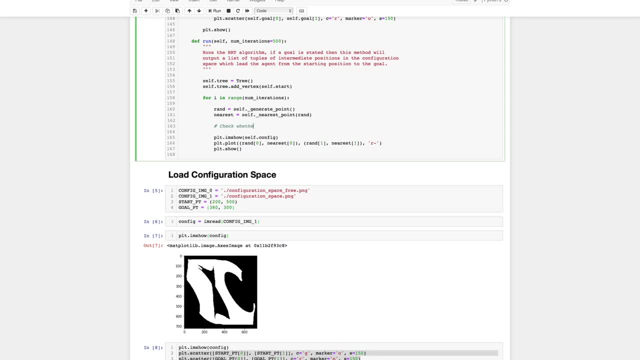 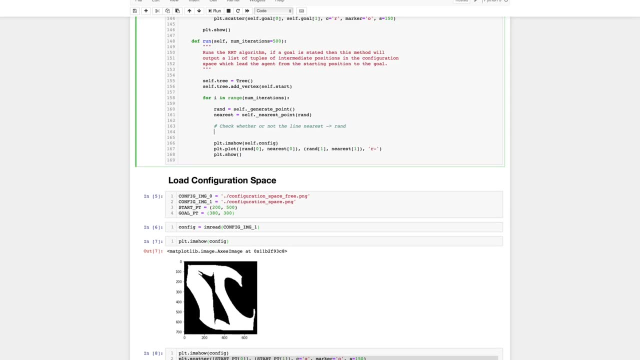 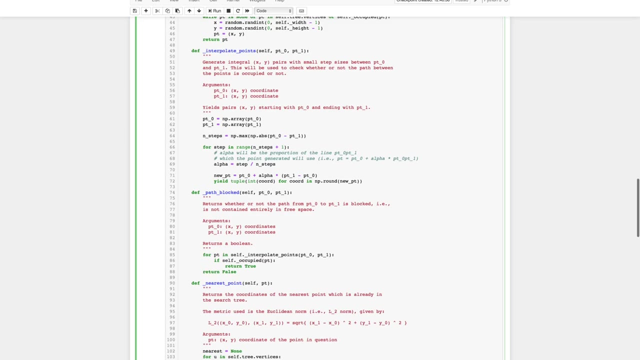 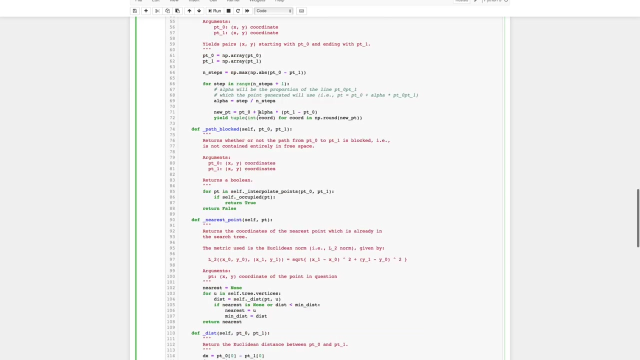 Well, we want to check whether or not the line from nearest to rand is contained in free space. Well, how are we going to do that? We can use this function here. Where is it? Path blocked, which I've written, So it takes two points. 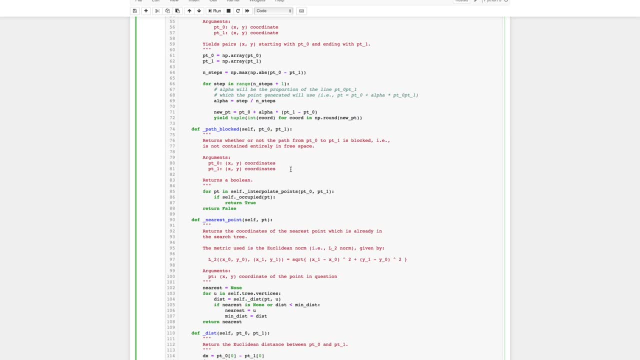 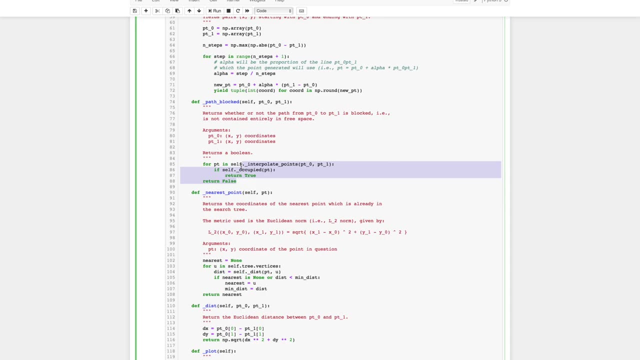 Point one, sorry, point zero and point one, And it's going to interpolate all of the points in our grid. So we've just got one point for each pixel And it's going to check whether or not they're occupied, whether or not that pixel is black in our image. 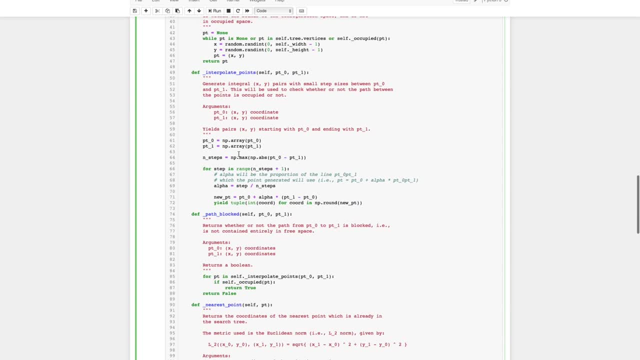 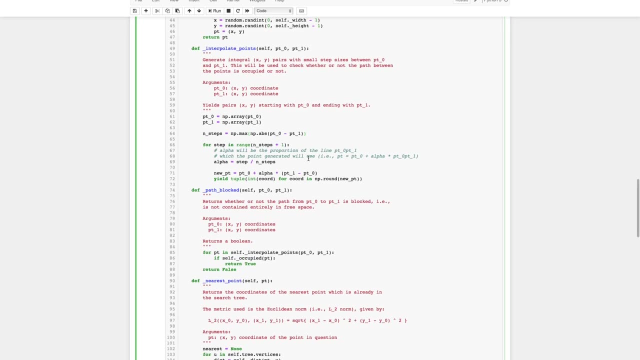 So interpolate points. how are we going to do that? Well, we're just going to figure out how far away these points are, Figure out how many steps we should do, And then we're just going to iteratively increase this percentage of the line segment from point zero to point one. 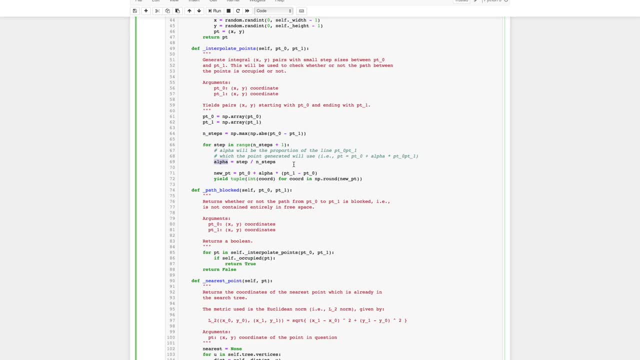 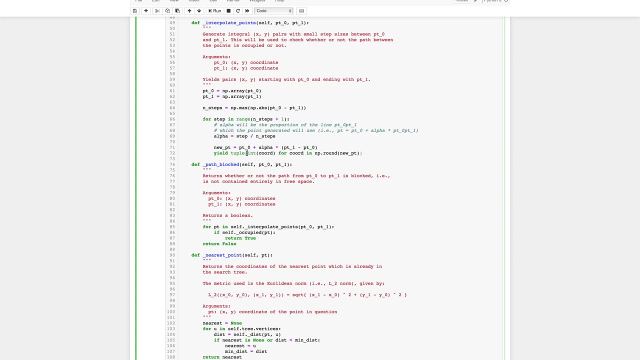 And return kind of the rounded coordinates of that so that we can access our pixels in the image. So by using int coord we're rounding these coordinates And then we need to yield to these as a tuple. So yield You might not have seen before. 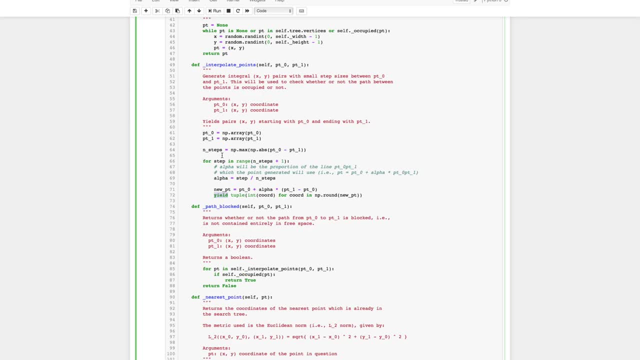 It's a Python generator, So this function will run And we can iterate over it just like a regular list or an iterable. But it's actually creating these points one by one. This just saves us some memory. We don't have to compute them all and then save them. 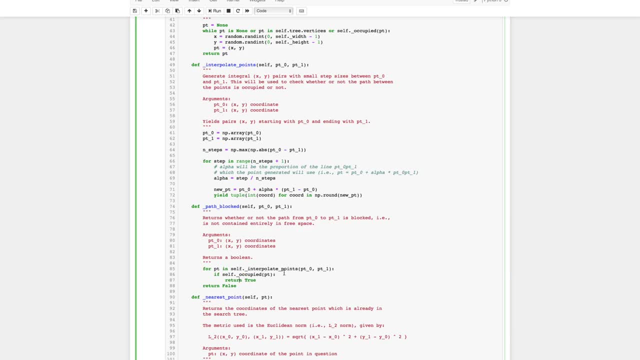 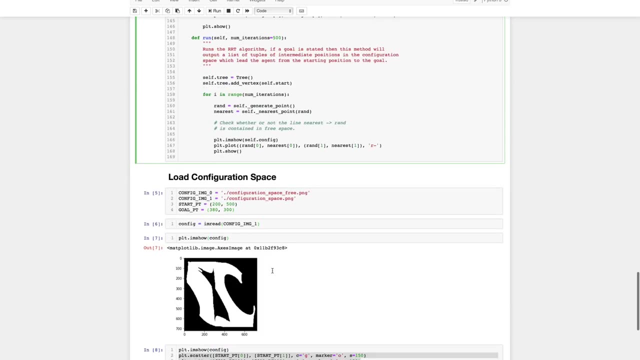 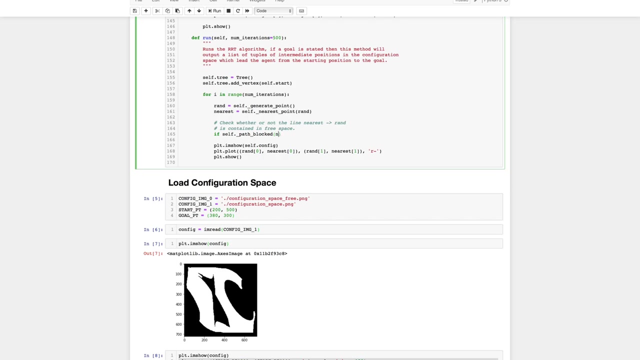 It also means that we won't compute all of them. if we find one that's in occupied space earlier on, We'll break out of the loop. OK, So let's call this function. So, if the path Is blocked from nearest to rand. 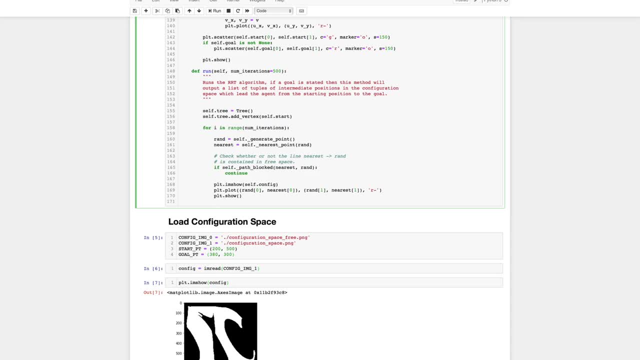 Let's just continue. Let's just discard that random point that we've generated and move on to the next one. However, what's the issue here? Well, now our i, the number of iterations we've done, doesn't necessarily match the number of vertices we've inserted into our tree. 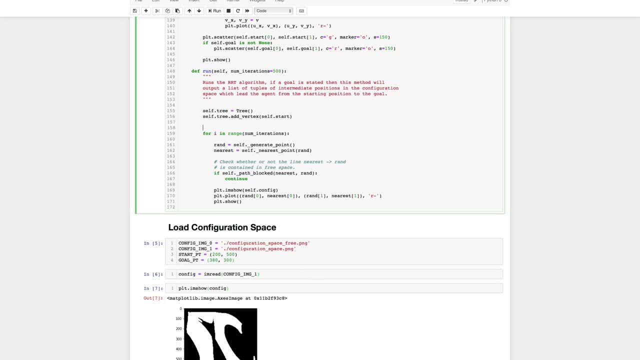 We'd like it to be the case that each iteration we insert one, exactly one vertex. So let's just keep track of i like this And increase it explicitly ourselves once we know that the path is not blocked. So if we do this again, 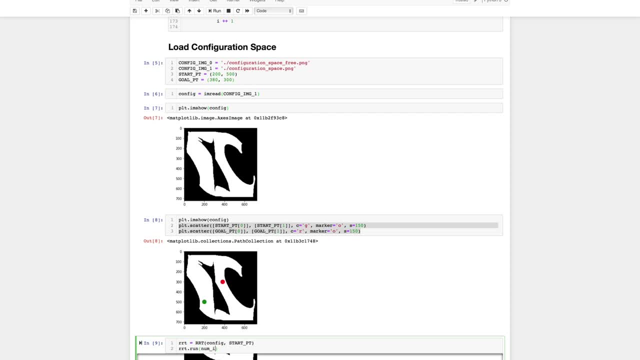 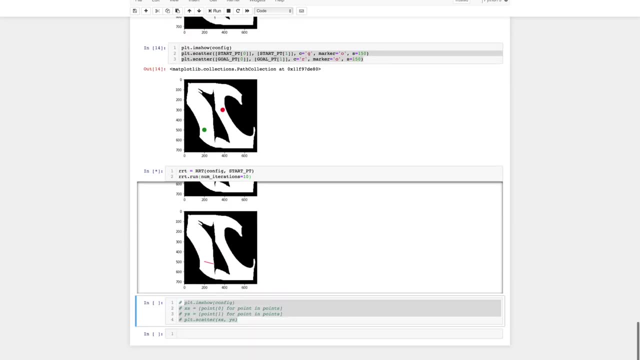 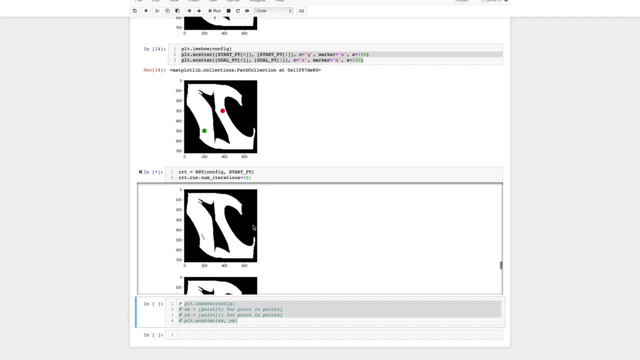 and I'm just going to bump down the number of iterations so that it runs quickly. We can see that we're only choosing points that don't go through occupied space. All right, It's doing a lot more than 10 iterations, unfortunately. 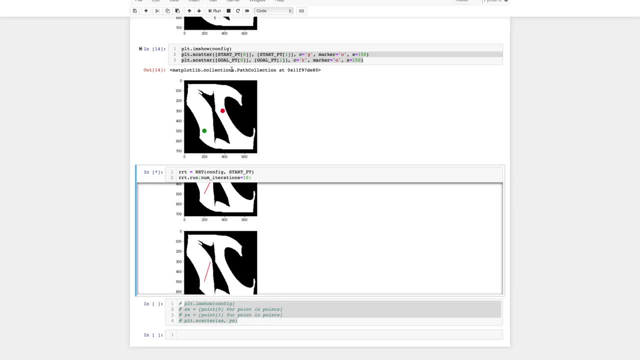 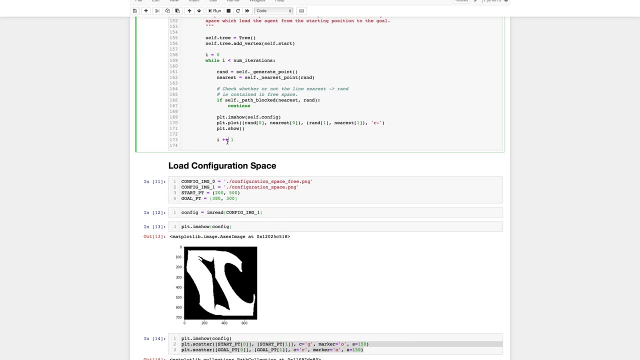 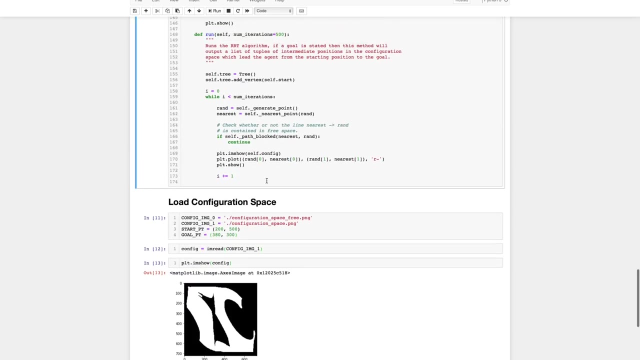 But that looks so good. So far, so good, All right. So Ah, there we go. There's my issue. That's why it's not counting the iterations. Let's make sure it stops that, Cool, OK, So we found a random point. 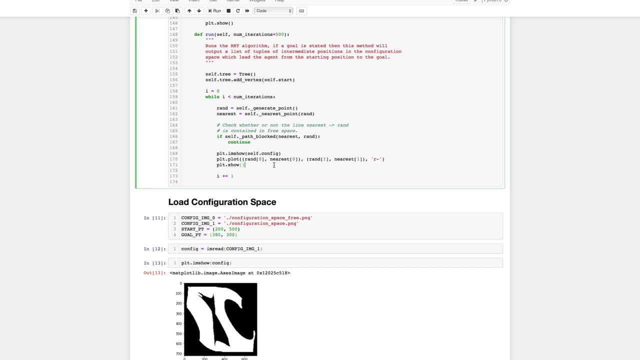 that we can add to the tree without moving through occupied space. So now what we need to do, looking back at the pseudocode, is we just have to add that vertex to the tree. So how are we going to do that? Well, self tree add vertex. 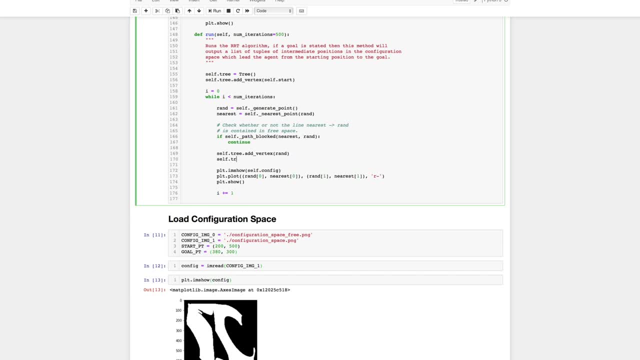 It's the random one, And we're going to add an edge from the nearest vertex, which is already in the tree, because we found the nearest point, which was already in the tree, and our random vertex. So what I'm going to do now is I want to plot this whole tree. 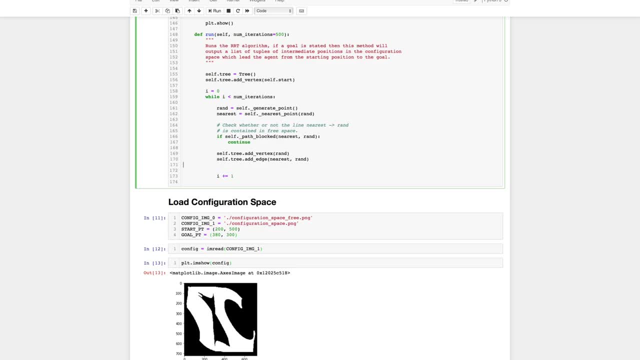 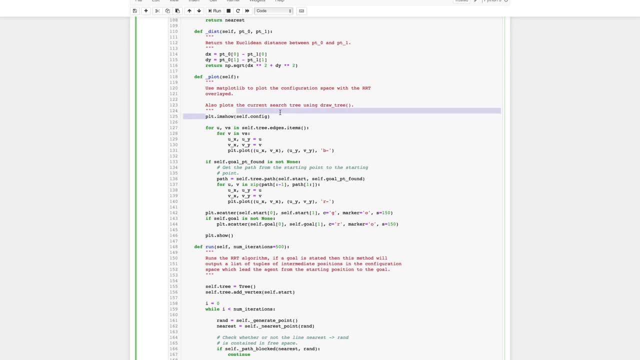 overlaid on the map. So rather than using these functions, here's something I've prepared earlier. This plot function does a similar thing. It just displays the configuration. It displays all of the edges in our tree. Don't worry about this bit yet. 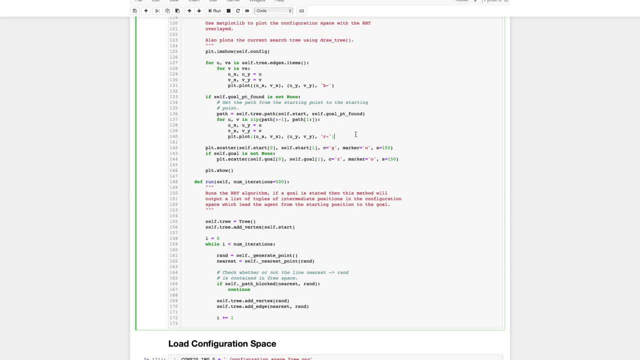 because we haven't actually found any goals or interpreted our search for a goal, And then it's also going to overlay the start and goal points as well. So let's just call that here Self plot, Once we bump up the number of iterations. 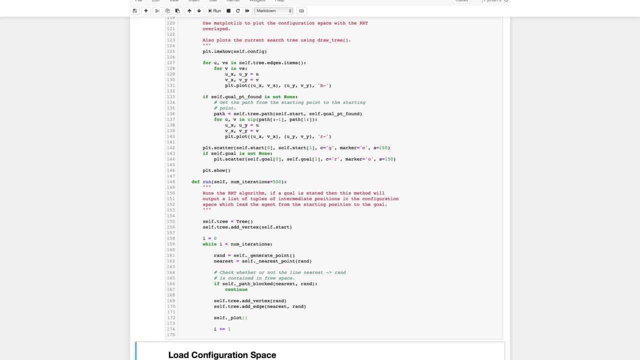 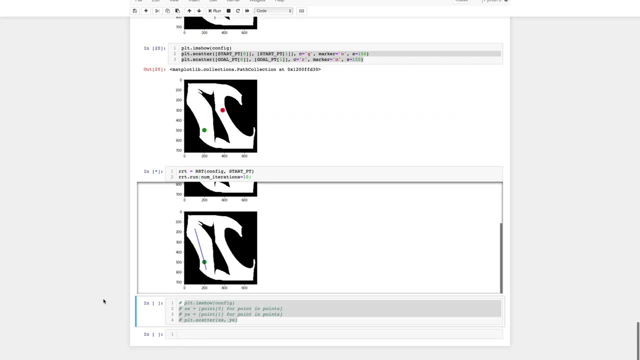 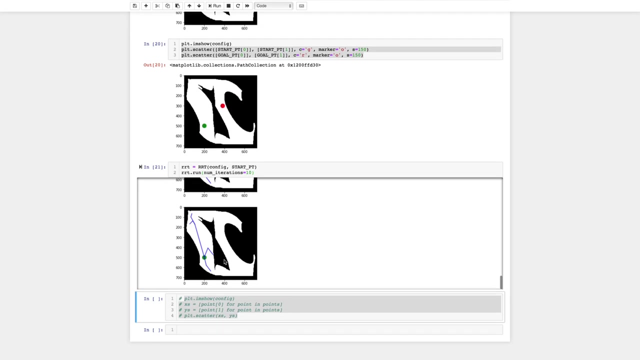 we probably won't want to plot this every time, because that's going to be a bottleneck in our algorithm. Cool, So we can see this tree is slowly building up. That was just 10 iterations. Let's bump it up to 50.. 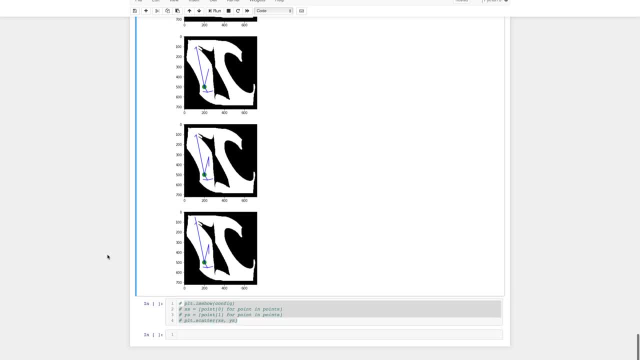 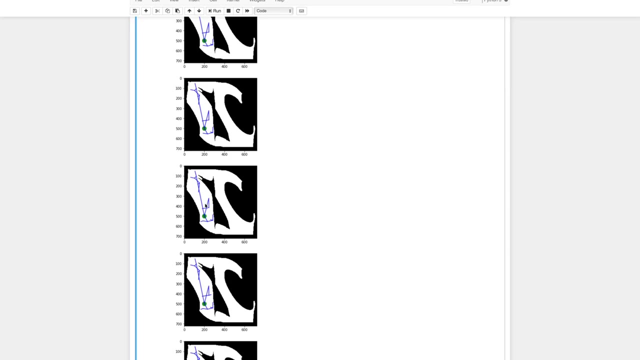 Looks pretty good. One of the things we'll notice is you can see that these edges are kind of doubling back on themselves, which kind of indicates that it's not necessarily the shortest path to that point from our goal, but it just is. from the points: 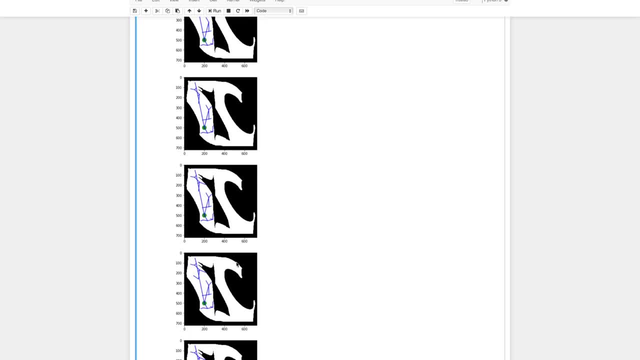 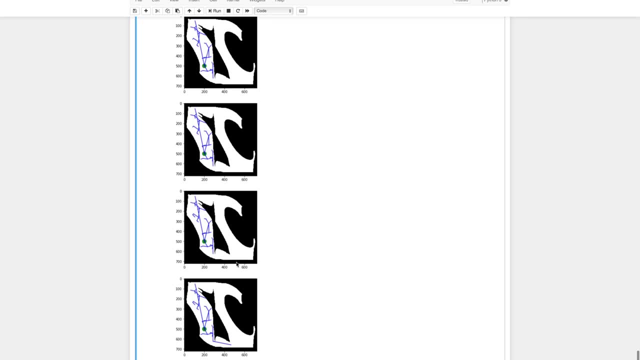 we had available in our tree. So we can talk at the end about some of the things we might want to do to rectify that issue. But at the moment it's kind of all right, We're filling out the tree, We're filling some space. 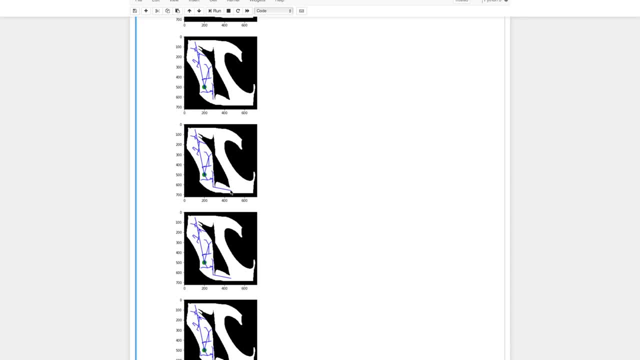 You can see that it's just started to turn the corner. It'll take a few iterations because it has to randomly get a point that's in free space and also be connected to something that's not blocked by an obstacle. So you can see now. 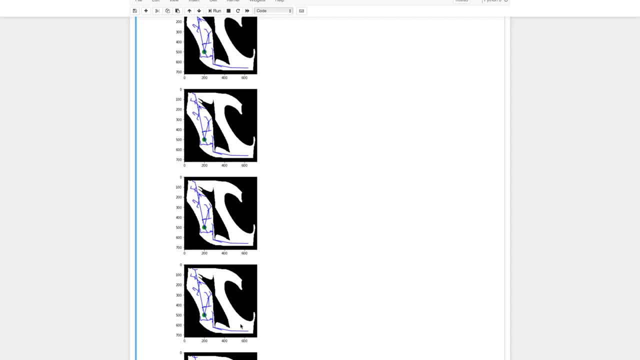 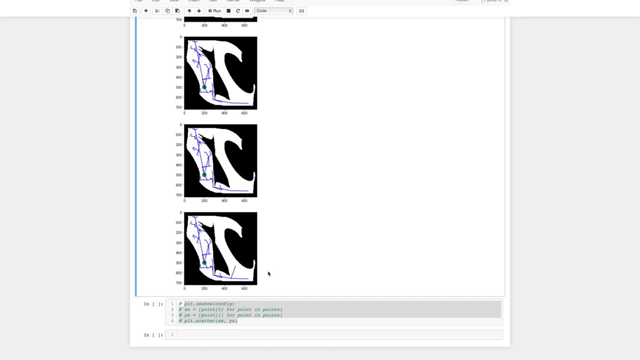 that we've got over to this spot, I imagine we'll start generating some points in this free space over here and adding the edges. You can see that started a little bit over there. All right, great, So it looks good, We're filling out this space. 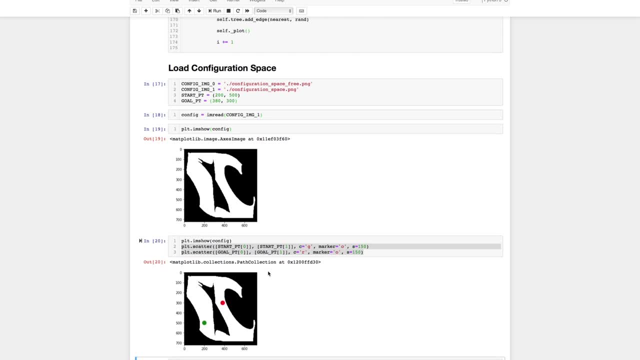 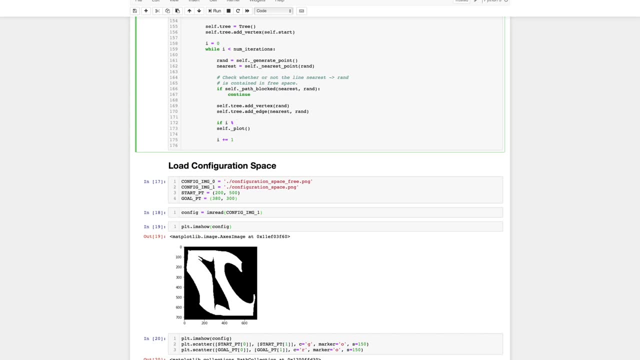 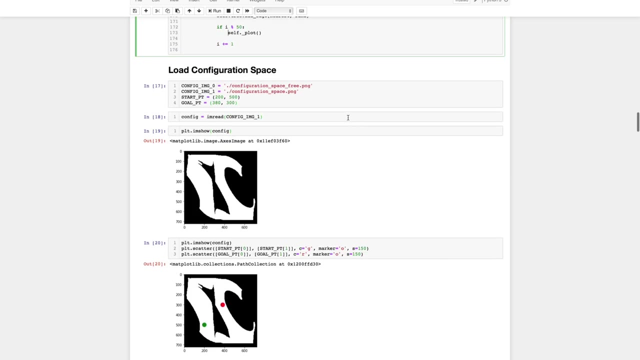 with our rapidly exploring random tree. Let's do just what I suggested before, And just for each iteration maybe let's say every 50 iterations. we'll plot it then. Then we should be able to bump up the number of iterations we're doing. 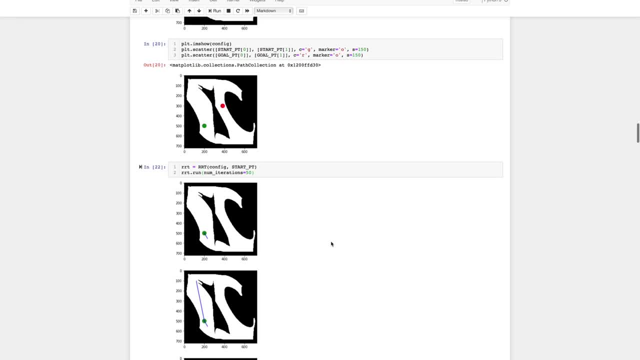 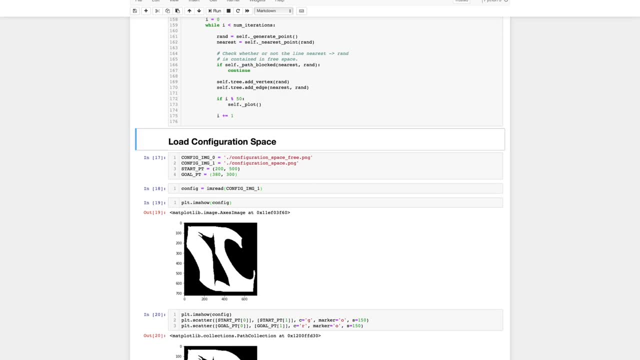 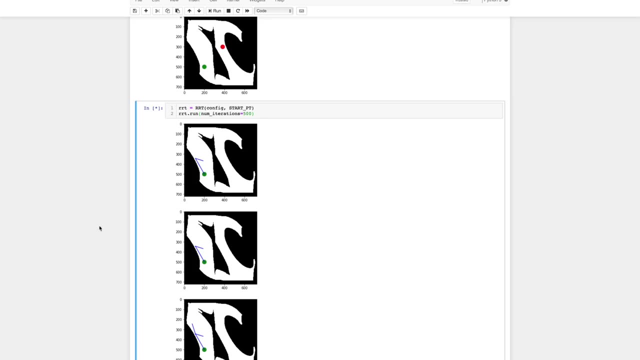 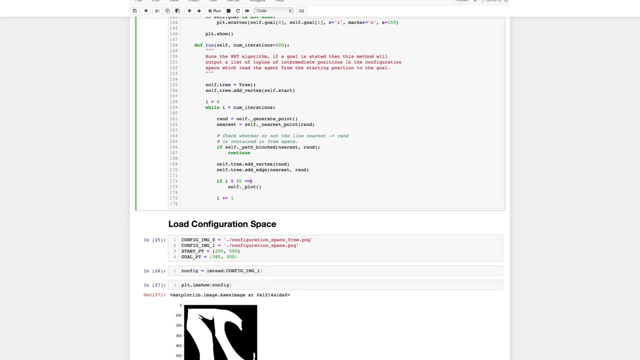 and see really how this tree grows. So let's bump up the iterations to 500, say: All right, this doesn't look too great because it's plotting it every time- Classic. I only want this to happen when it's zero. 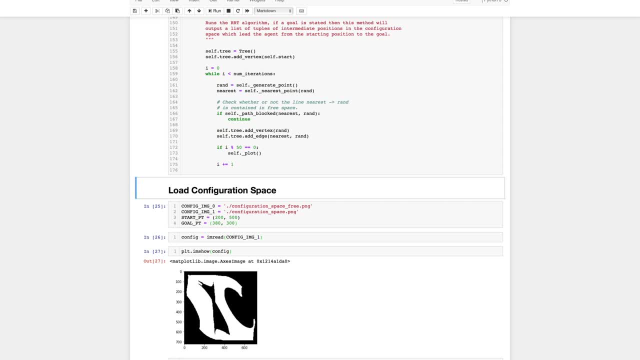 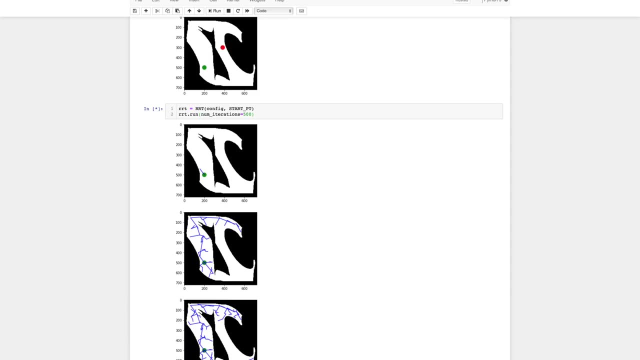 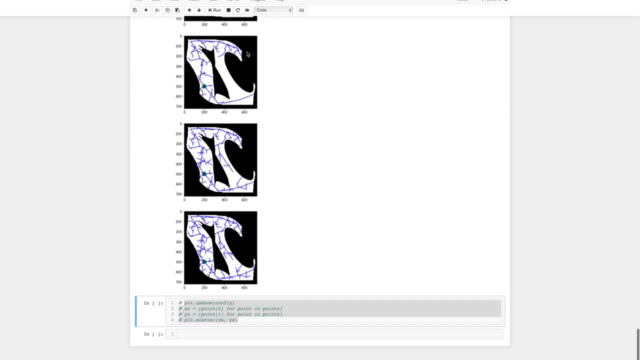 not when it's non-zero. All right, let's try that again. All right, so first iteration. that's 50th. iteration 100th Looks pretty good. You can see that we're filling the space and with our goal overlaid. 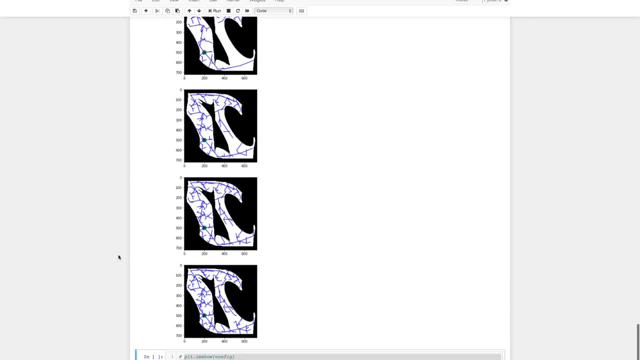 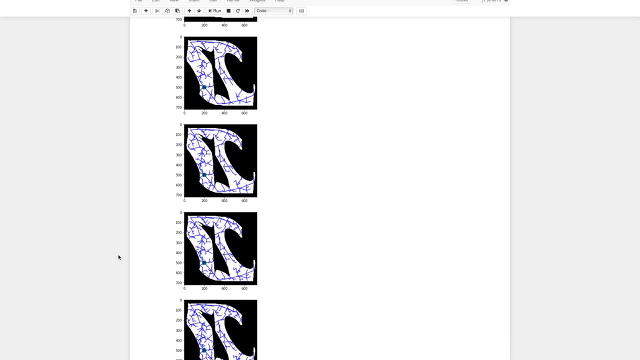 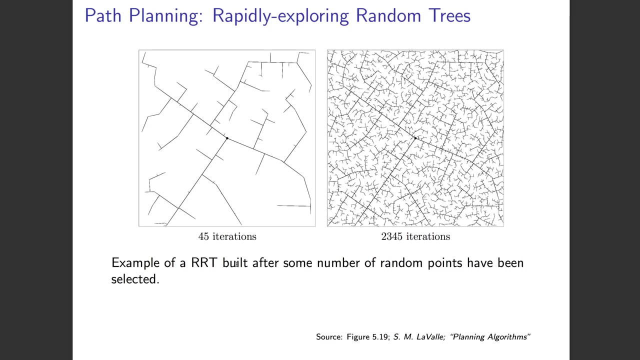 which was this point. here you can see that we're pretty close to actually finding that goal. I'll let this run into completion, just to see what's going on. All right, cool, Very good. That's looking something like this picture we had before. 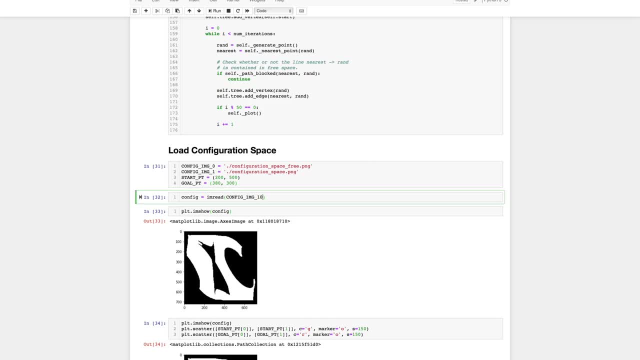 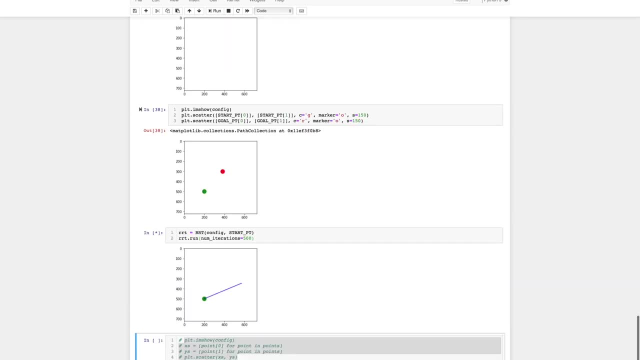 Let's have just as a comparison point. just have a look at what happens if we do this without any obstacles. It should still work, but we're just expecting it to be able to expand much faster because there's no obstacles in the way. 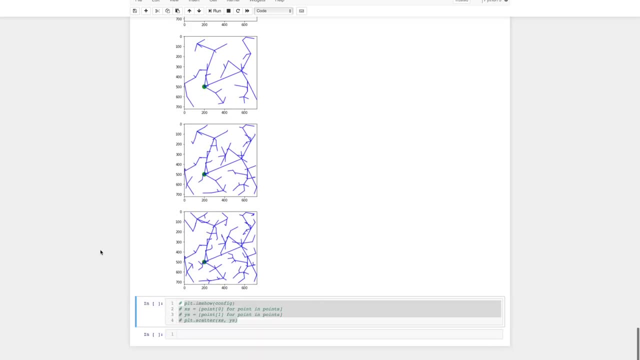 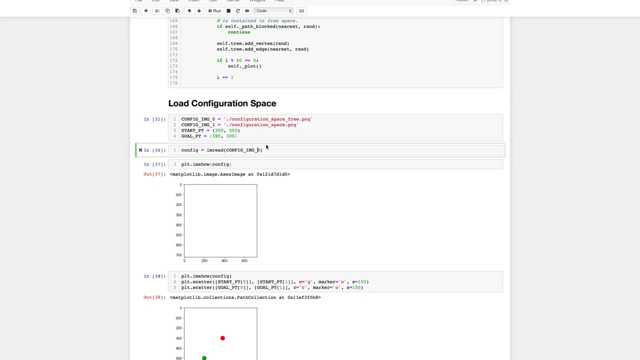 And we see exactly that happening. It gets to almost all the corners really quickly, within about 100 iterations or so, And then we just start filling out the space. So I'll stop that quickly. Great, So moving back to our configuration space with the obstacles. 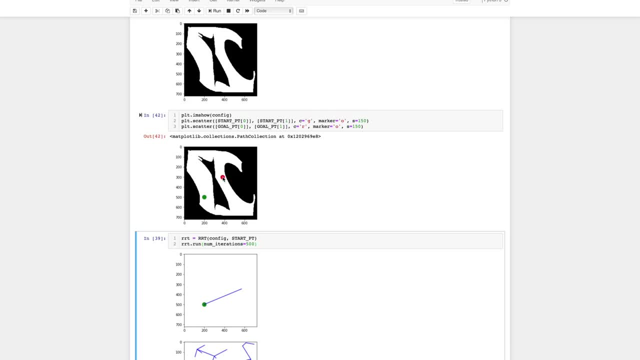 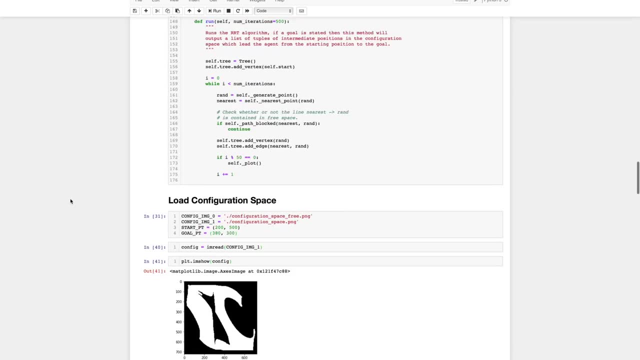 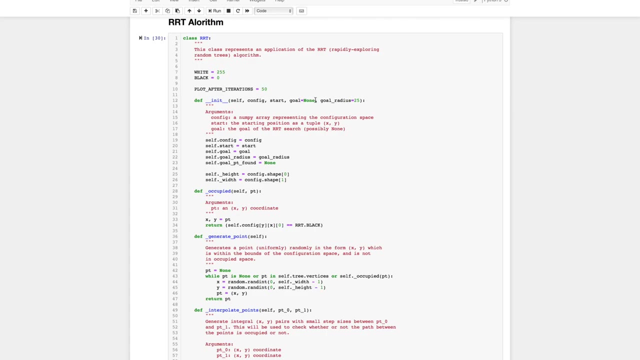 let's have a think about how we're going to incorporate this goal. So the first thing we're going to need to do is pass in the goal point to our algorithm. Up here we've got goal as an optional parameter to the algorithm. 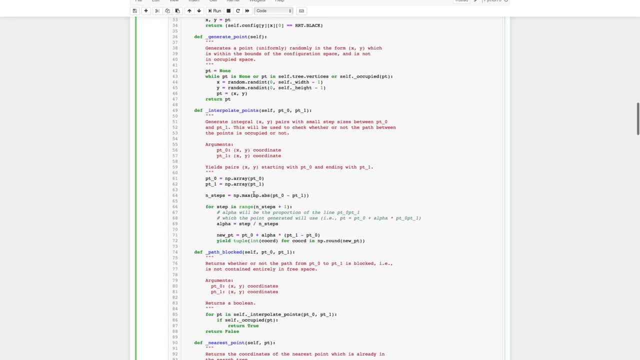 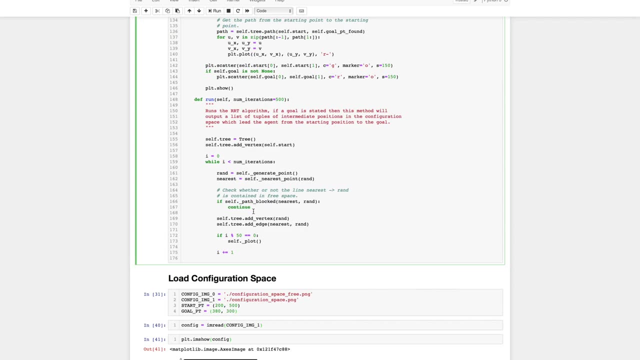 So if we specify the goal, this goal point will be not none. So then when we're searching, one of the things we want to do is check whether or not we found this goal. So maybe here we just say, oh, we still want to add it to the tree. 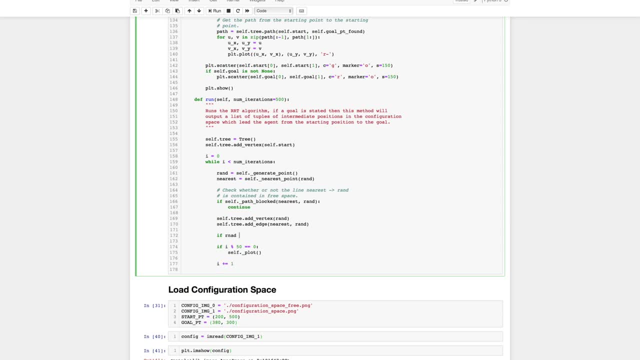 So we'll do it after we add it to the tree. But if rand is equal to the goal, then we want to break Once we're at the end. if we found our goal, we're going to want to, so if we found the goal. 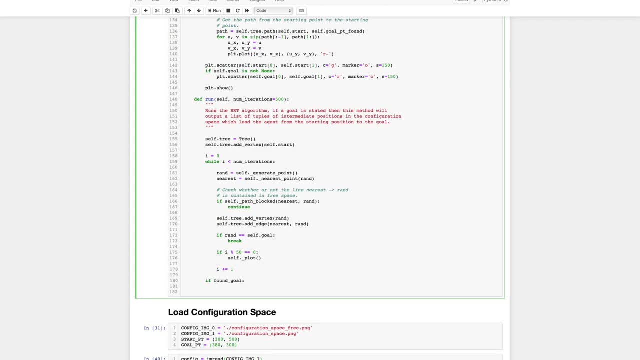 that's not a variable to see, but we'll define it in a second. So if we found our goal, then we want to return the path from the root to our goal. So remember that we had this path method in our tree And it's going to be between the start and the goal. 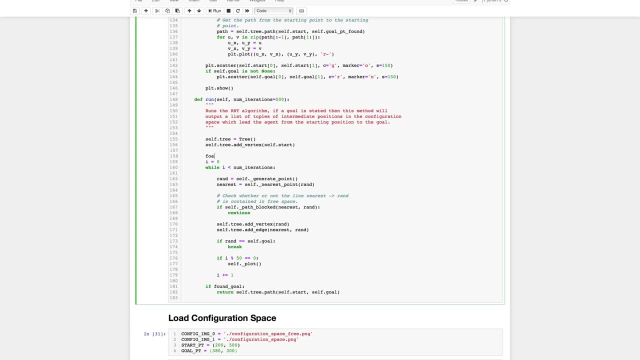 So what we can say is that we've found the goal. Initially we have not found the goal, so we'll set it to false. But once we do find the goal, we'll set it to true. So found goal equals true. 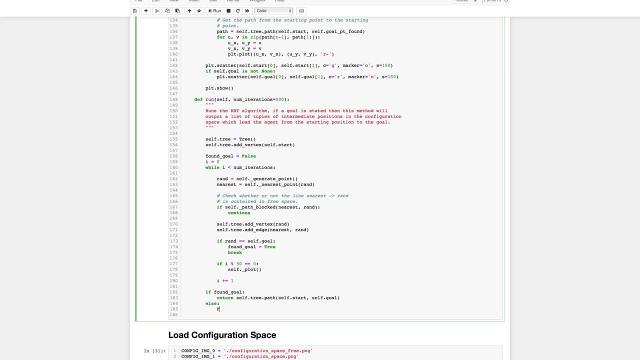 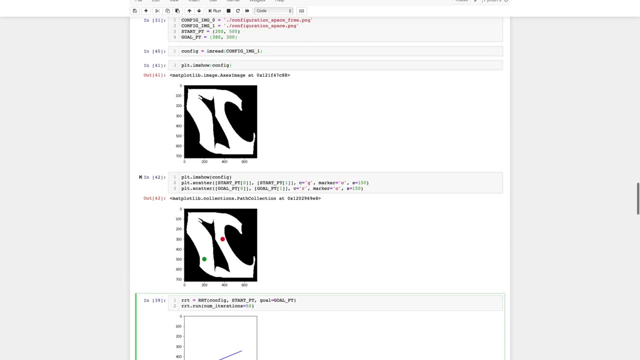 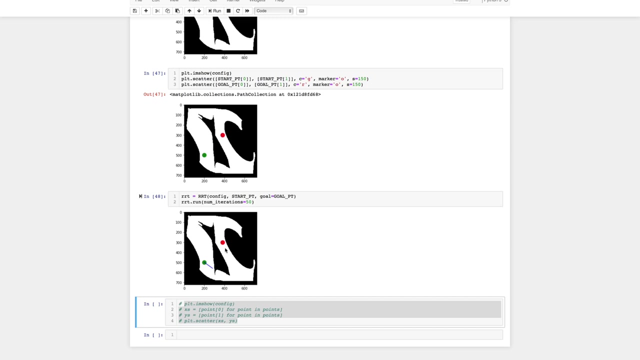 All right. So otherwise we'll return false. All right, So trying with a smaller number of iterations, first, just to make sure that nothing's broken. First of all, we say that we're now plotting this goal point, which looks good. 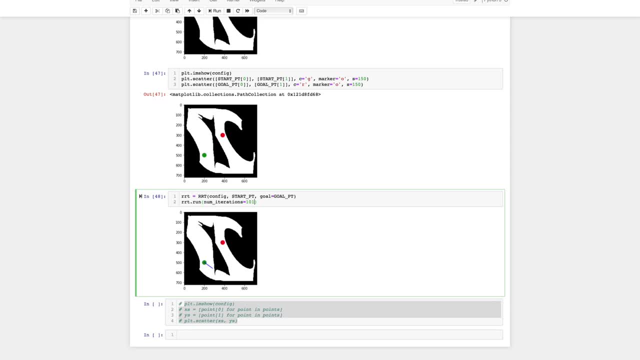 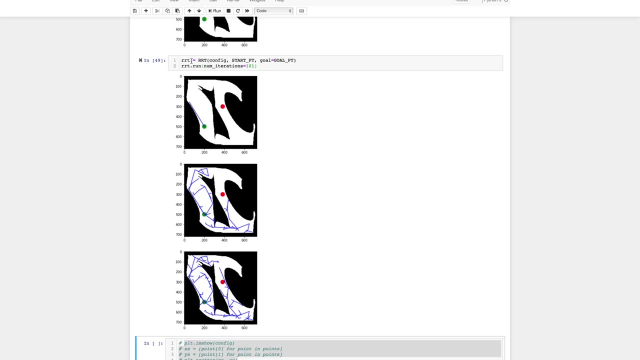 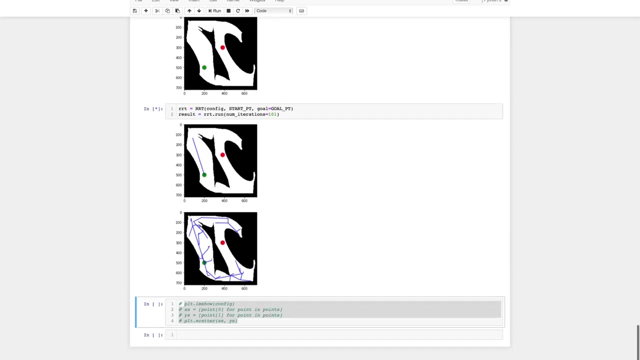 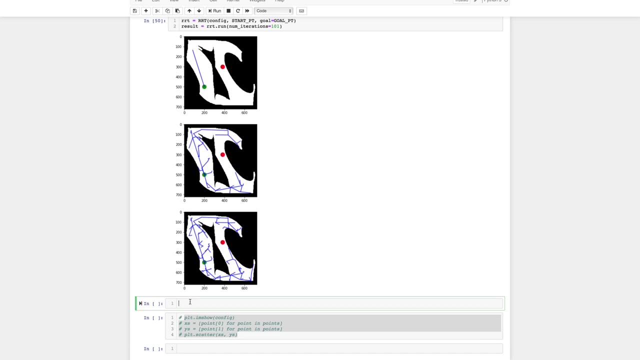 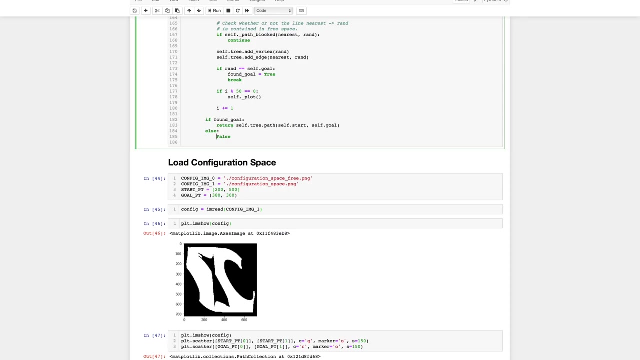 I'll go 101 iterations just so we get both those plots. All right. So what actually returned? Well, let's say the result is this: All right. Well, what's that result? Let's print it out: No Return false. 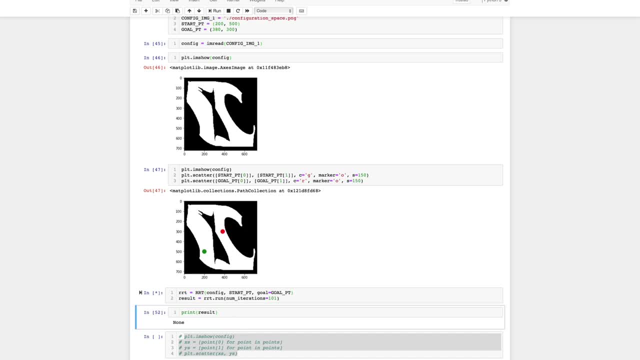 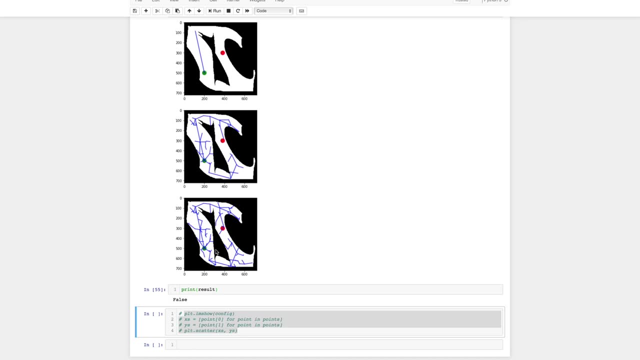 My bad, All right. So it's still saying that we didn't find the path, but we got pretty close to our goal, So what might be going on there? Well, at the moment we're expecting to find our goal, exactly right. 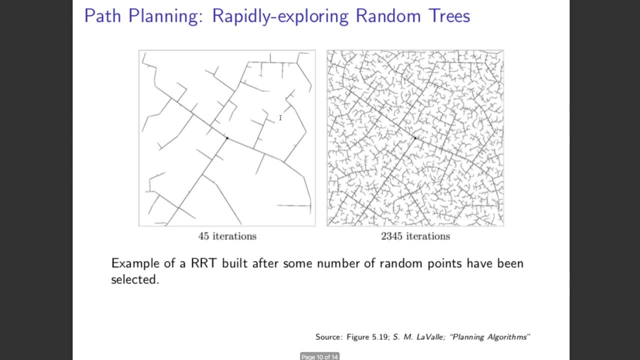 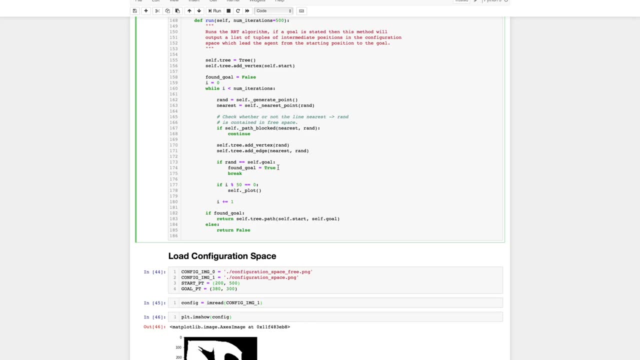 Which we spoke about before. since this is a space-filling tree and it is eventually dense, we will eventually find every point, But it might take a long, long time. So one of the things we could do is we could think: all right, well. 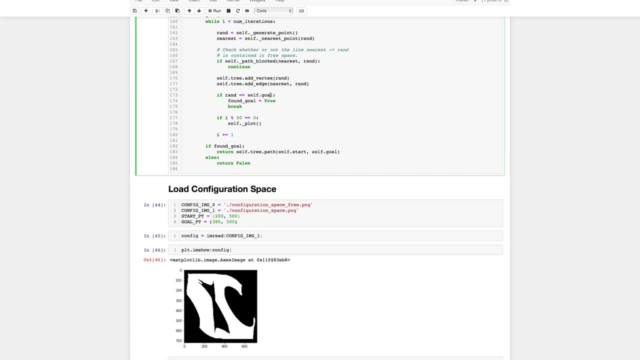 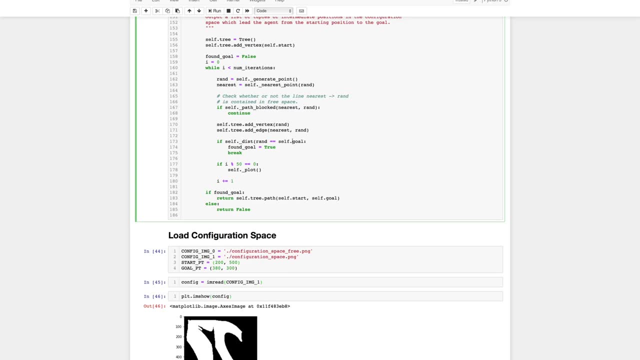 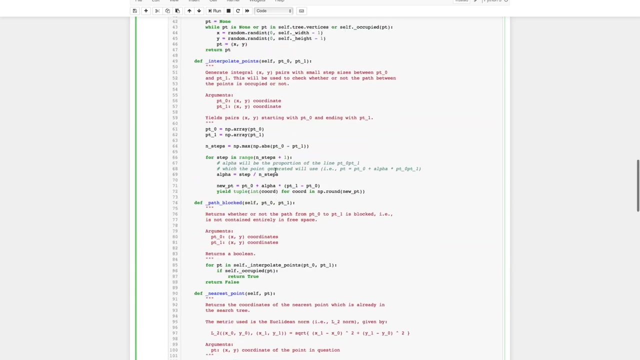 how close is close enough to our goal. So rather than checking if our random point is exactly our goal, maybe we want to check that the distance between them is smaller than some radius. So I've already defined this goal radius here. We've set it to 25 pixels initially. 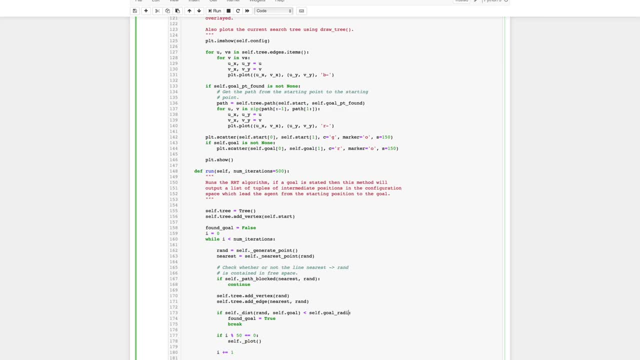 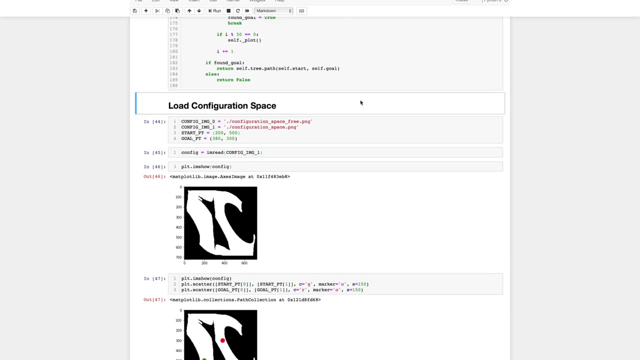 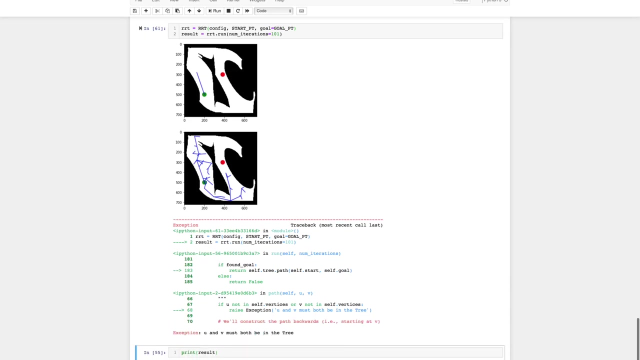 Let's stick with that, All right. Now let's try this. All right. So it looks like we found the goal, but we've got this exception: u and v must both be in the tree. So we've tried to find the path. 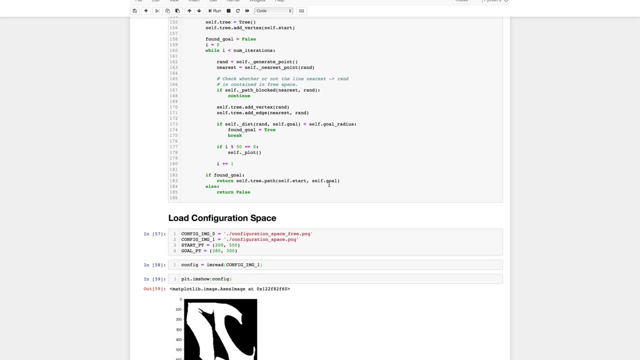 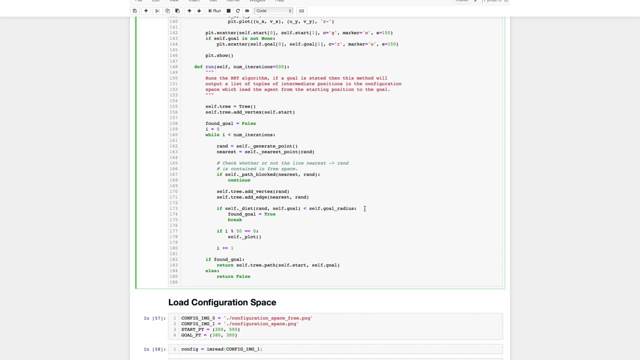 Between the start and the goal, But the goal exactly isn't in the tree. So we're going to have to keep track of, kind of the closest point we found. So we're just going to say that once we found the goal, we found some point which was close enough to our goal. 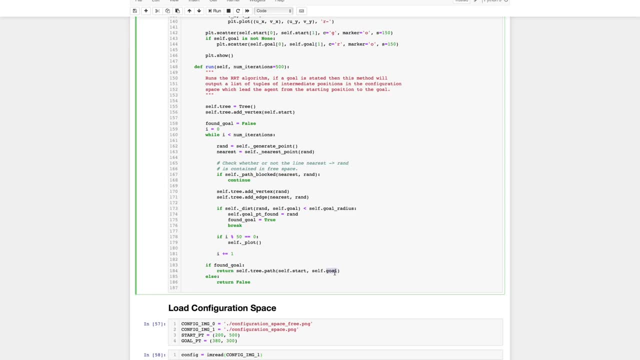 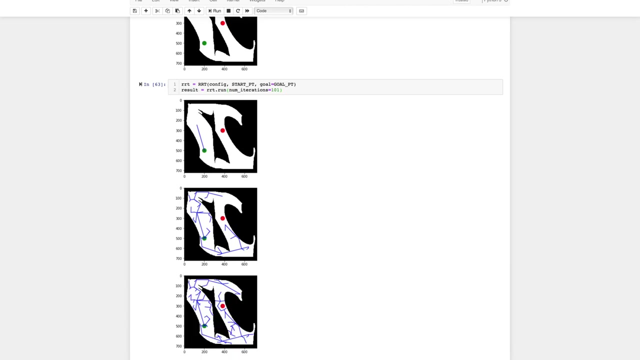 Set that to random And then here, rather than finding the path between the start and the goal exactly, we'll just start to find the path between the start and the goal point found. Let's have a look and see if that fixes our issue. 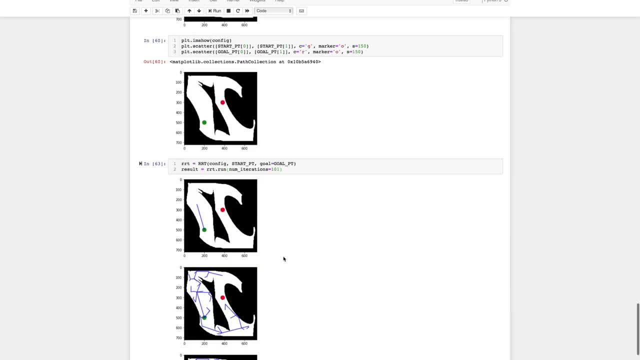 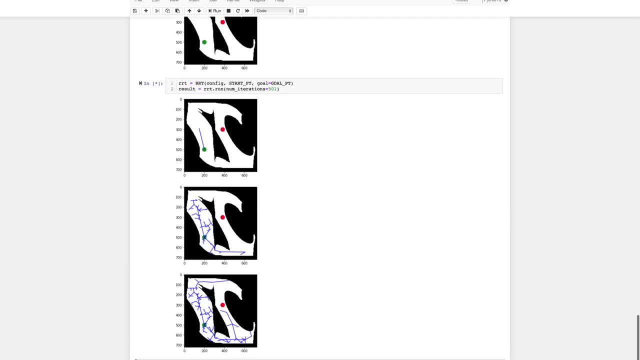 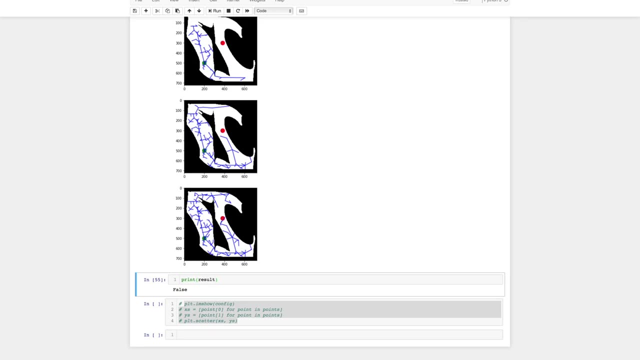 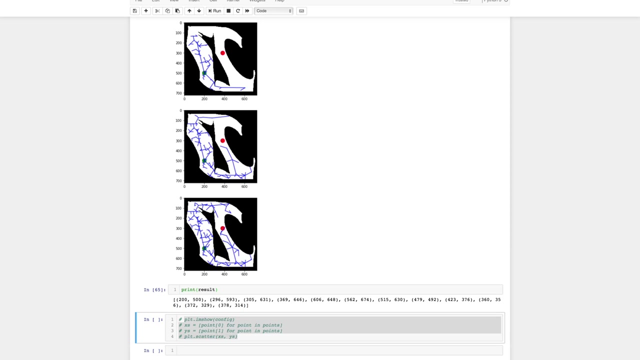 All right, We got pretty unlucky there. We skipped right past it, So let's bump up the number of iterations. All right, That looks like it stopped, Cool. So the result is this path: It's a sequence of states that we can move between linearly. 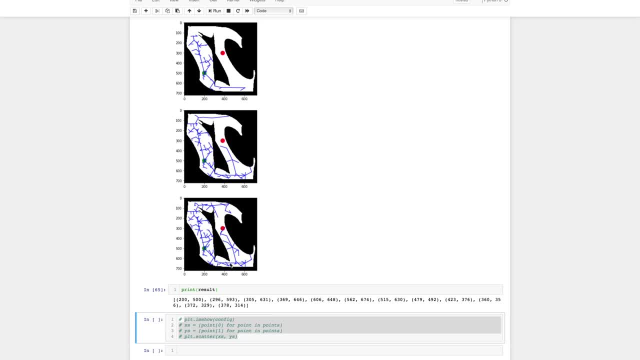 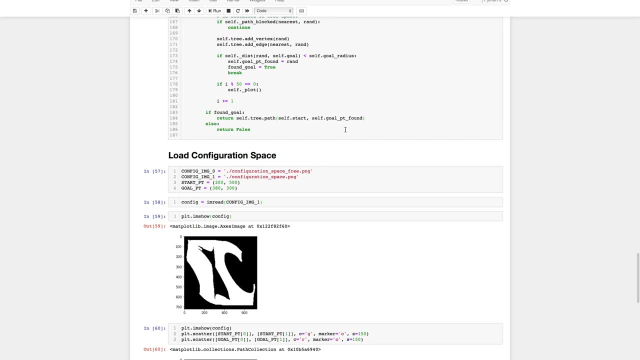 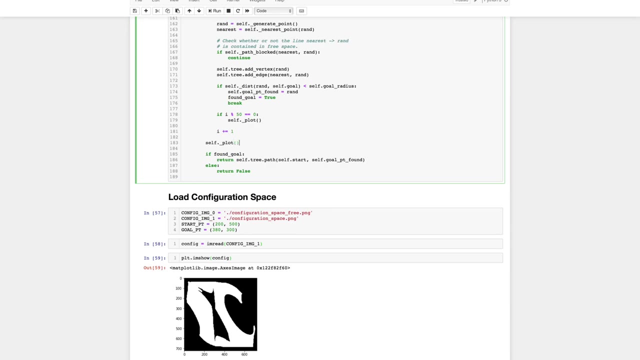 And we will get from our initial point to our goal. Let's have a think about whether we can plot this. Maybe at the end we'll just call this self plot function again And we'll see that in this plot function we've checked whether or not we found this goal point. 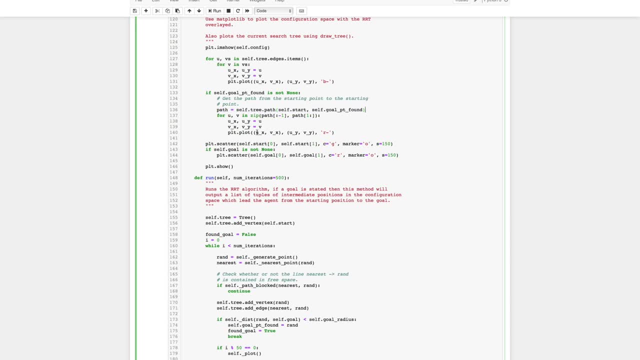 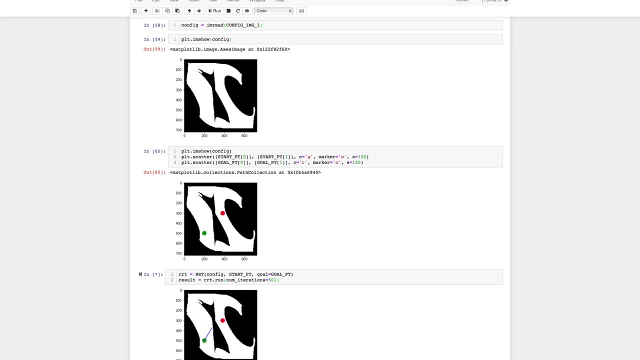 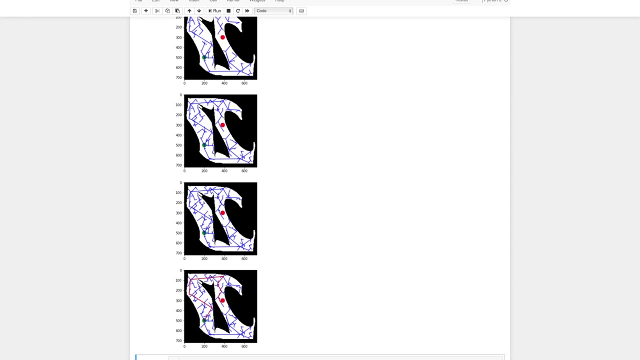 And if we have, then we're going to find the path And we're just going to draw that path in red. So let's try again. All right, So still getting pretty unlucky? Ah, cool, So we've found a random point. 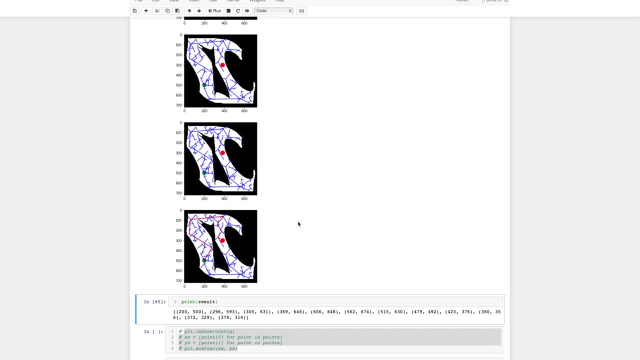 which is close enough, And we found this red path. Let's print out what that path is. Looks great. So I mean, what are some of the issues here? Well, it's a pretty silly path to take to go all the way over there. 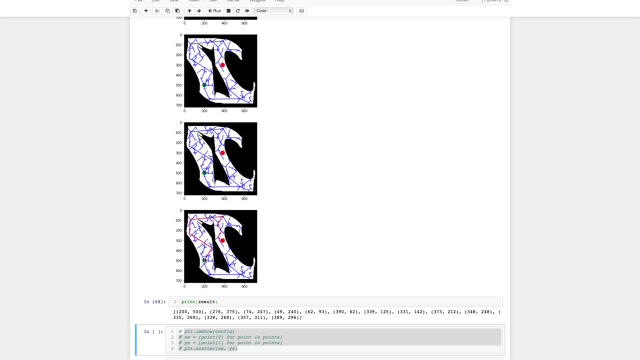 all the way over there, all the way up, But we could have just got to that point directly. So maybe one of the things we could do is we could see if we could smooth out this path. Maybe we can see if there's any vertices which can be avoided. 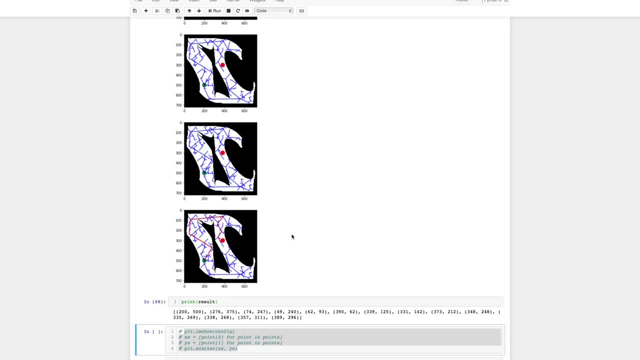 and get straight to the end point. I'm just thinking whether or not I've got time to go over that now. Perhaps what we can do is we could just check for each vertex in the path whether or not that vertex in the path can be removed. 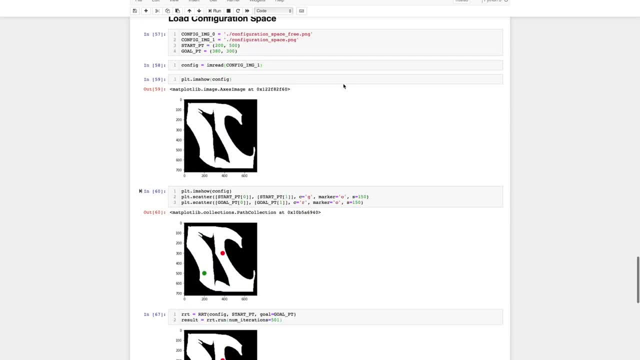 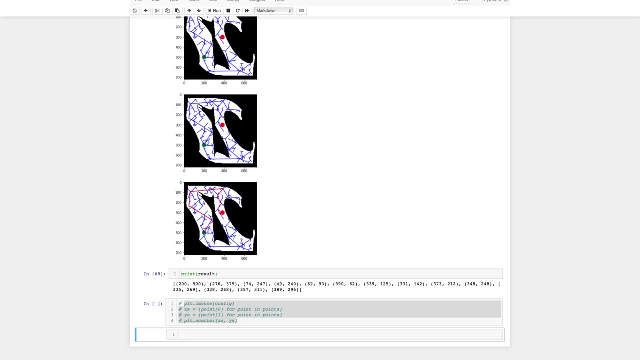 So what we would do, I guess just in terms of some pseudocode, it'll be: for each vertex, see how far in the path it can go without hitting an obstacle. Then we want to remove intermediate vertices which are not needed. 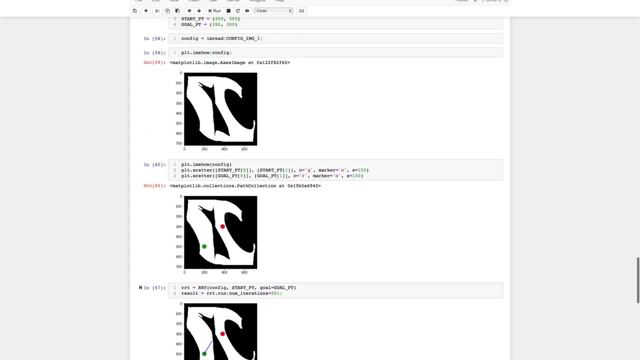 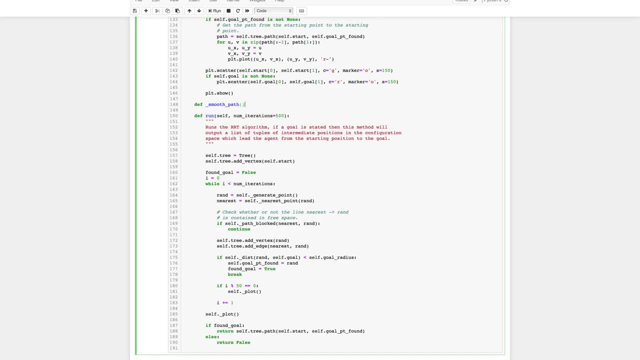 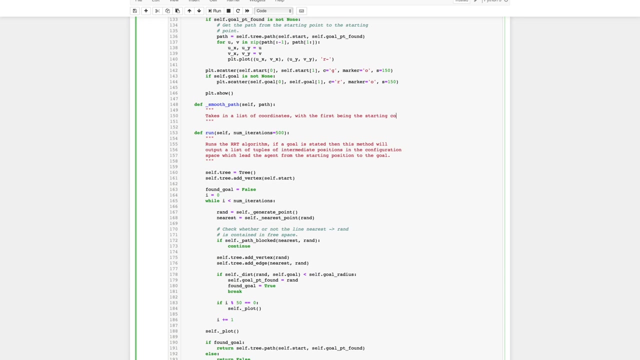 All right, let's have a think about that. So let's write this function, smoothPath. It's going to take in a list of coordinates, with the first being the starting configuration and the last being the goal point our algorithm has found. 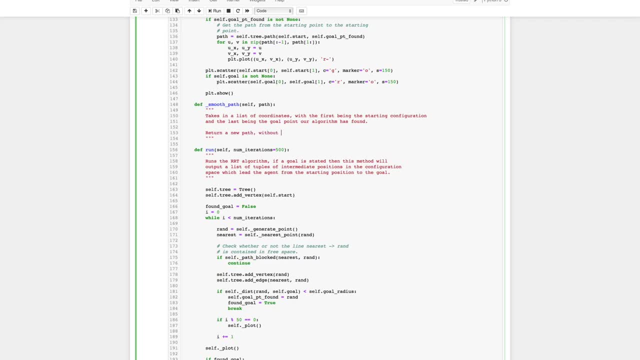 It's going to return a new path without unnecessary intermediate vertices. Cool. So rather than deleting from our path, we'll build up a new path. So for each vertex in the path actually, rather than each vertex in the path, we'll just add them incrementally to this new path. 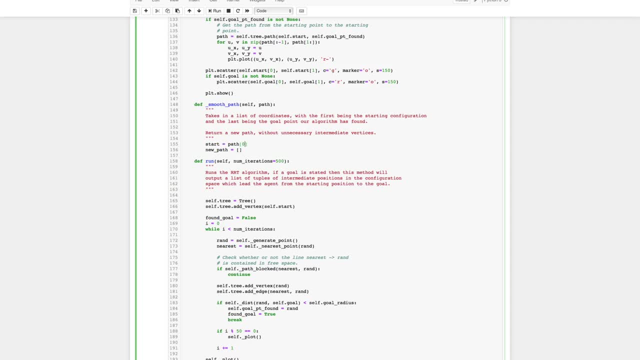 So the start is going to be the first coordinate in the path and we'll just include that in our new path because we better have the starting position in our new path. Let's also keep track of the goal, which is that last element. 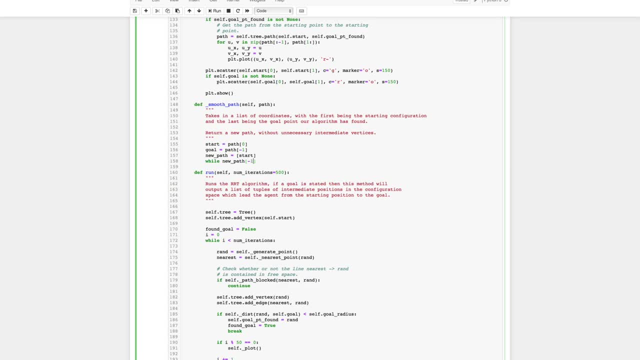 So while the path has not ended, ie while our new path doesn't contain the goal, at the end we're going to take the last point that we've got to And then we're going to search through our original path to find. 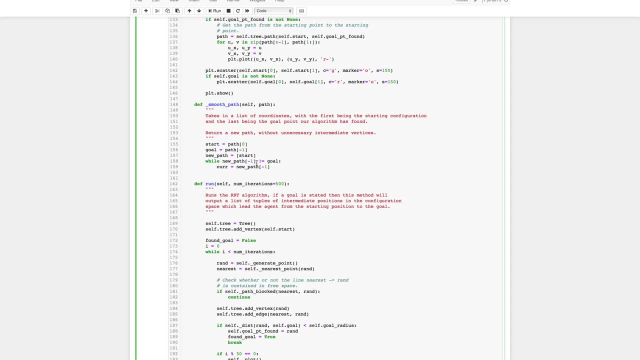 the furthest away vertex which doesn't have its path blocked. So we're going to need to keep track of the indices. So the first index is 0. And the current index is going to be the new path index- that last element. 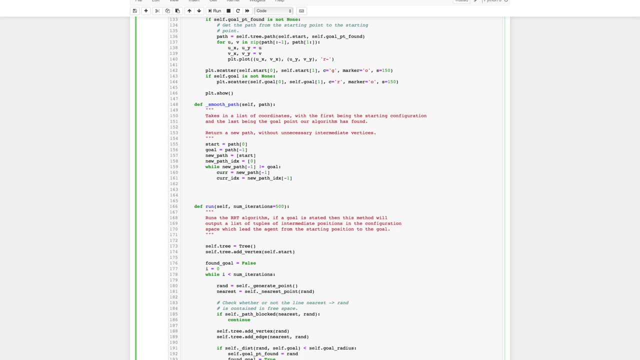 So now we're going to- I'm just going to say wild truth now, because I'm not sure what the guard is going to be at the moment, but I'll come back to that in a second- What we're going to do. 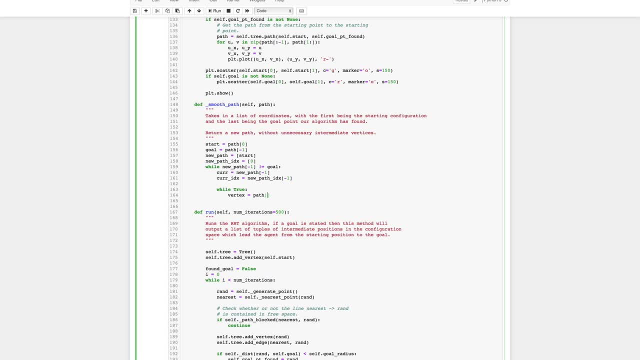 is we're going to look at the next vertex. I guess we want to say we'll keep track of this vertex index And we'll check whether or not the path is blocked. So I mean what we want to do is we want to. 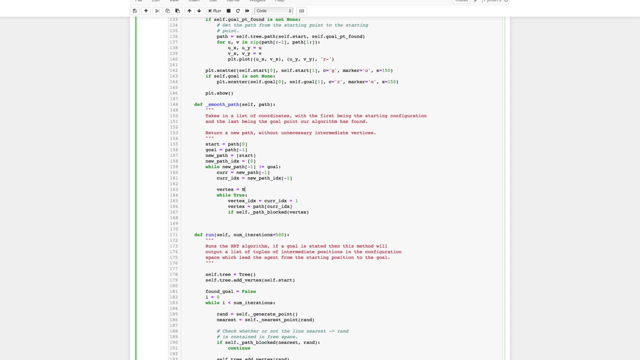 pick up what the vertex is going to be. So we'll just say it's none at the moment, And then these are the candidate vertices that we will use in this smooth path. So we're going to say, if the path is blocked between 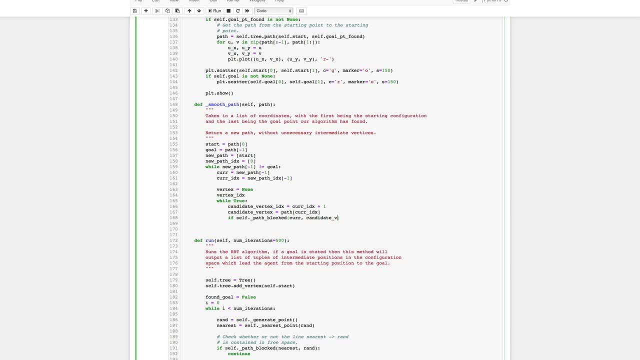 our current vertex and our candidate vertex, then we're going to break. So we've found a vertex which there isn't a path from the current vertex. we're looking at to it, Since we know we've already got a path of vertices which do have. 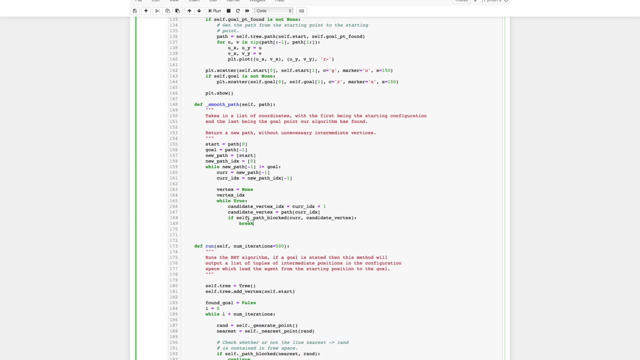 jumps which are entirely contained in free space. this vertex will not ever be none. We always know that at least the next one is going to be able to be reached from the current vertex. So now we can have a think about what this for loop is going to be. 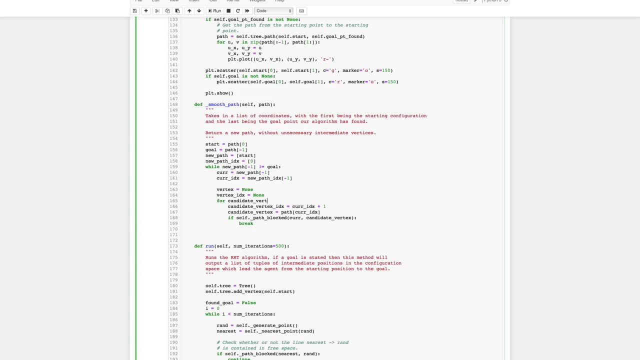 Let's actually say for candidate vertex, index and candidate vertex- and enumerate. Well, we want to go from the current index. Sorry, this was wrong, This should have been current index plus one. But we want to enumerate this path from the current index. 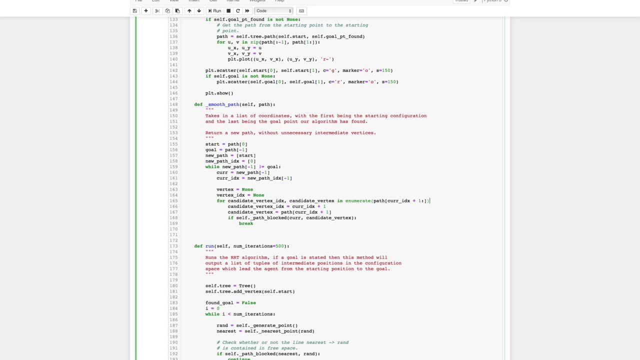 I think we probably want to enumerate it from the next one as well. So if the path is blocked, then we want to break. Otherwise, we're going to update the current vertex we're looking at- Well, I mean the current best vertex we have. 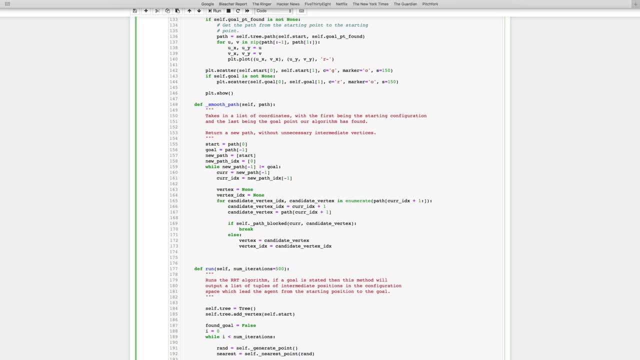 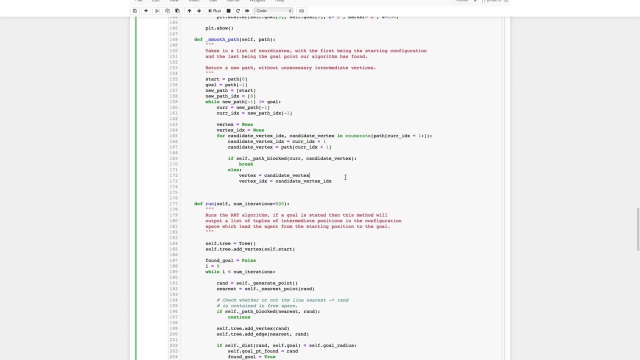 Okay, So let's see whether or not this works. So the first thing we need to do is now we need to add this new vertex to the new path, And we also want to keep track of its index Vertex index. So 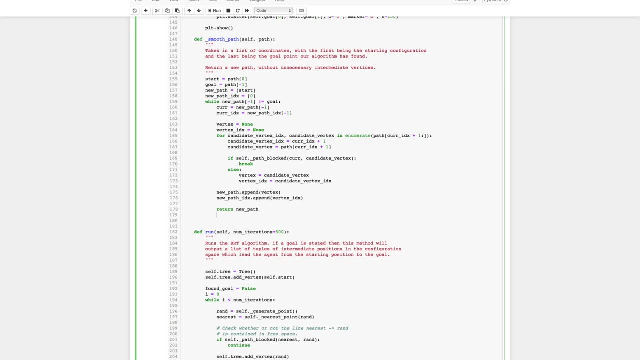 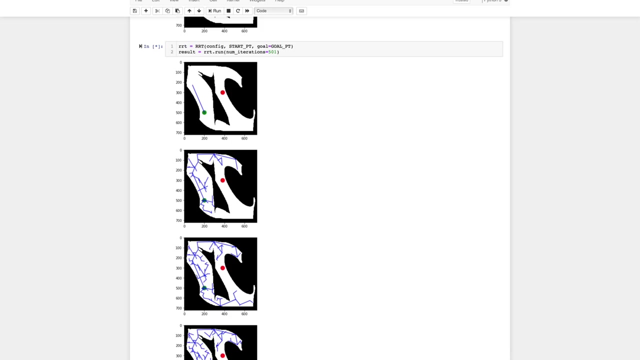 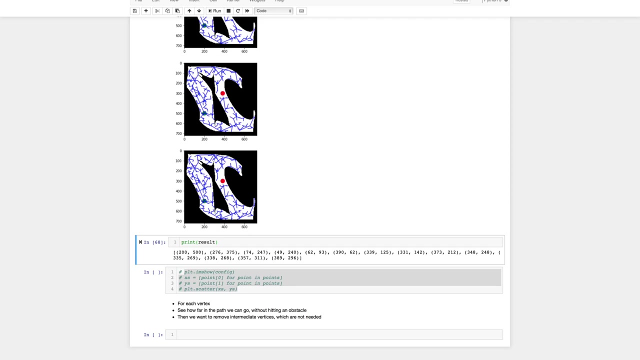 let's return this new path, Alright, So excuse my lack of commenting. Let's see whether or not this works for this path we've found down below, So we'll find a path. Come on, Maybe we're going to get unlucky and not find it. 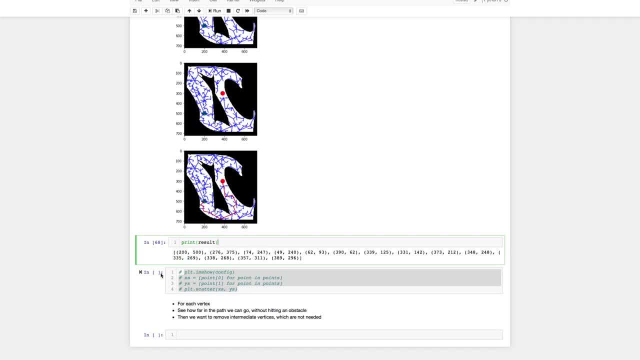 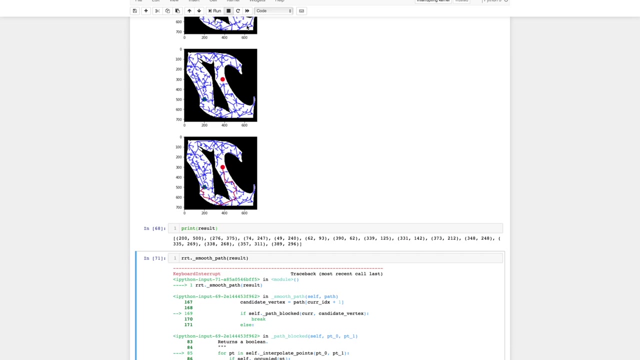 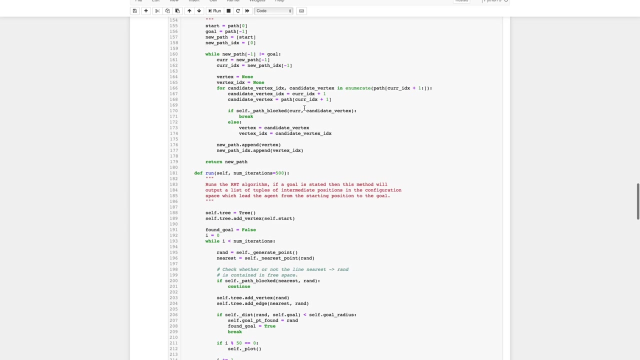 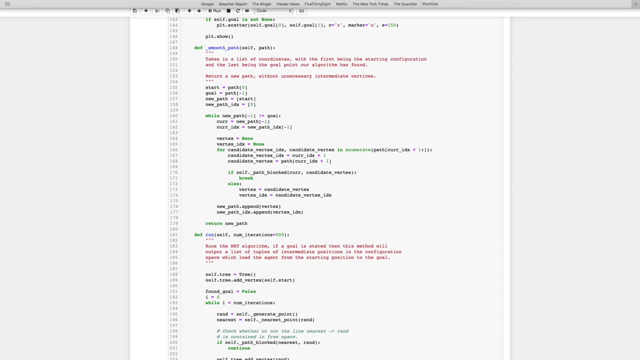 Ah no, There we go, We've found a path, So that's our result. And then we want to say, well, let's smooth the path. Not looking good so far. I imagine we might have got stuck in an infinite loop. 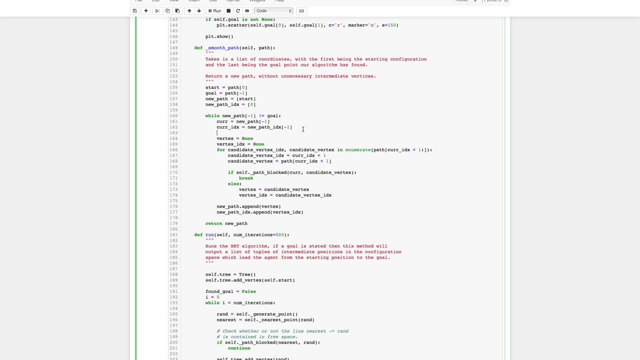 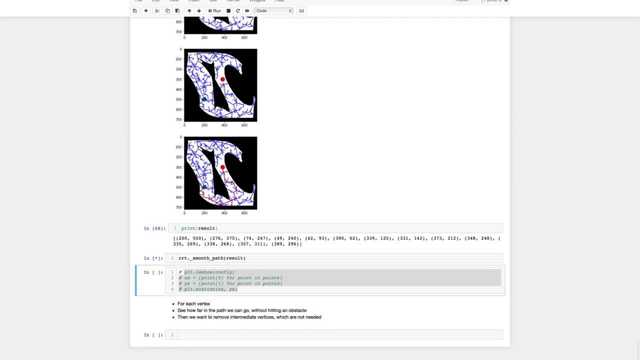 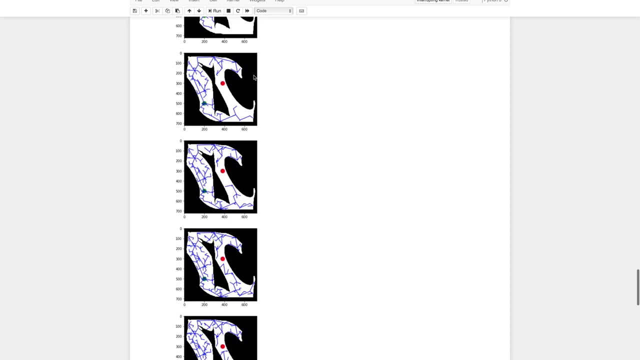 Okay, So why might this be the case? Let's just print out what our new path is, Well, what the indices are at each point, And figure out why this might be getting stuck. I guess I need to run this again. 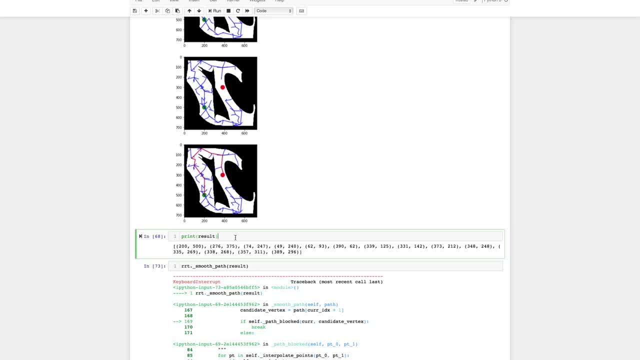 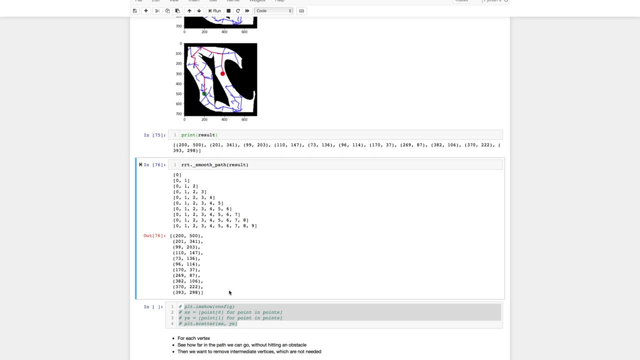 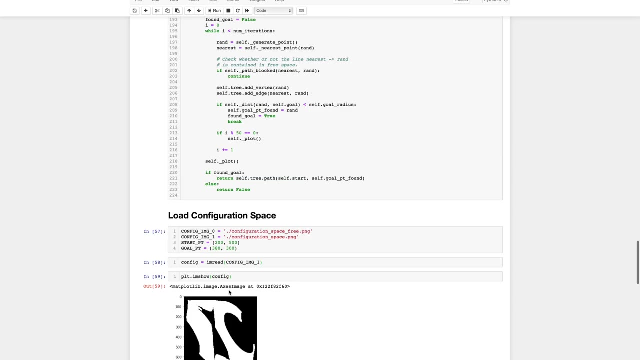 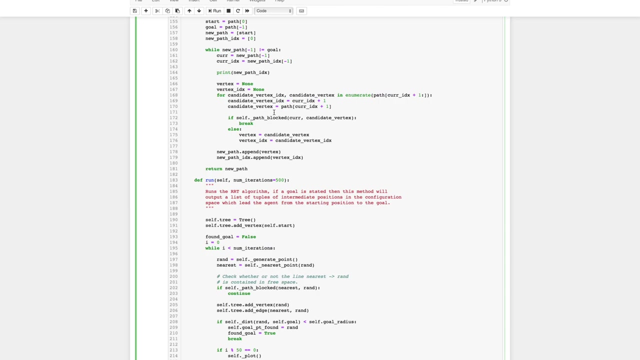 Alright, So we've found a path. Let's print out that result. Alright, That works well. that time. actually, Unfortunately, we haven't smoothed out the path at all, So what are we doing? Let's just see when this is being blocked. 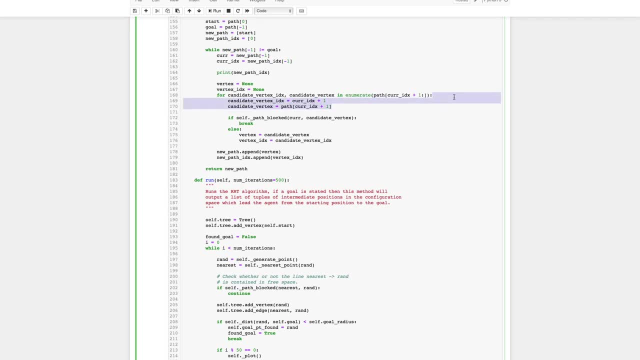 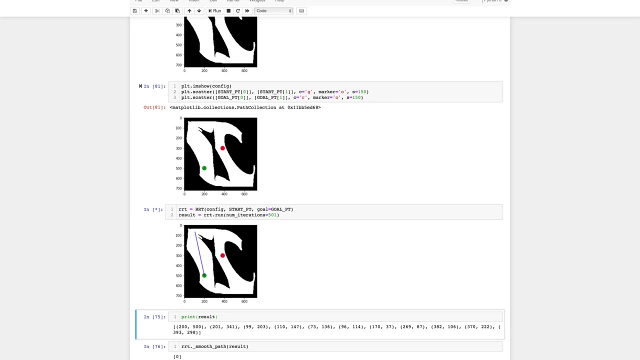 Alright, So I'm overwriting these during the for loop. That was silly of me, My apologies. Let's see how we go this time. Okay, So here we go. So we're trying to find a path, Okay. 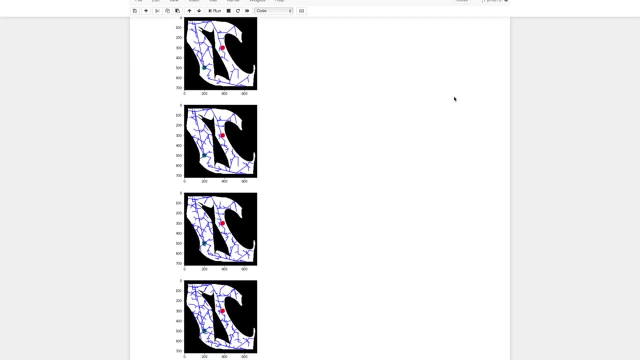 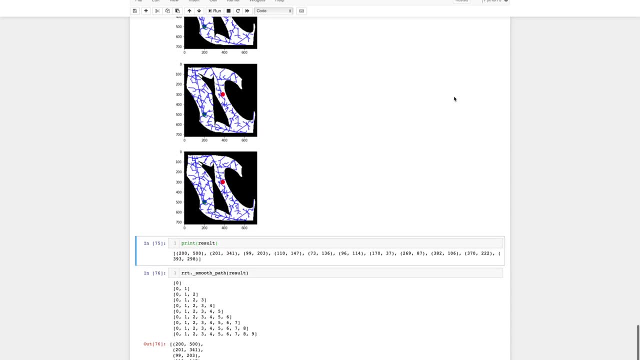 So let's go back to the top. Come on, Let's find a path, Not quite Not getting very lucky. here are we, There we go. I mean, luckily for us, the path's pretty smooth already. I think we can maybe smooth out one or two vertices. 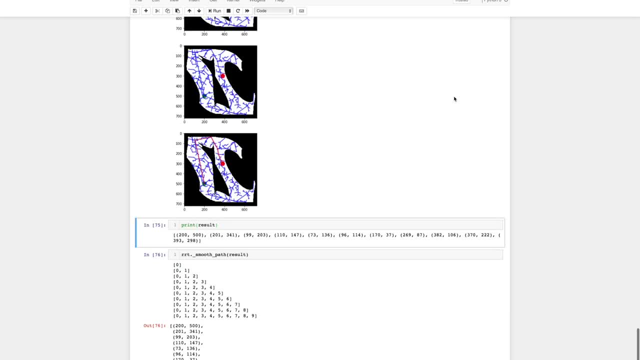 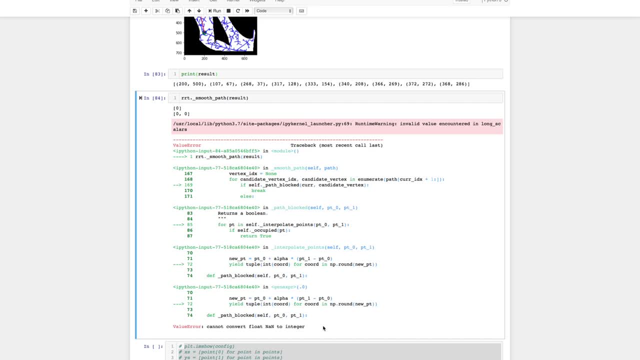 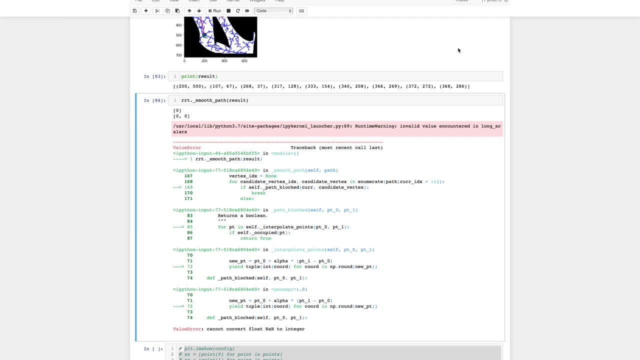 I've got this. I've got this. I've got this. So this is not looking good so far either. Alright, What's going on? Alright, I'm going to stop this for now, figure out the problem offline and then come back. 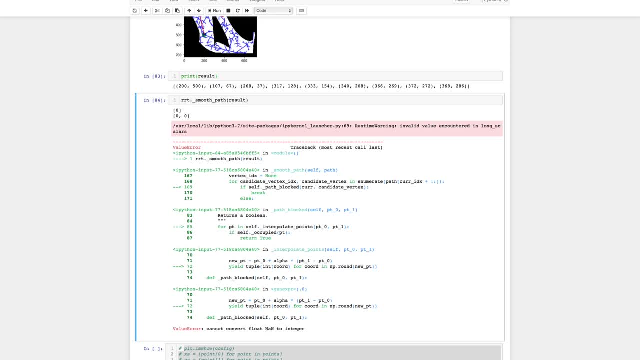 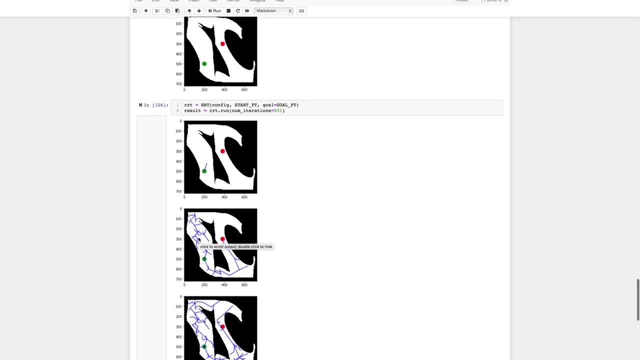 Alright, I'm back, Figure out what the problem was. So let's go in here. I've got a couple of vertices here too. Alright, I'll take a look. So there we go. So what I was doing. 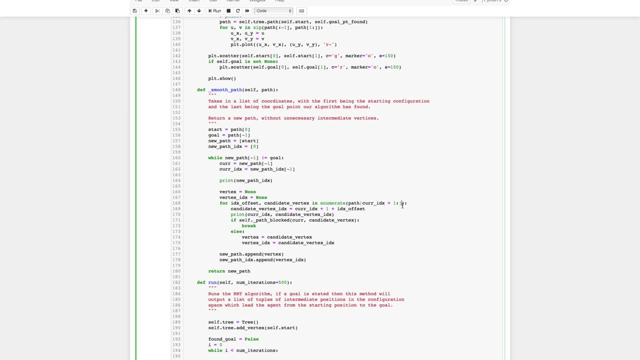 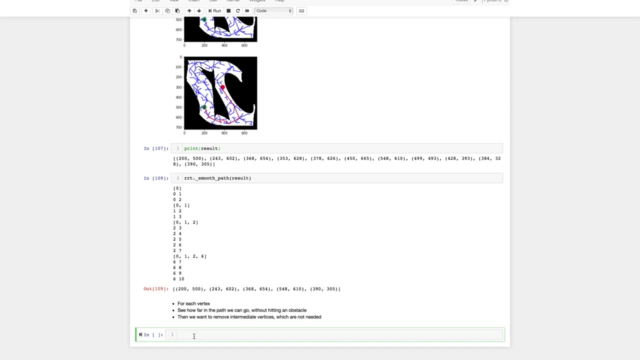 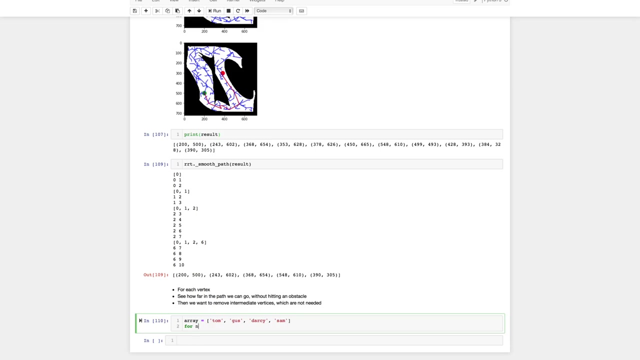 this enumerate was. so the way enumerate works is: if you've got- I'll just do a quick example- if you've got an array- Tom, Gus, Darcy and Sam- if you want to iterate over the elements for name and array, you can print out the name, right? 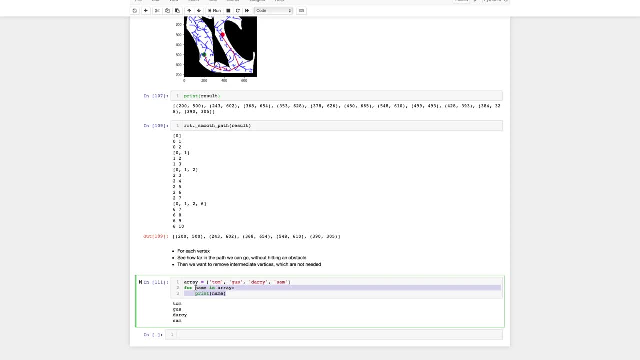 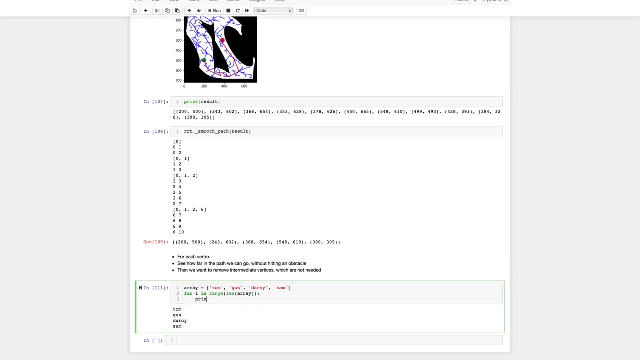 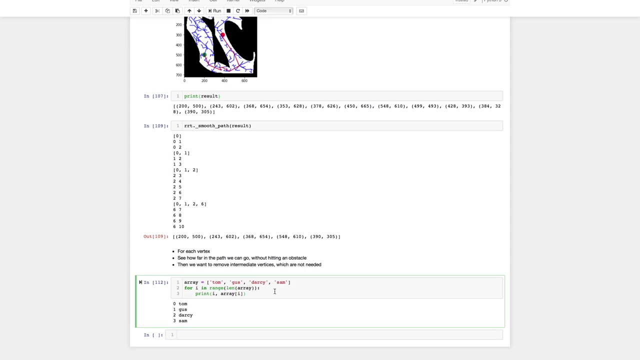 but how do you actually get the indices? well, another thing you can do is you can say for i in range len array, you can print out the index and the element, but that's kind of clunky. then we have to keep accessing this, we have to keep indexing our list. 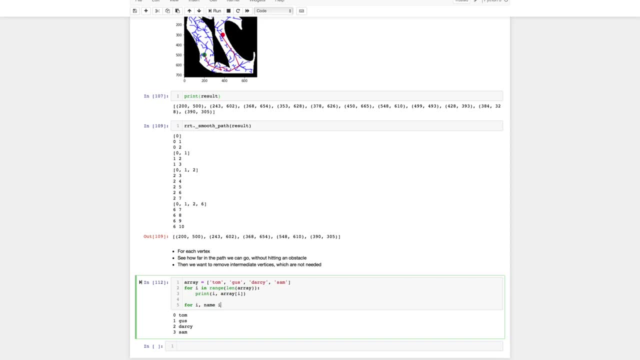 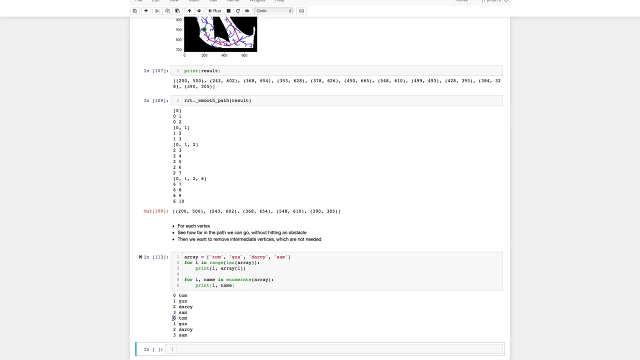 so one thing you can do is you can say for both, so for i in range and name in enumerate and give it our list. you can just say print i and the name, so it's going to do the same thing. so it just gives us the index. 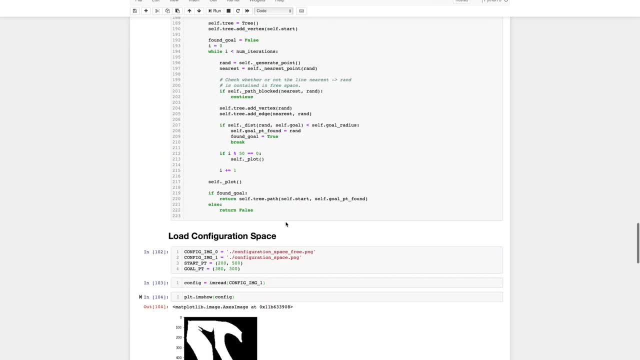 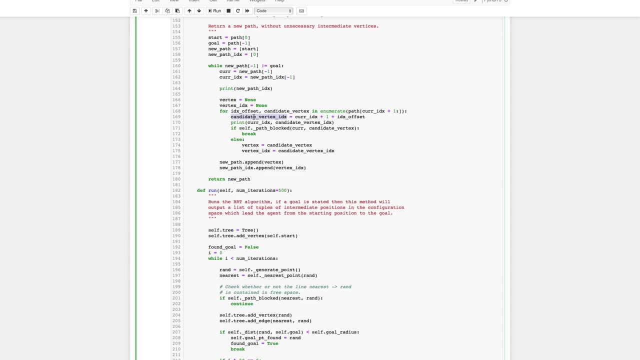 and the element my issue was when I was calling this. I didn't have. I was using the index it gave as the index to the vertex. however, of course I also have to include that that's some offset past the current index we're at, so that didn't quite work out. 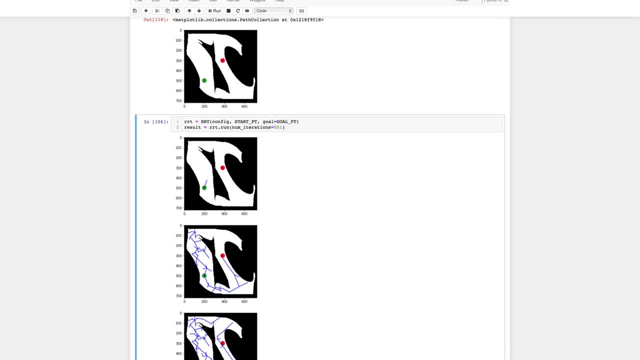 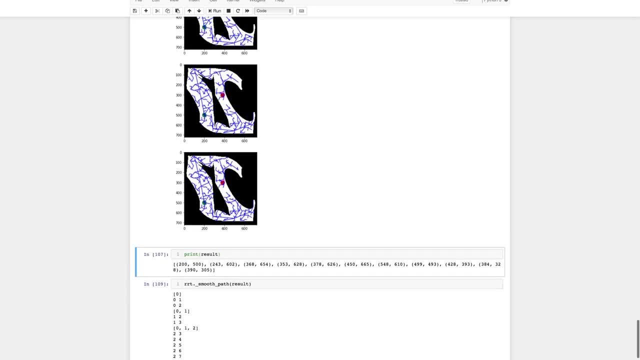 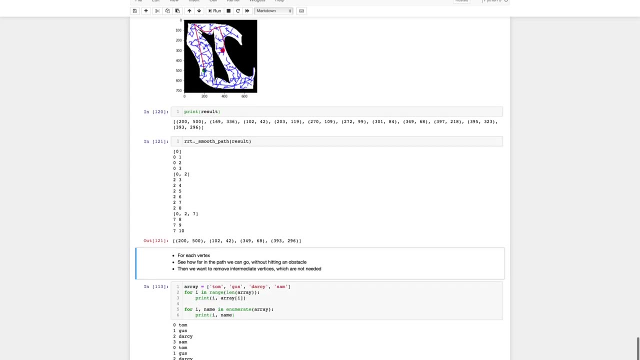 but it works. now let's have a look, let's run our algorithm. cool, so we've found a path. we can smooth out that path and we see that we get significantly fewer vertices. one, two, three, four. I anticipate it goes like this: 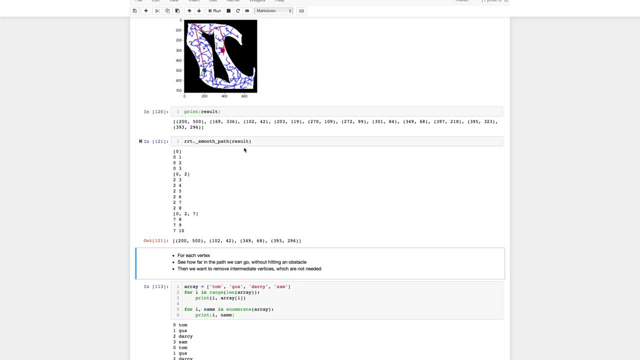 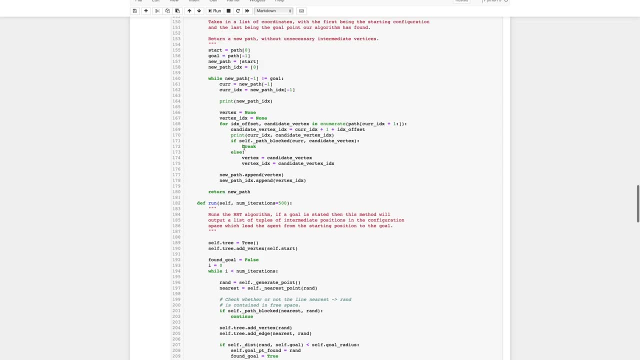 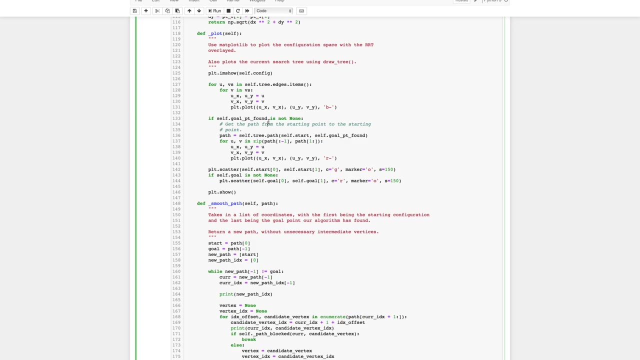 there and down to our solution. so let's incorporate that when we're plotting our path. so what we'll do is, once the self-call is found, we check that path, we find some path and we plot that. let's just smooth that path out. so path equals self-smooth-path. 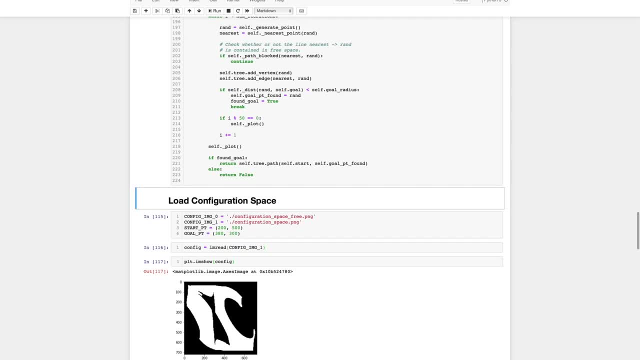 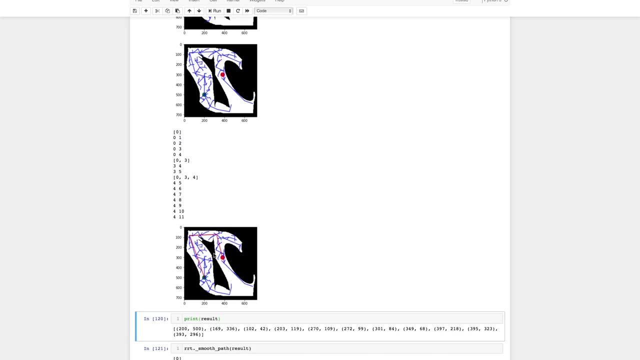 give it the old path and then we run our algorithm once we find a path. you see, it'll actually smooth that out. for us looks good, alright. so that's all that I'll cover for the demo. I'll make this code available so you guys can play around with it yourself. 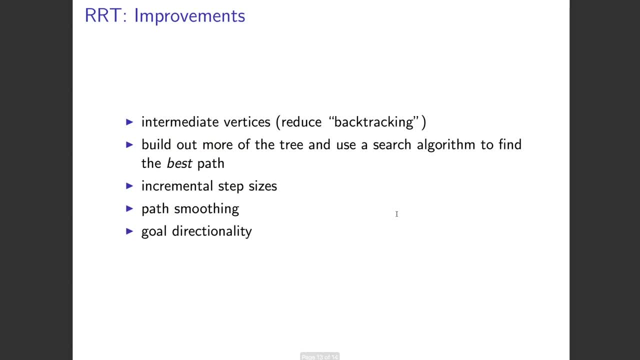 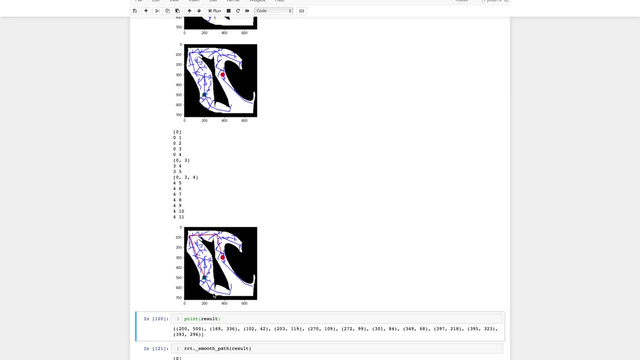 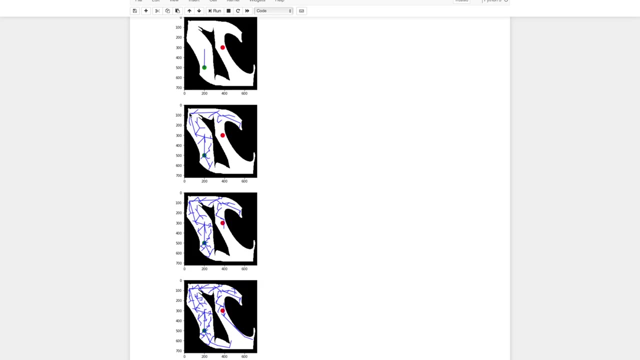 I want to quickly talk about some of the things we could do to improve such an algorithm. I mean, when we were over here. you can see that. where's a good example of this? to get from this point to this point, we went all the way there. 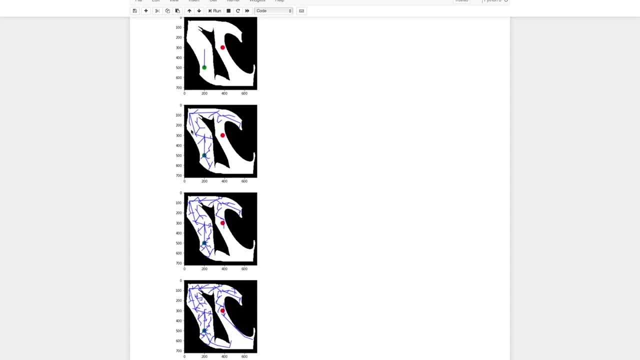 and then kind of came back: if you were actually implementing this as a motion problem, you would just want to go from here straight there. so we can use a similar thing that we were doing with the smoothing, or we can model intermediate vertices along these paths. so then when we get the closest point in the tree, 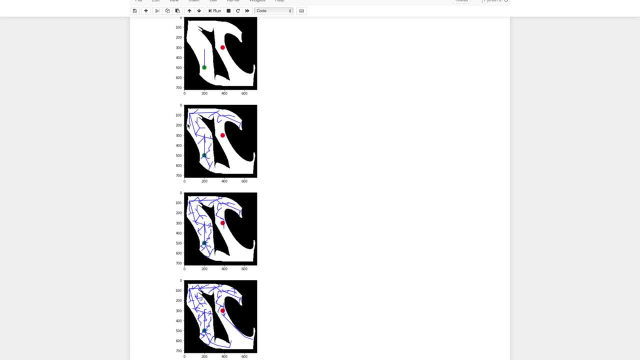 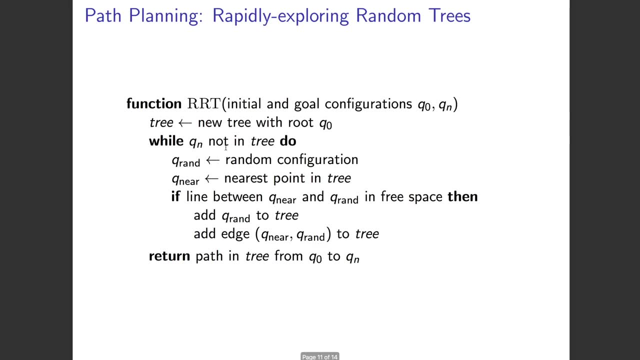 it'll actually end up almost perpendicular to this line. so rather than joining up and going there and all the way back, we would go there, but then the next point would just come straight off this, and you can see that's what's happening here. almost all of the edges are perpendicular to the previous one. 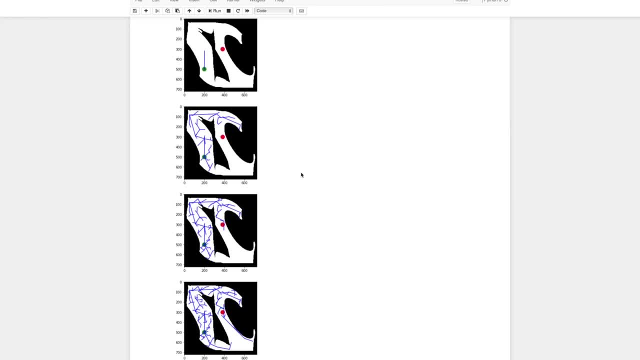 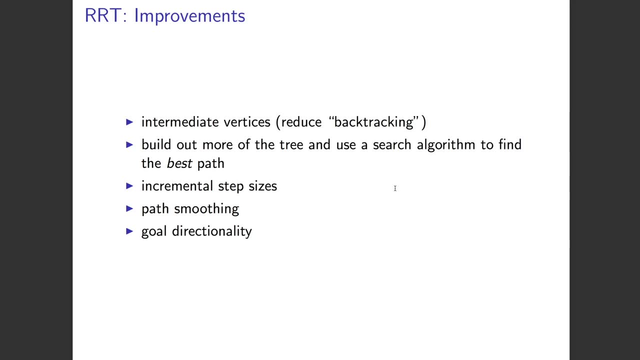 alright. another thing we could do: we're stopping when we get to the solution. so we get to this point and then we stop our search. what we could do is we could build out the tree for more iterations and then we might get multiple paths from the start to our goal. 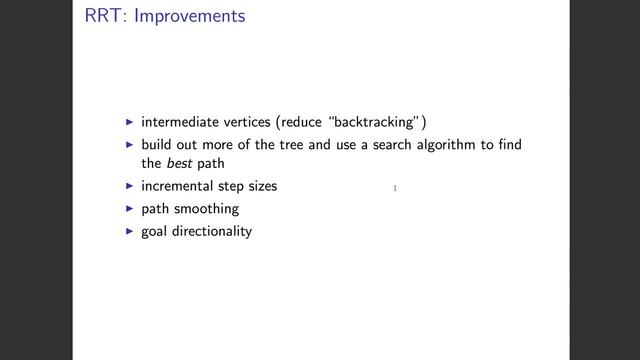 and then we can use some other search algorithm. we've got to find the best path, so I guess that depends on what our definition of the best path is, but it's certainly not the case that this RRT algorithm is always going to find the optimal path. 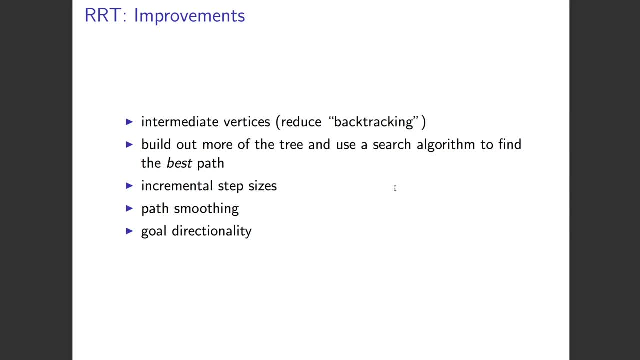 first time round. the other thing is we could use incremental step sizes, so rather than going from one point to the random point and drawing a line between them, we could just say, alright, well, let's only go 10 pixels at a time, just to keep this kind of tree growing uniformly. 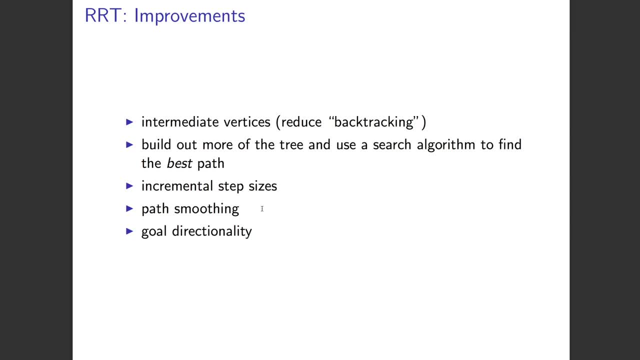 path smoothing we talked about. there's a few other things you could do with path smoothing, I guess, and one of the other things that has resulted in major speedups in this algorithm is goal directionality. so when we were choosing random points, we were just choosing random points uniformly from around the configuration space. 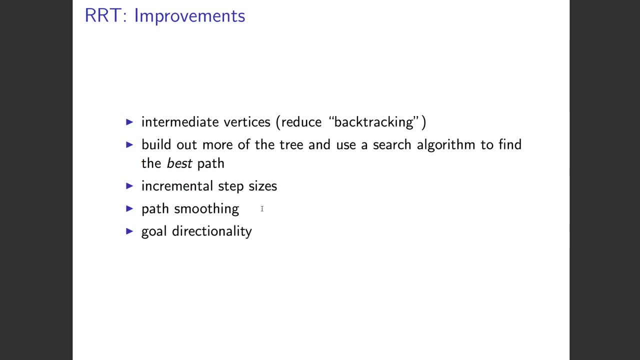 one of the things we could do is we could tweak the probabilities so that we're much more likely to choose random points in the direction of the goal, and that'll kind of encourage our algorithm to build out the tree from our starting point towards the goal rather than just uniformly in every direction. 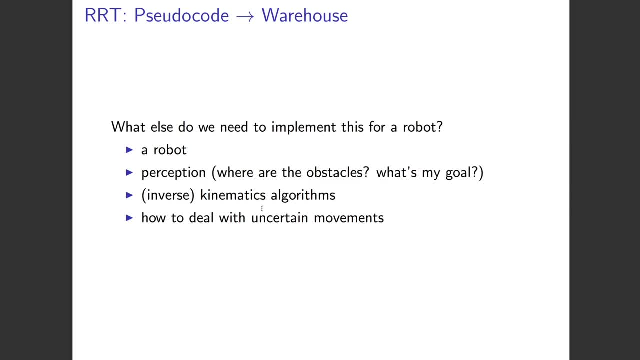 alright, so we've got this algorithm. it's a great algorithm, um- and what we've done is we've solved this motion planning problem in the sense that we've taken one configuration and we've got to another configuration. but how do we actually implement this if we've got 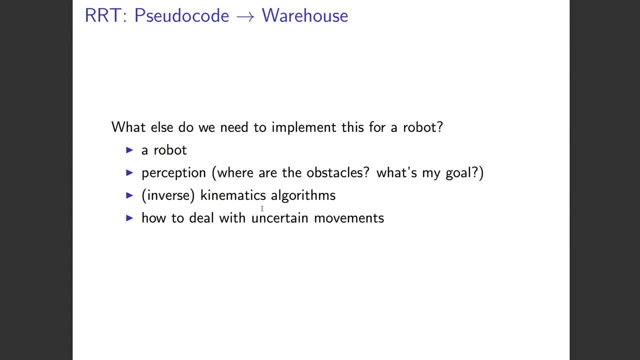 not just this problem, but we actually want a robot in a warehouse that works like this. so one of the things we need, obviously, is the robot and all the mechanical and electrical engineering that goes along with that, all of the joints, all of that, um, all of the controls that go into that. 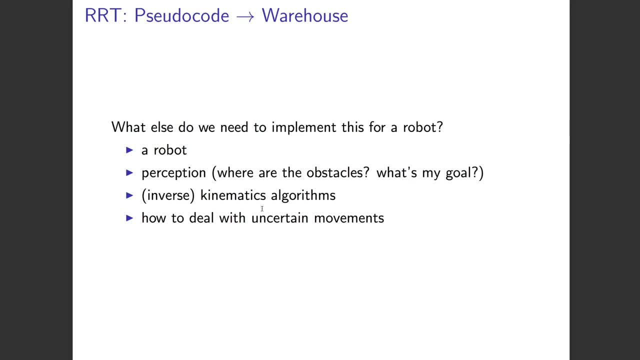 um, but from an AI point of view, we're going to have this perception problem. we need to know, we need to be able to detect where our obstacles are and then convert that into some representation in the configuration space. we also need to determine what my goal is.